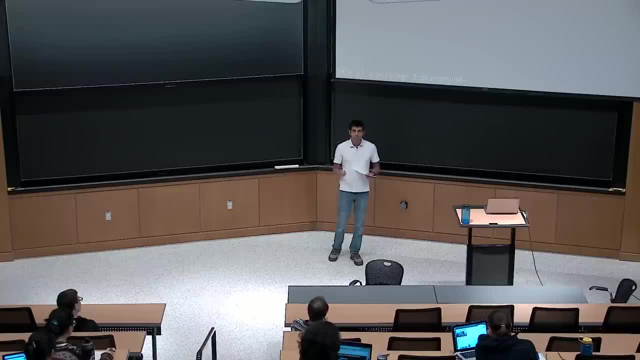 contained within Sumtopl, And then version control systems also maintain a bunch of metadata along with the actual changes to the content, And this is to make it possible to figure things out, like who authored a particular change to a particular file or when was a particular change made, And so version control systems maintain. 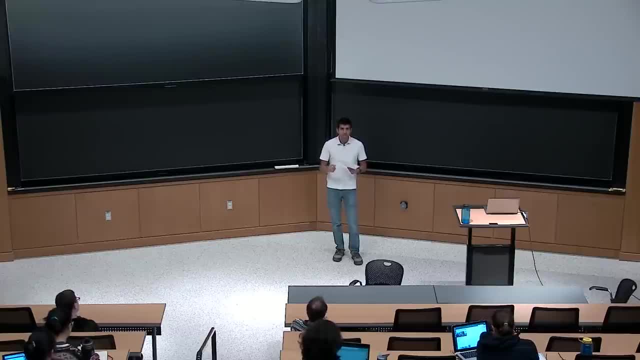 metadata like authors and commit timestamps, And you can also attach extra messages to these snapshots and things like that. And so why is version control useful? Well, it's useful even when you're working on projects by yourself. You can use it to look at old versions of code you've written, figure out like why something was. 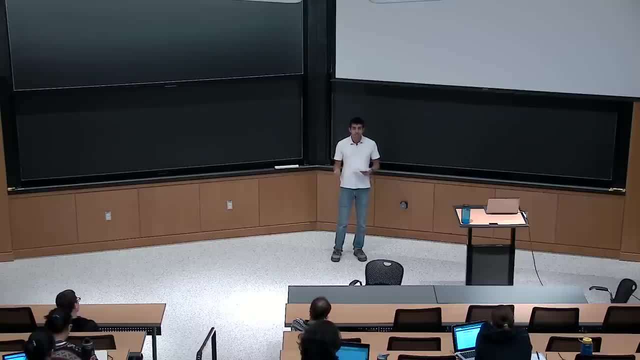 changed by looking at commit messages, work on different things in parallel without conflicts, by using different branches of development, or be able to work on bug fixes while keeping work on different features independent things like that- And so it's an invaluable tool, even if you're. 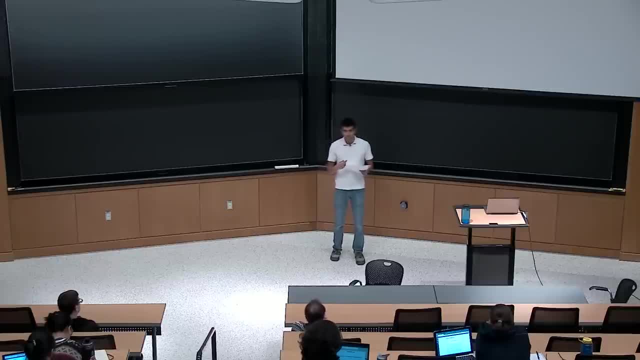 working just by yourself, even on a small scale project, Like, I think, the instructors of this course use Git even on things like homework assignments or class projects, even small scale Things in addition to our research or larger software projects, And then, of course, version control. 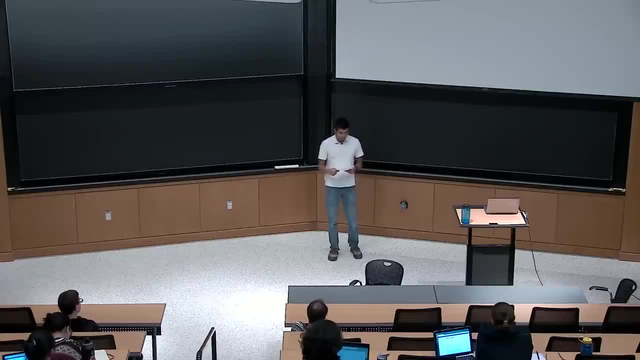 is a really powerful tool for working with other people, So it's useful for sending patches of code around, resolving conflicts when different people are working on the same piece of code at the same time- things like that- And so it's a really powerful tool for working by yourself or with others. 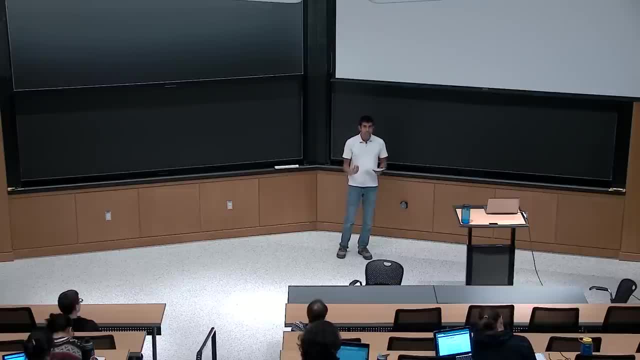 And it also has neat functionality to let you answer questions that would otherwise be kind of hard to answer, Like who wrote a particular module in a software project Or who edited a particular line in a particular software project? Why was this particular line changed? When was it changed, By whom? Things like that And version. 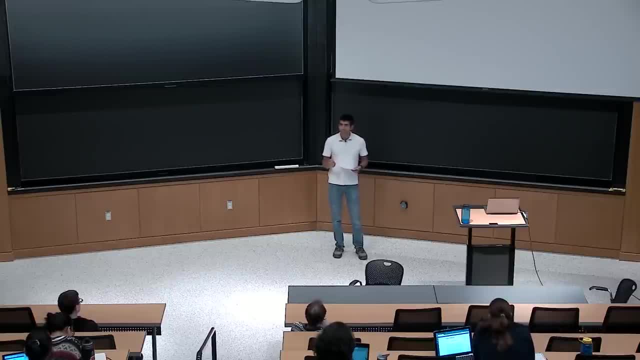 control systems also have some really powerful functionality that we might cover at the end of today's lecture or you can find in the lecture notes if we don't have time. to do things like: suppose you have some project you've been working on for a couple years and then you notice that 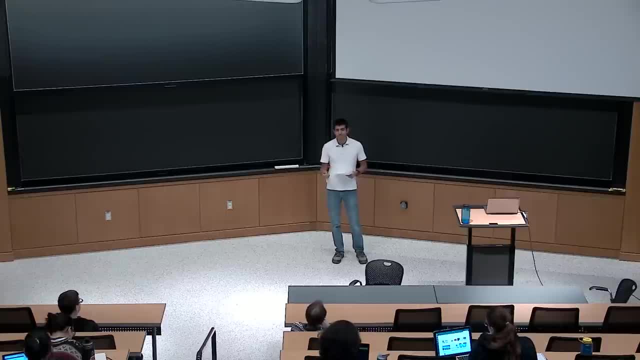 some funny thing about the project is broken. Like you have some unit test that doesn't pass anymore, And it wasn't broken just now, it was broken some time ago and you don't know exactly when this regression was introduced. Well, version control systems have a way of. 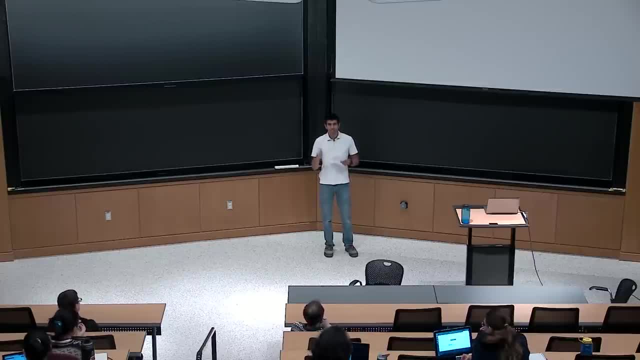 automatically identifying this. Like you can take Git and give it a unit test that's currently failing, but you know it's passing at some point in the past- and it can binary search your history and figure out exactly what changed your code made it break. So lots of really powerful fancy. 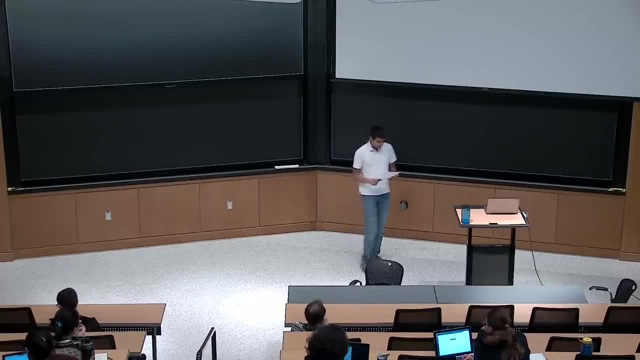 features if you know how to use these tools properly. There are a number of version control systems out there that are really powerful, and Git has become kind of the de facto standard for version control, So that's what we're going to be covering in today's lecture. 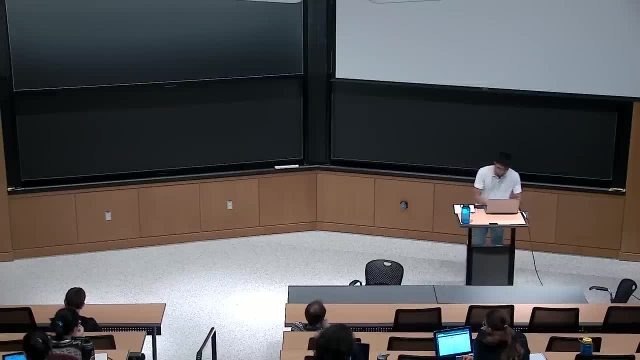 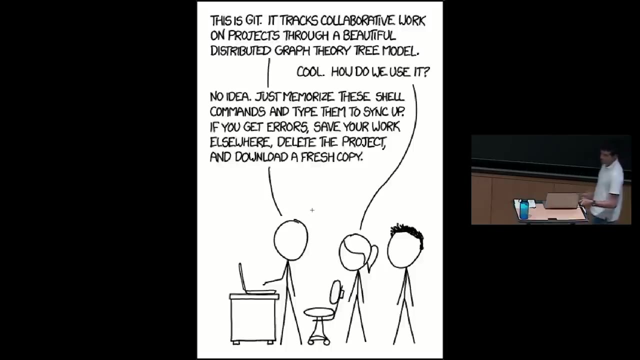 One comic I want to show you, which was on the screen beforehand. Let me bring it back up. So this is an XKCD comic that illustrates Git's reputation. So let me read it out loud for you. This is Git. It tries collaborative work on projects through a beautiful distributed graph theory tree model. 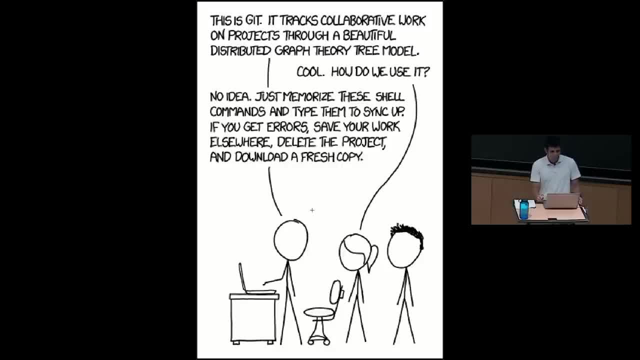 Cool. How do we use it? No idea. Just memorize these shell commands and type them to sync up. If you get errors, save your work elsewhere, delete the project and download a fresh copy. So maybe some people may not want to raise their hands for this. 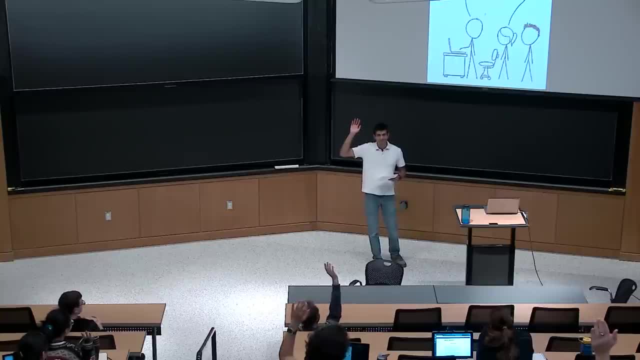 but raise your hand. if you've ever done this before, I certainly have when I was learning this tool, So a good number of you here have done this before, So the goal of this lecture is to make it so you don't have to do this anymore. Unfortunately, as this 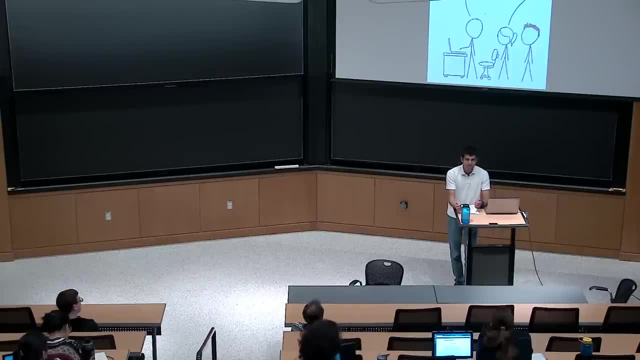 comic illustrates, Git's interface is a pretty terribly designed interface. It's a leaky abstraction, And so, for this reason, we believe that learning Git top down, starting with the interface, is maybe not the best way to go, And it can lead to some confusion. 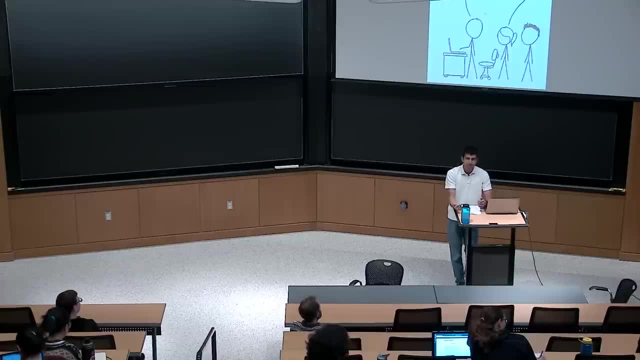 It's possible, like this comic shows, to memorize a handful of commands and think of them as magic incantations, And when everything's working all right, it kind of works out all right, But then you have to follow the approach of this comic whenever things go wrong. 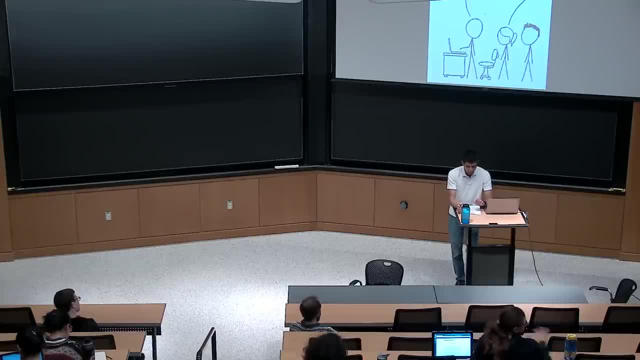 So while Git has an ugly interface, its underlying design and ideas are actually pretty beautiful. An ugly interface has to be memorized, but the beautiful ideas underlying Git can actually be understood. And once you understand Git's internals, its data model, which is actually not that complicated- then you can learn. 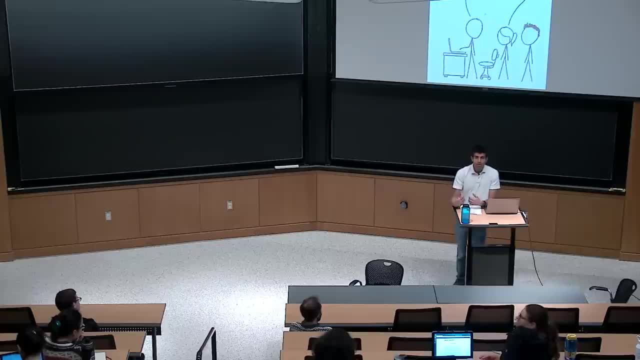 the interface to Git. You'll have to memorize some things, but you can understand what exactly certain commands do by understanding how they manipulate the underlying data model, And so the way we're going to teach Git today is first talk about the data model almost in abstract. 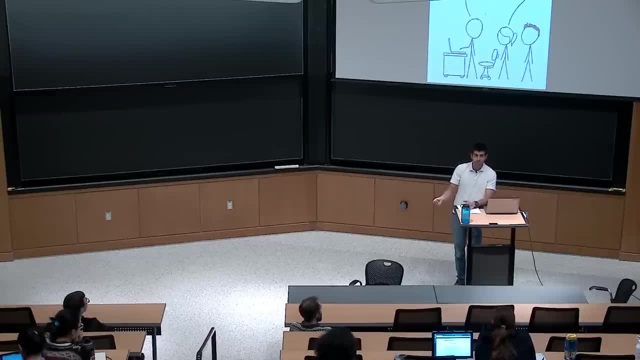 talk about how we might model files and folders, snapshots of history and how they relate to each other, And then, after that, we'll walk you through some Git commands And then, finally, in the resources and exercises, we'll link you to tutorials that'll teach you all the specifics, because there are lots of different commands. 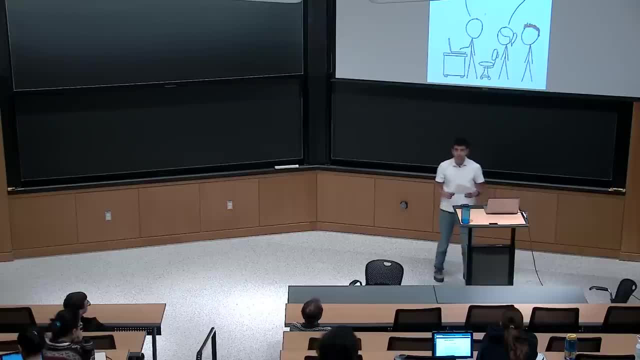 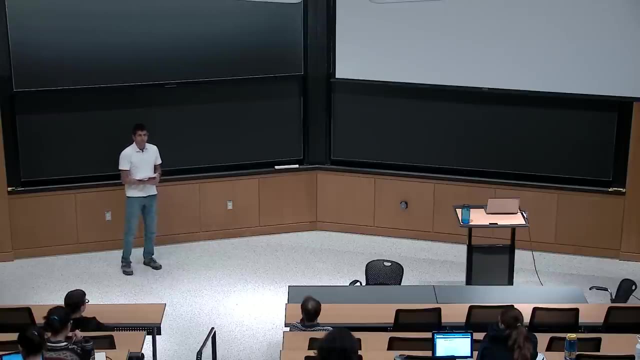 that you will need to learn eventually. Any questions so far about our teaching approach for today? Cool, Great, So let's get started. There are probably many ad hoc approaches you could take to version control And I'm guessing some of you may have done this before, Like, say, you have some file or folder. 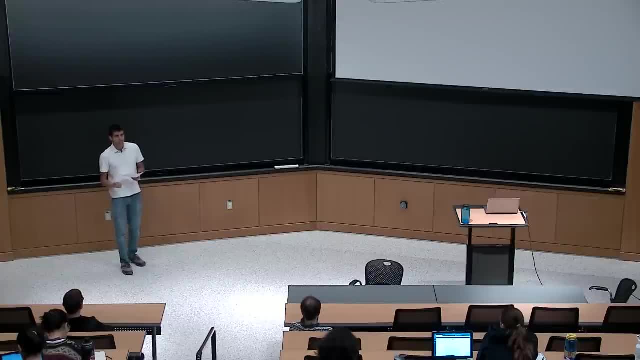 where you have a bunch of different files corresponding to some software project and you want to track changes, You could just say: every day make a copy of that entire folder and give that folder a timestamp. When you want to do things like collaborate with other people, you could take the entire folder, turn it into a zip archive and email it to. 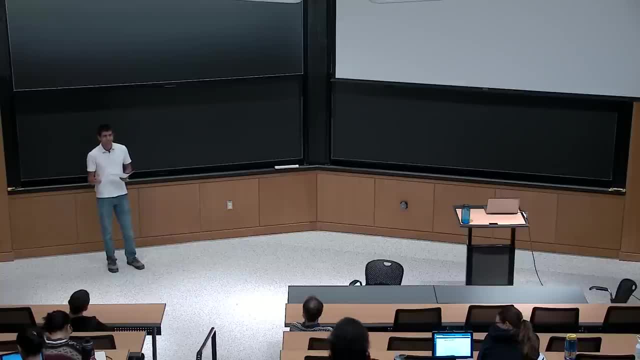 somebody, And then whenever you and your buddy are working on two different features of a software project, you can work on them in parallel- Then one of you emails the zip file to the other person and then you manually copy and paste the appropriate segments from their code into your code so that eventually you end up with one piece. 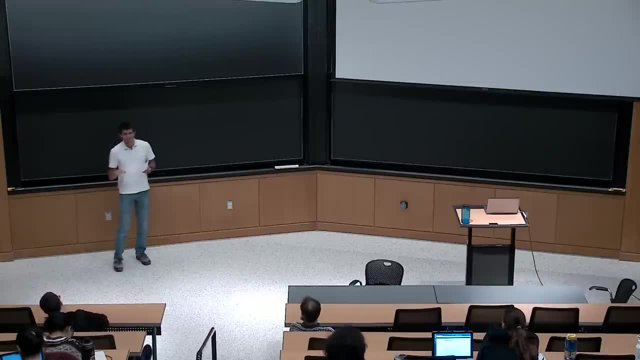 of code that has both of your features in it. This kind of sort of works. Raise your hand. if you've done this before, I certainly have Still a decent number of you. Git lets us not do this sort of thing. It has a well thought out model that kind of facilitates these sorts of interactions. Things that you might want to do, like tracking your own history on your own project or collaboration or things like that. Git has a well thought out model that enables things like branches and collaboration and merging, changes from other people- All sorts of neat stuff. 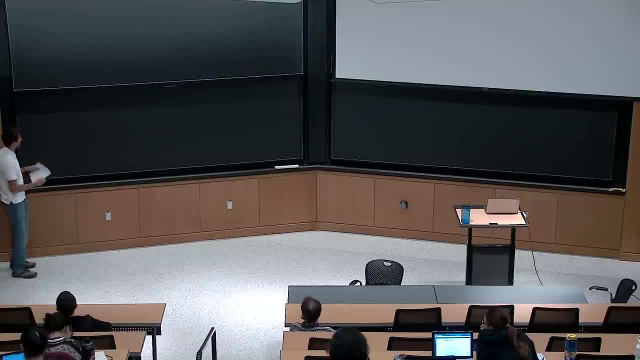 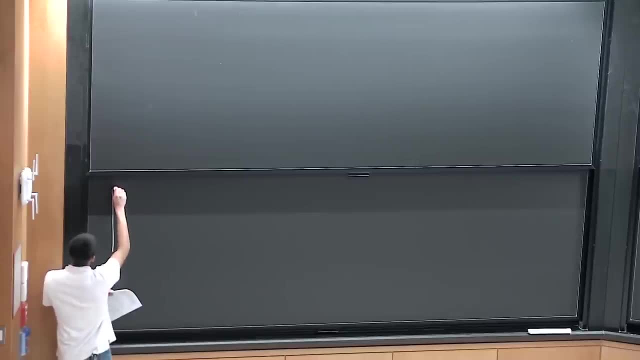 Git models history as a collection of files and folders within some top level directory. You're probably familiar with this abstraction just from files and folders on your own computer. Here's one example. You might have some top level directory- I'll just call this root and parentheses. 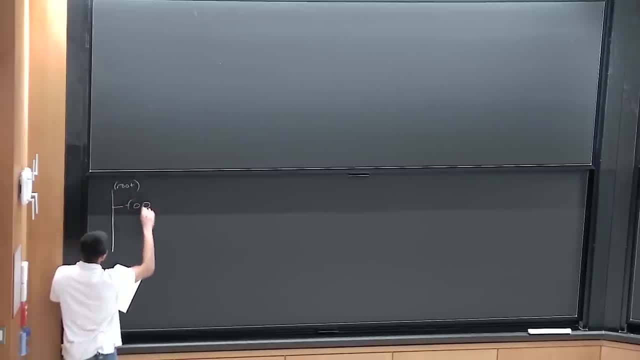 And this directory might have, say, a folder in it called foo, And this folder inside of it might have a file called bartext And this might have some content in it like, say, this says hello world. And then maybe this top level directory- it has one folder in it- It could also have another file in it. 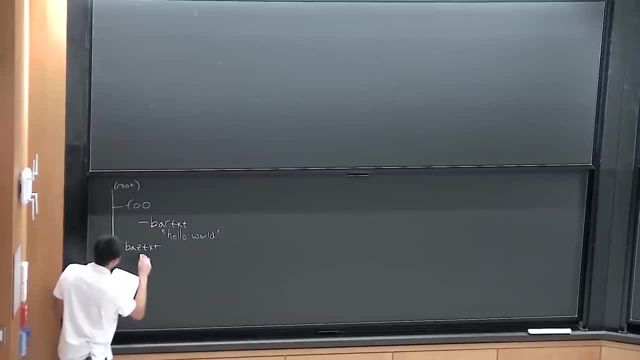 So say, there's some other file And this file also has some content in it. All right, Simple enough. The terminology Git uses for these different things for files and folders is this, and the top level thing are called trees. So this is a folder, And then these things. 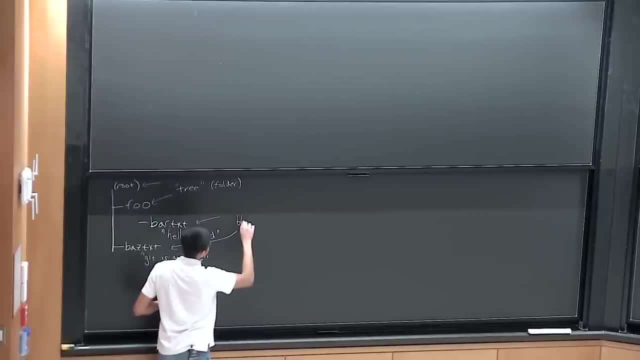 what we normally call files are called blobs. All right, OK. So now we have a model of files and folders, And this is a recursive data structure. Trees can contain other trees, And then trees can contain both trees and files. Obviously, files can't contain trees. 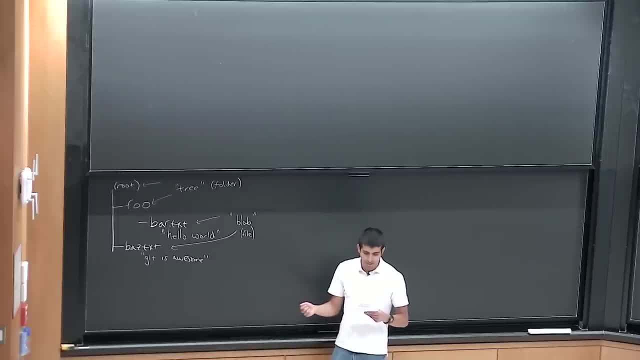 All right. So now we have a model of files and folders And the kind of top level of this thing. the thing I've just labeled root is the directory being tracked. Like you might have some folder on your computer corresponding to a software project. 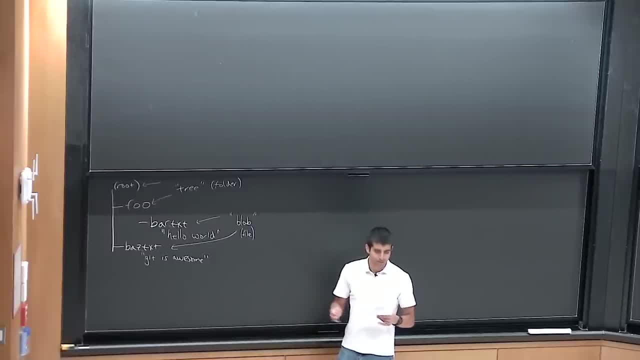 Now, how do you model history once you have a model of files and folders? Well, you can imagine one way of doing it, which is you take a snapshot of this entire thing and then history is just a linear sequence of snapshots, Like you might imagine. that it's, you can almost think of it, like you have copies of the folder. 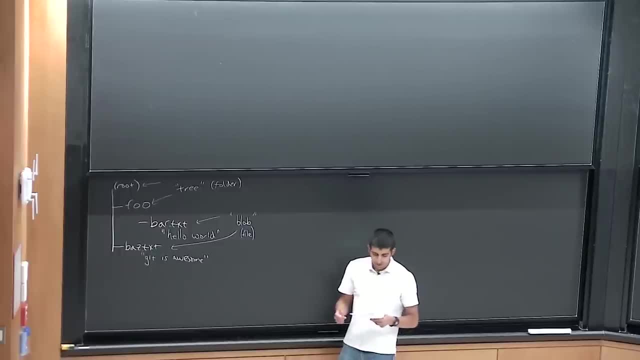 which are dated and timestamped. Well, Git doesn't use a simple linear model like that. It uses something a little bit fancier. You might have heard this terminology before, but Git uses a directed acyclic graph to model history, And this might sound like a bunch of fancy words. 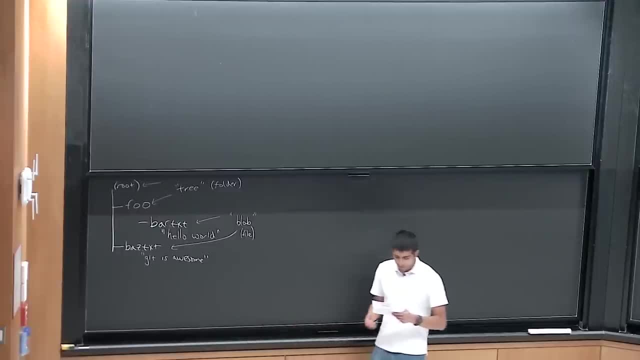 fancy math words, but it's actually not all that complicated. So in Git each snapshot has some number of parents and basically you want to know like what change preceded what other change. So suppose here I'm going to use circles to refer to individual snapshots. 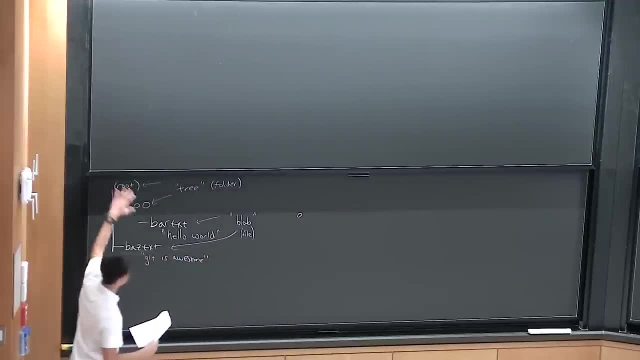 This is the entire contents within this tree, So all the files and folders in my project, My entire project, may be in some state, and then I edit some files and now it's in some other state. And then I edit some more files and now it's in some other state. 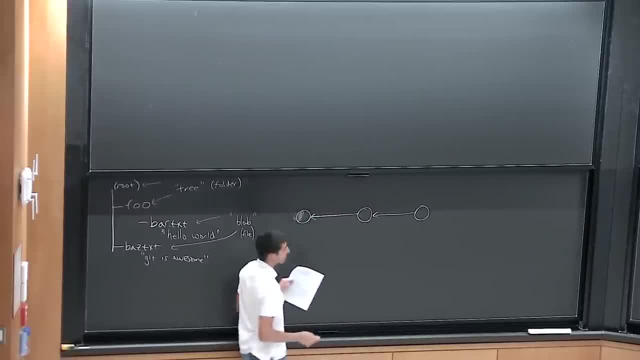 And every state points back to which state preceded it. This, so far, is a linear history. but, Git, lets us do something a little bit fancier than this. You can also, from a certain snapshot, fork your history and say: I want to base changes off of this version. 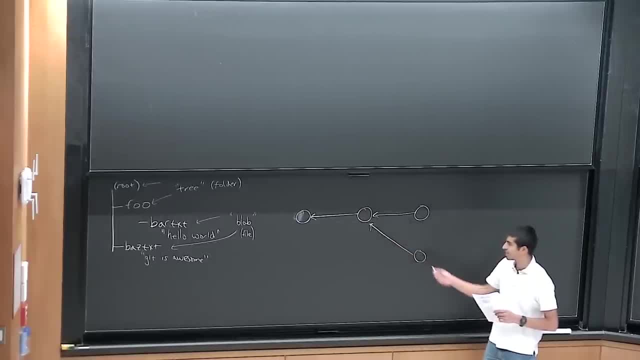 and create a new snapshot like this. So this way of modeling history allows you to do things like: okay, I'm working on my project, This is my main line of development. I go up to here and now I have two different tasks I want to work on. 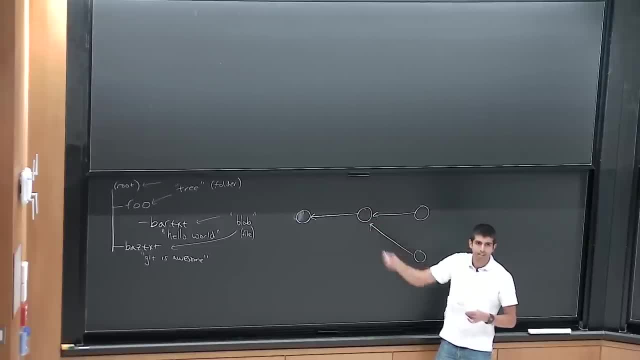 Suppose, on one hand I have some fancy new feature I want to add to my project and so I'm going to be working on that for a couple of days. But separately from that, somebody's reported a bug to me and I need to go chase down that bug and fix it. 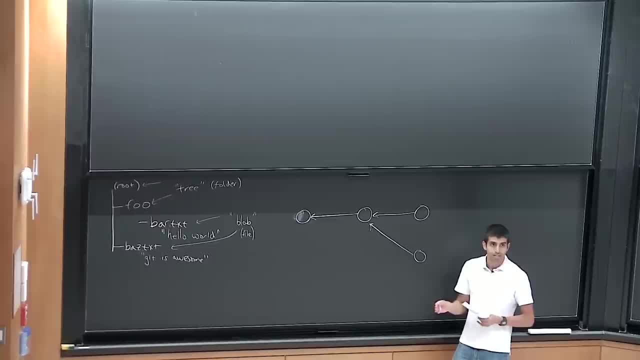 Well, instead of working on all that stuff kind of concurrently at the same time in the same line of development, Git has this way of branching the history into two separate forks and working on different things in parallel temporarily, in a way that are unrelated to each other. 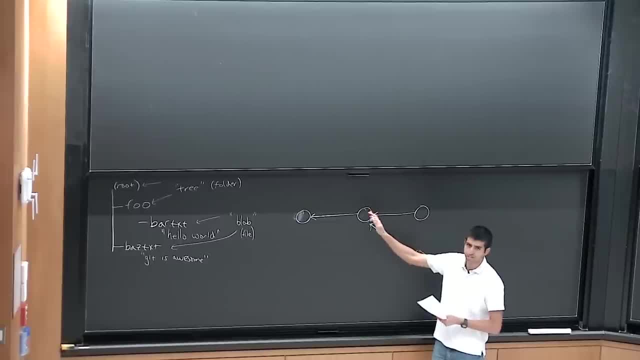 So I could take this base snapshot, like my project is in some state where it works, and then from here I could implement a new feature that creates a new snapshot. So this has the base project plus a new feature. So I'll do like plus feature. 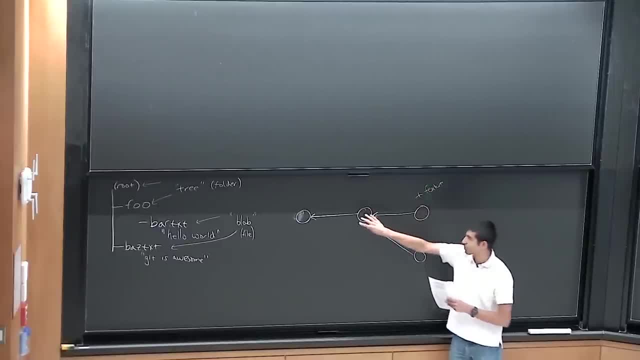 And then, similarly, separately from this, I could go back to this original snapshot, because I don't want to do bug fixing while implementing my new feature, Go here and then work on my bug fix and create a different snapshot. So this has only the bug fix. 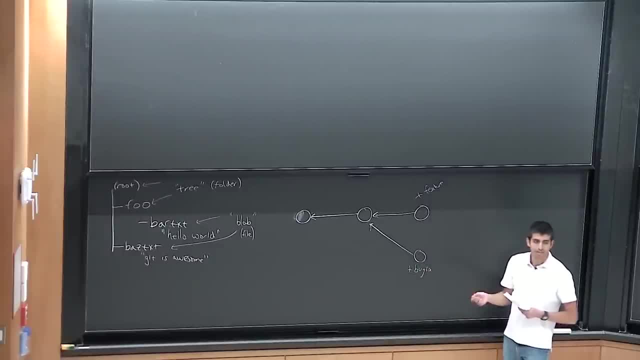 But not the feature. And then finally, once I've done these two separate things in parallel, eventually I want to incorporate them all into my common source code that has both the feature and the bug fix. So eventually I might author a new snapshot by merging the changes present in these two different snapshots. 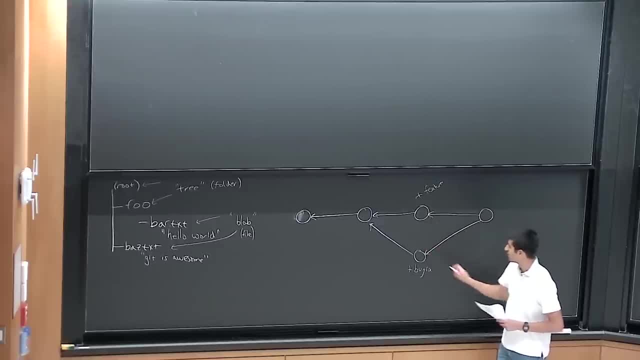 And so this one will have both of these snapshots as parents, And this version here will have both the feature and my bug fix. So does it make sense why Git model's history in a way that's a little bit fancier than just a sequence of snapshots of my files and folders? 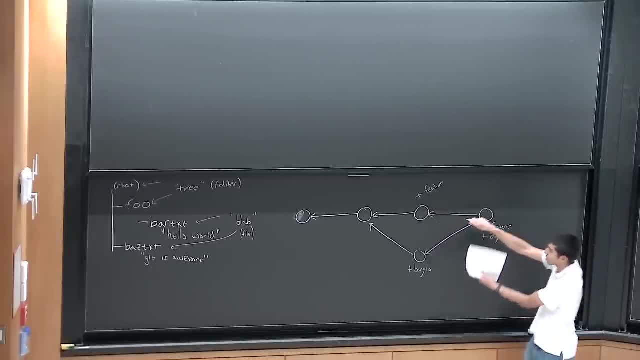 why I want to be able to support branching, to work on things in parallel, and then also merging to combine changes from different parallel branches of development. Question: When you merge things, it seems like you can create errors that weren't anticipated. Yeah, So that's an excellent point. 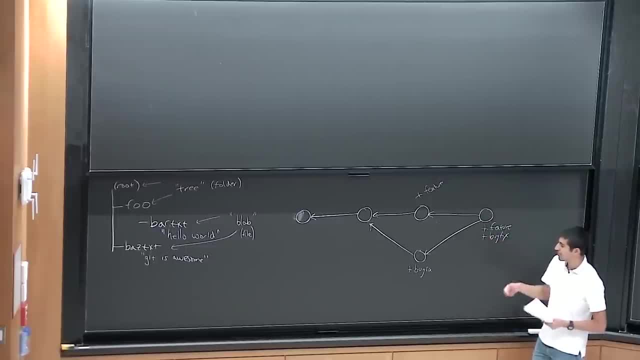 It seems that when you merge things, you could create errors that weren't anticipated. You could imagine here that this feature actually changes something that makes this bug fix redundant, Or you could imagine this bug fix breaking this feature or something like that. That's a really good point. 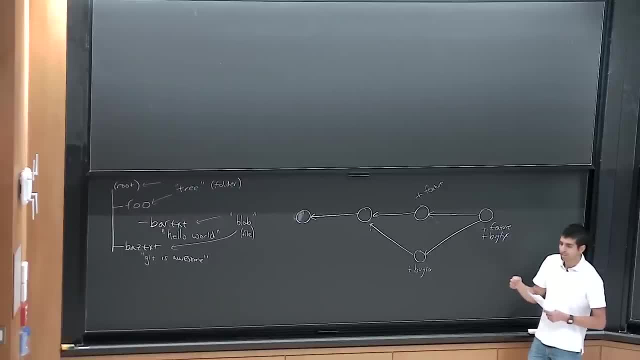 That's something known as merge conflicts, And this is something that Git will try to do. Like when you merge two parallel branches of development, it will try to automatically combine the changes in a way such that it retains all the important changes, But if it gets confused it will report a merge conflict. 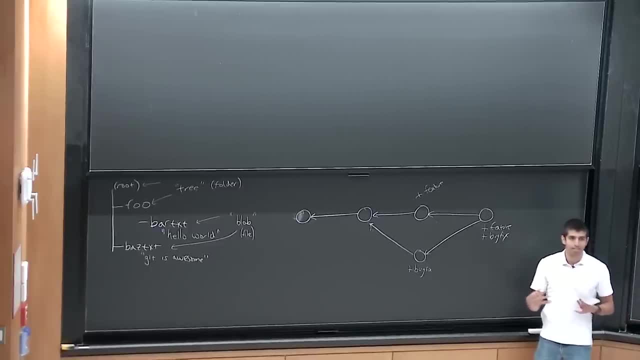 and then leave it up to you, the programmer, to figure out how to combine kind of concurrent changes to the same files or things like that. And then Git has some tools for facilitating this. Any other questions? Great, Okay, so now we have a model of files and folders. 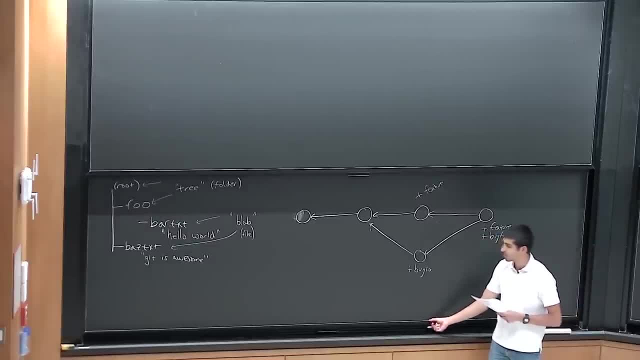 and then we have a model of history how different snapshots of our code relate to each other. One little detail here is that each of these circles, so they kind of correspond to a snapshot, like a tree with files and folders, but they also have a little bit of metadata. 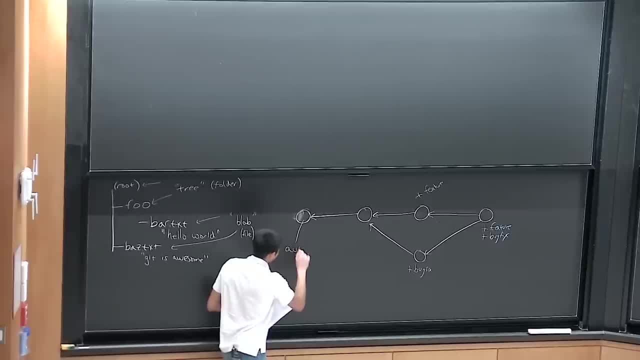 So, like inside here, we might have- like the author of this commit is Anish and we might have other metadata, like some message associated with this commit, And I might describe what kinds of changes I've made that are present in this snapshot but not the previous one. 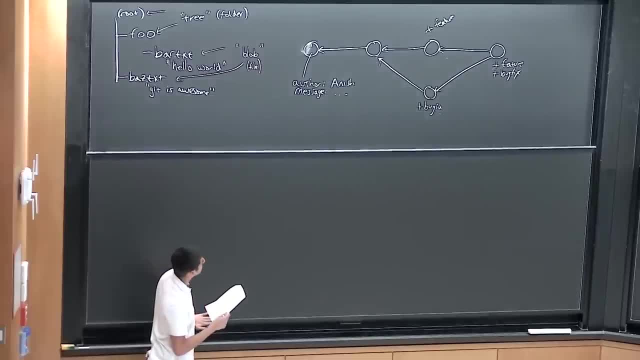 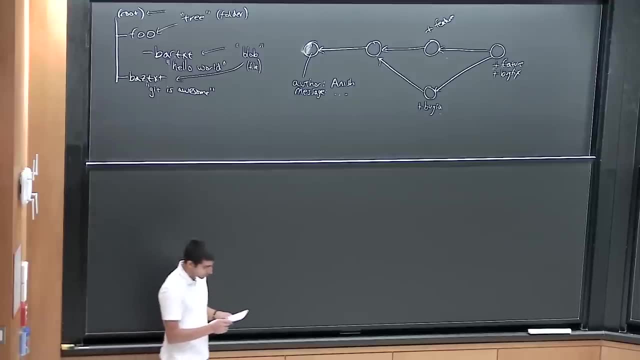 That is not related to our class, So. So next we're going to talk about kind of one level lower than this, Like how exactly is this represented as a data structure inside Git? And so I'm actually going to write down pseudocode. 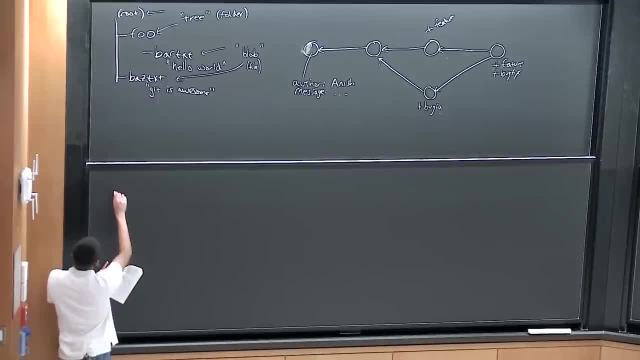 because I think it's actually easiest to understand this way. So first we have files. So a blog is just a bunch of bytes. So I'll say: this is an array of bytes. Okay, then what is a tree? Remember that this is just a folder. 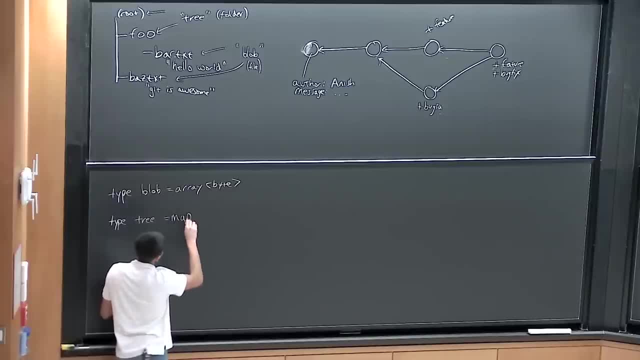 What are folders? They're mappings from the file name or directory name to the actual contents, and the contents are either another tree, like a subtree, or the file. So, And then finally, we have the last thing there, what I've been calling snapshots so far. 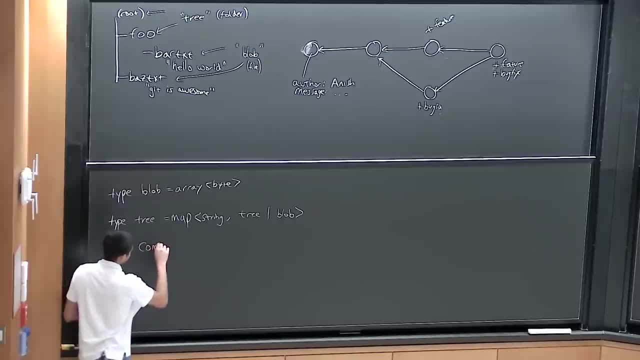 In Git terminology those are called commits. And so what is a commit? It's a bunch of stuff. Commits have parents that describe what precede them. So in the case of most normal commits they have one parent, like what they came from. 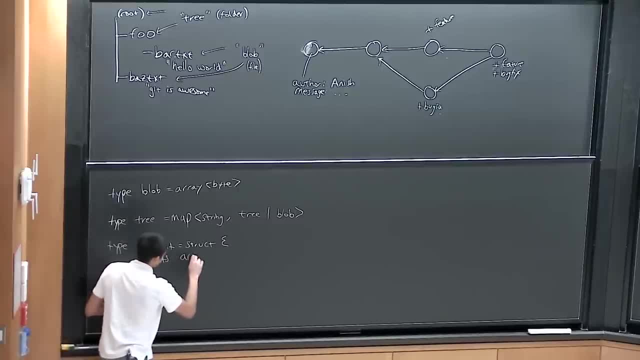 But merge commits can have multiple parents, So Parents are an array of commits. And then I have some metadata, like the author, And maybe a message, And then finally The actual contents, the snapshot, which is a tree, That's the top level tree. 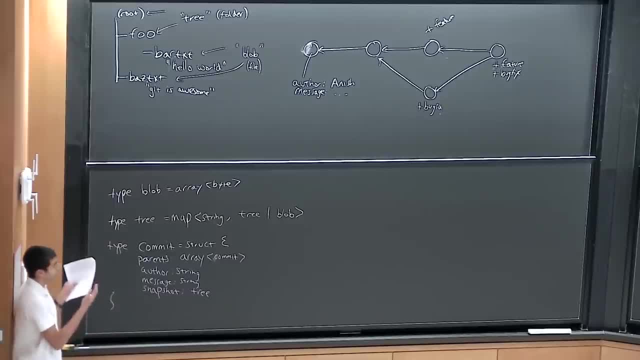 And then the last thing is the corresponding to a particular commit. So this is a really clean, simple model of history And this is basically all there is to how Git models history. Any questions about that? Alright, so now we have that going a little bit deeper. 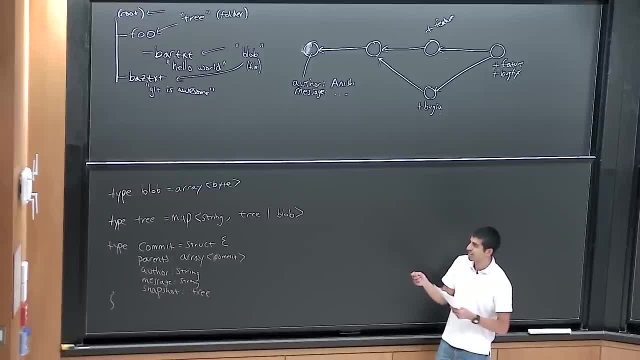 Let's talk about how Git actually stores and addresses this actual data. Like, at some point this actually has to turn to data on disk, right? So you have an object, kind of a big sounding term, But an object is any one of those three things. 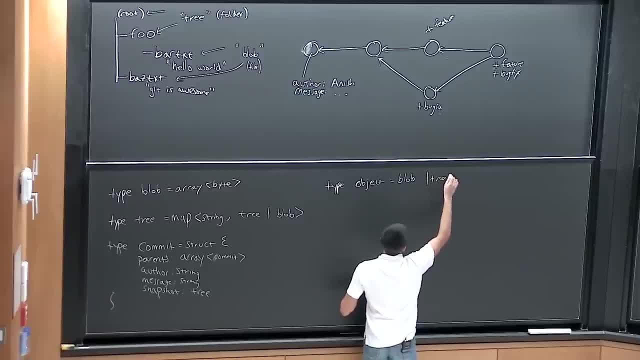 So it's a blob or a tree, a tree or a commit, And then in Git all objects are content addressed. So what Git maintains on disk- and you can actually we can look at this later- is a set of objects. 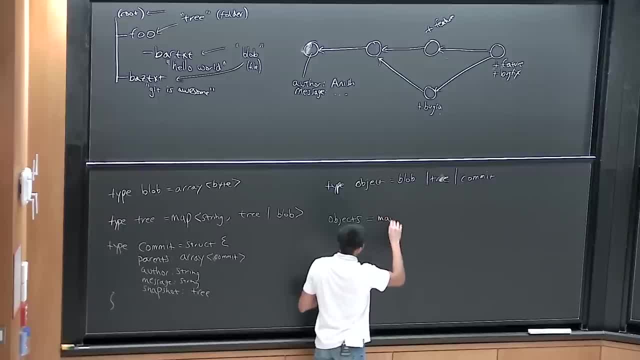 Maintained as this content address store. So if you have any one of these objects, the way you put it into the store is its key is the hash of the object. So, like in pseudocode, I might say that to store a particular object O. 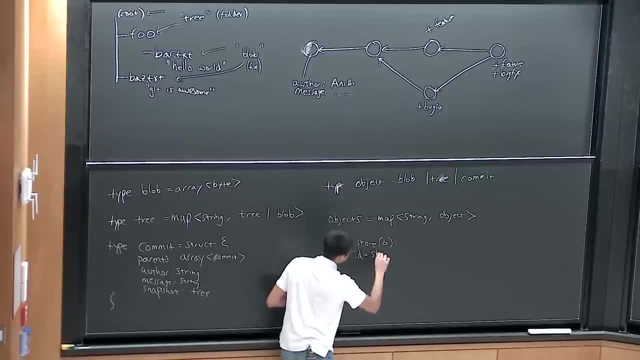 what I do is I compute its ID by taking the SHA1 hash of O and then I put it into my objects map, store it to disk. Quick show of hands. who here knows what a hash function is? All right, so I'll quickly summarize. 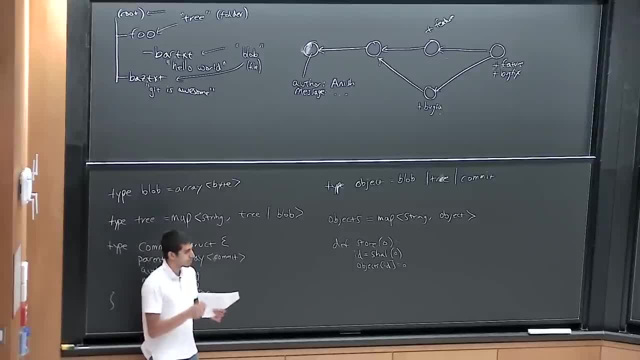 Basically a hash function is. you can think of it as like this magical function that takes a big piece of data and turns it into a short string At a high level. these are used to, or maybe that's like a sufficient explanation. I won't go into too much more detail here. 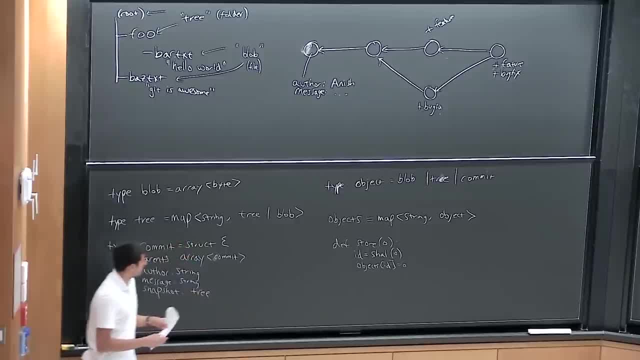 but you can ask me afterwards if you're curious. So basically, they give you a way to name a thing in a way that's kind of deterministic, based on the contents of the thing. It takes in a thing as input and gives you a short name for it. 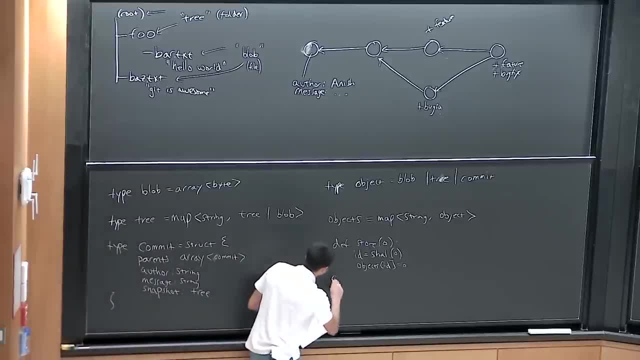 And then the opposite of store is load. The way we can load things from the store, you might have just guessed: you can look them up by their ID and this is just. we retrieve it from the object store by ID and it gives us back the contents. 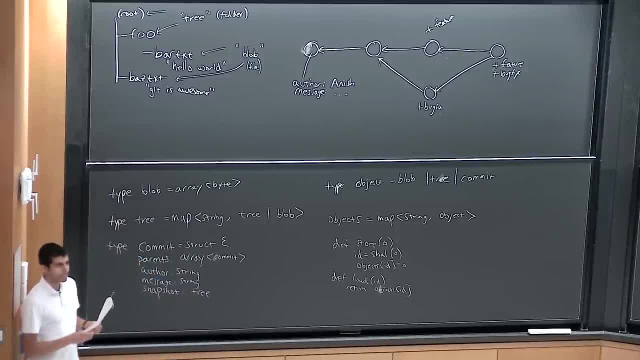 Any questions about this so far? Question: What language is this all written in? That's a good question. What language is this all written in? It's written in a language I just made up, So it's pseudocode, The Git implementation itself: 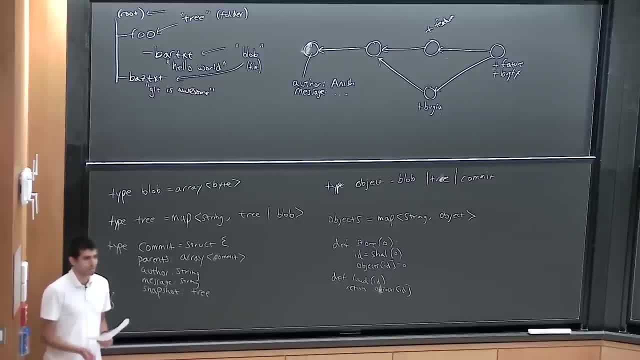 is a mix of C- it's mostly C- and then some Bash and Perl scripts, I think. Any other questions? Is this made-up language clear enough or do I need to explain any aspects of it? Great, Okay, so blobs, trees and commits in Git. 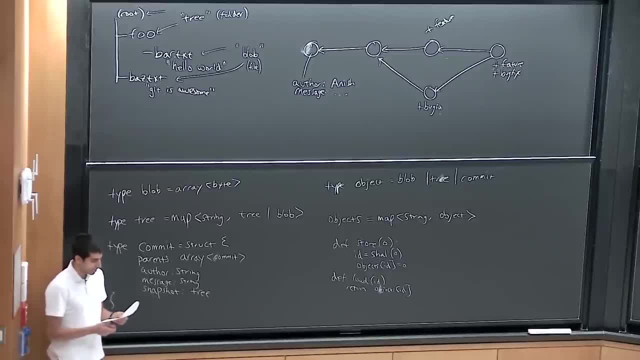 are unified in this way: They're all objects And also, as you might think, given my description here, like it looks like commits contain a whole bunch of other commits and contain a snapshot and things like that. In practice, it doesn't actually work that way. 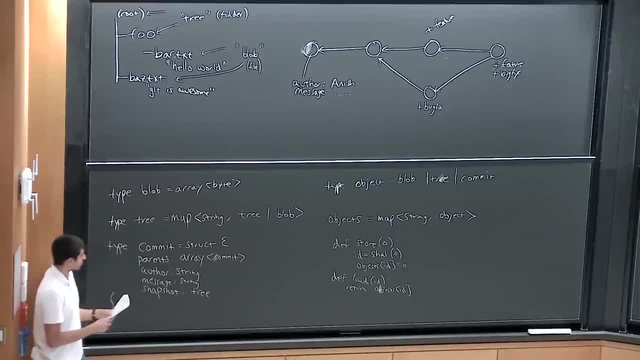 Instead, all of these are pointers, So a commit will be able to reference a bunch of parents by their IDs. So this is actually not an array of commits themselves but IDs. And similarly, the snapshot inside a commit is not the actual tree object. 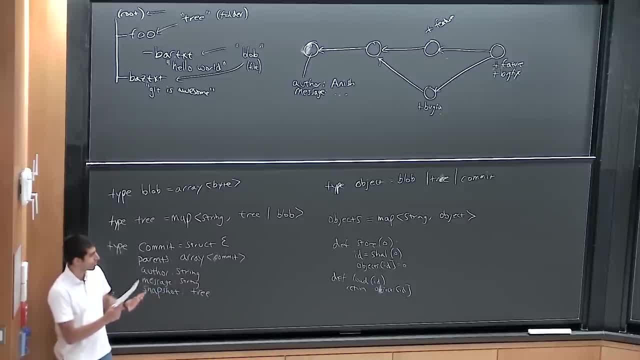 it's the ID of the tree, And so all these objects are kind of stored on their own in this object store and then all the references to different objects are just by their ID, by their SHA-1 hash. Does that make sense? 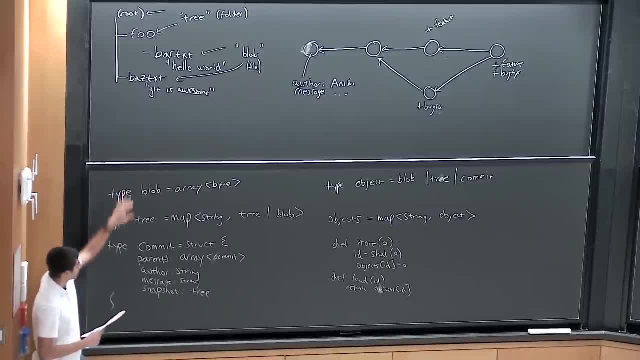 You can, almost in your head, map it to like: these are objects in a programming language like Java, and then this is a reference to a tree, so it's like a pointer, And then that is your RAM. Maybe this analogy helps, maybe it doesn't. 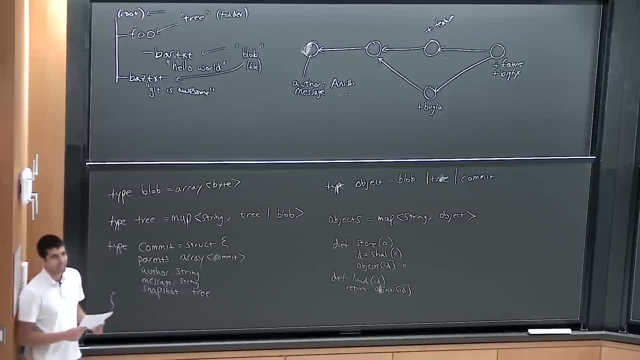 There's a memory model for storing all this stuff that you're not telling us about, but it's an object store that the index will buy and then the hash: Yeah, exactly. So I'll just repeat that for everybody to hear it on the microphone. 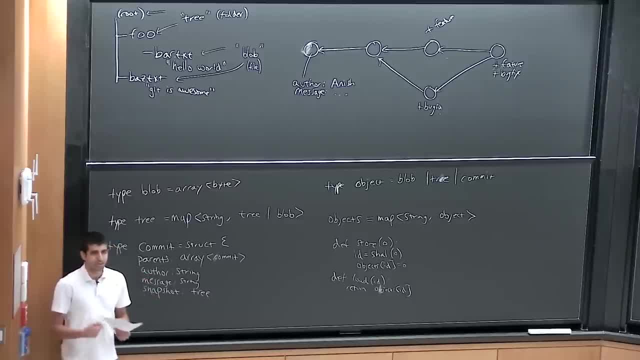 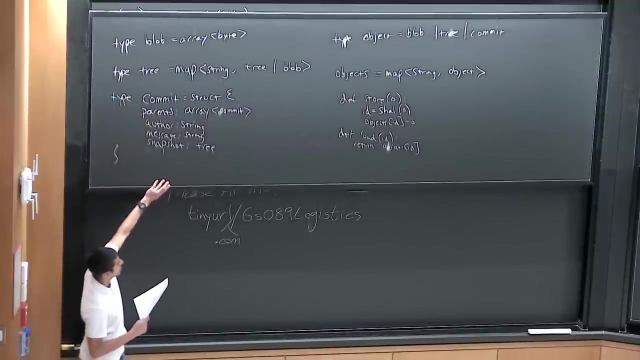 This is Git's on-disk data store. It's a content address store where objects are addressed by their hash. All right, any questions about that? so far, Okay. so now we have a way of identifying. We've unified different types of objects. 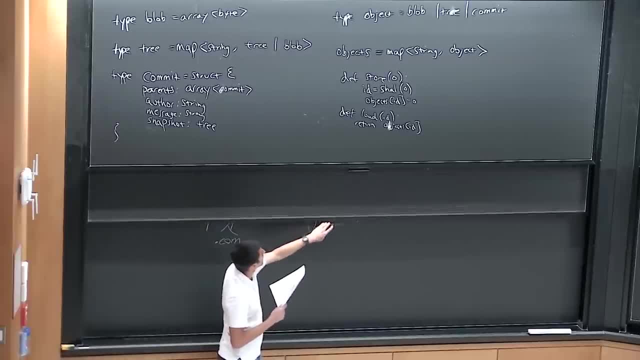 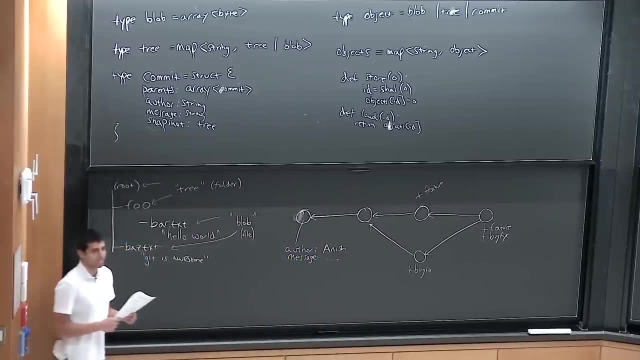 into one type of thing we call object and we have a way of identifying objects by their SHA-1 hash. What do these actual SHA-1 hashes look like? Well, they're hexadecimal strings that are 40 characters long. like SHA-1 is a 160-bit hash. 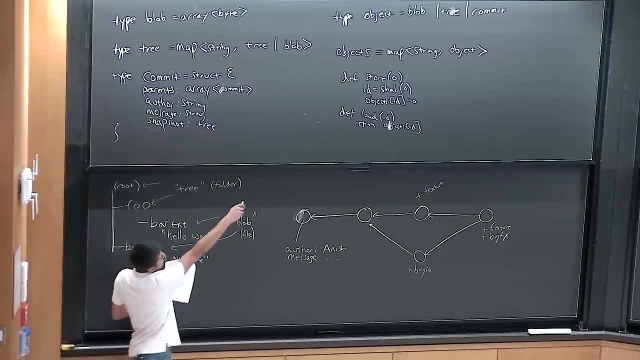 And so one of the actual IDs returned by that SHA-1 function is gonna be a really long string, And so, given that we'll have ways of identifying these different things Like this, will have corresponding to it an ID like 4AF32CB, something, something. 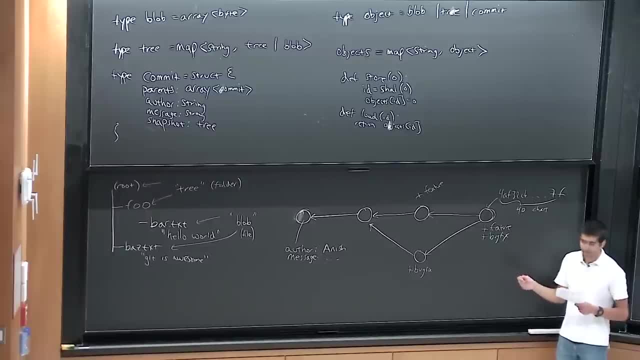 So now we have a way of naming everything in this commit graph, But these names are really inconvenient because they're super long and they're like hex strings- They're not meaningful to humans in any way. So Git's solution to this problem is one other thing. 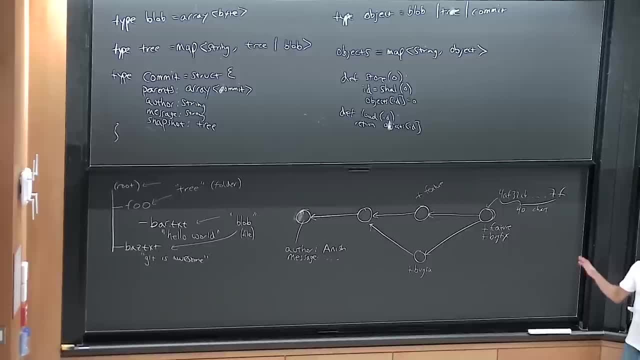 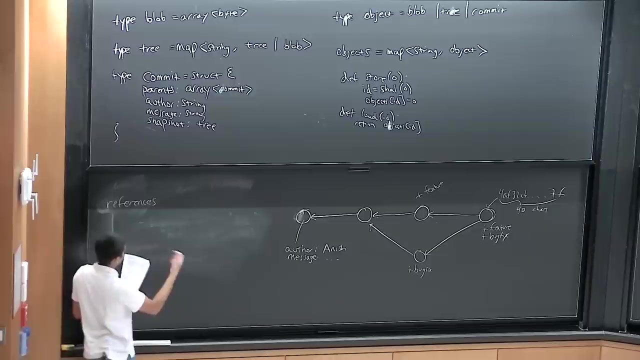 So Git maintains a set of objects and then it maintains a set of references. What are references Here? I'll erase this bit on the left, since this part's pretty logical. So references are here. So this is another piece of data that Git maintains internally. 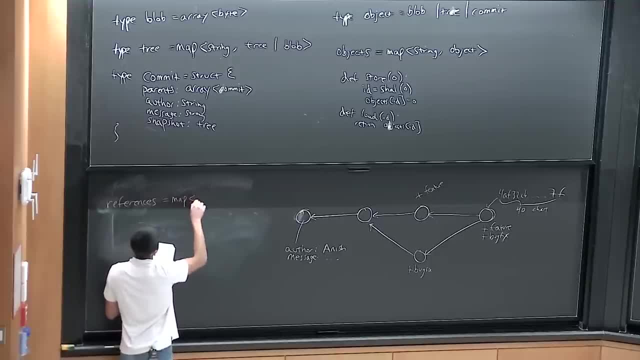 References is a map from string to string And you can think of this as mapping human-readable names, Like I might have a name like fix-encoding-bug. fix-encoding-bug is a human-readable name And this would be mapped to like 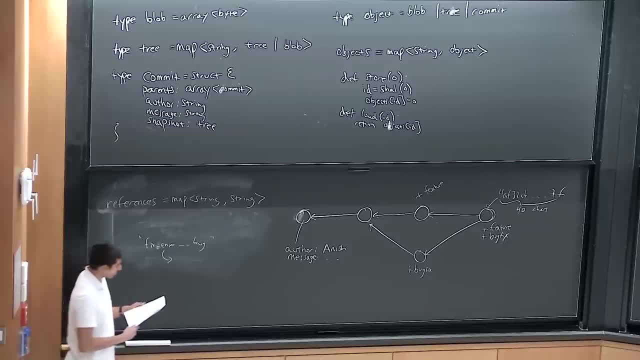 that long hexadecimal string there. And so with these references- and you can imagine how we might have ways of creating new references and updating references and things like that- With this I can now refer to things in my commit graph by name, So I might have this thing be called like: 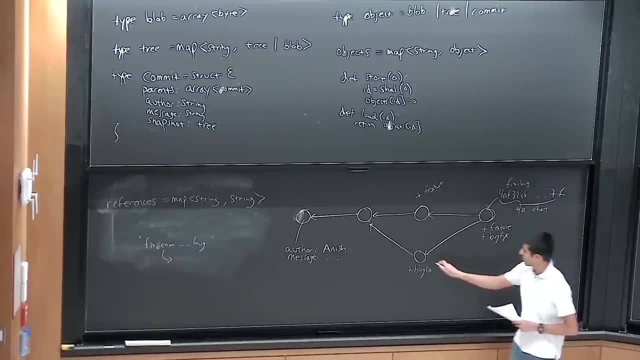 fix-bug, Or I might have a name for something over here, things like that. And so yeah, with this, Git can use human-readable names to refer to particular snapshots in the history instead of these long hexadecimal strings. One other thing to be aware of here is: given Git's design for history, this entire graph is actually immutable. You can add new stuff to it, but you can't actually manipulate anything in here. I won't go into the details of exactly how or why, but just assume that that's the case. 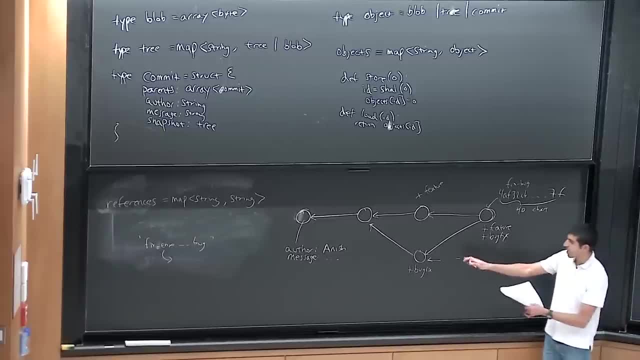 However, references are immutable. So as you're updating the history- like suppose you keep working on this piece of software- you create a new commit. So I'm representing that by the circle This points to the previous commit. I can actually have, say, my fix-bug reference. 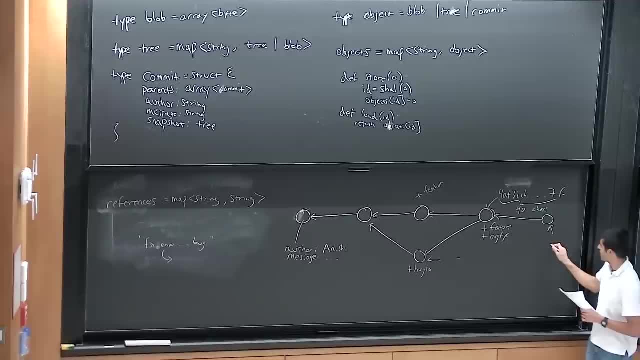 was pointing here. I can update this reference to now point over here. However, I can't, for example, make this point over here. That's not even a meaningful thing to say, because this is just the hash of this object. To change this hash, I'd need to change the contents. 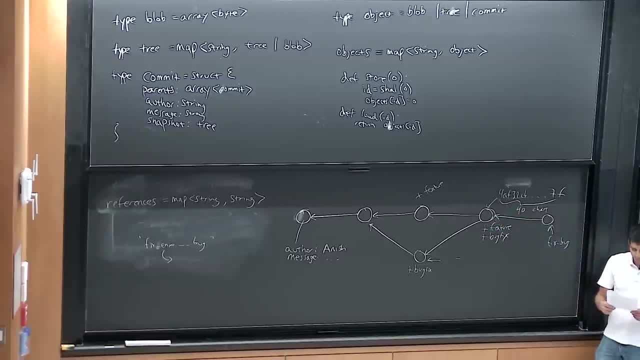 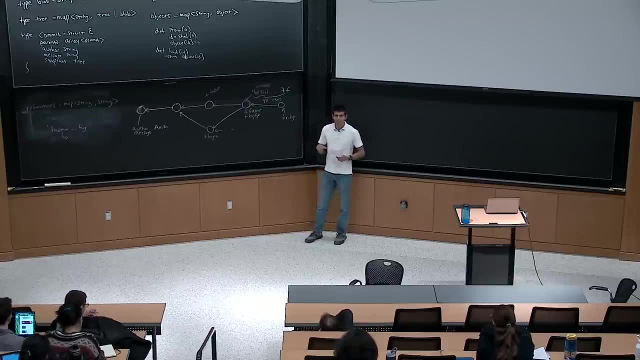 of the object, which doesn't really make sense. All right, any questions about that? so far, That's basically it for Git's data model, And then we'll go into actually interacting with Git via the command line And we'll see how Git commands correspond. 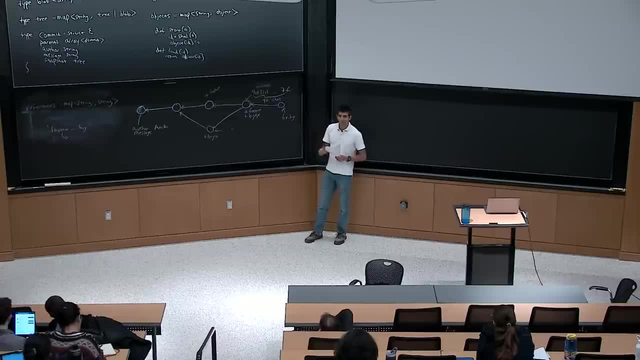 with manipulations of a graph data structure. So any questions about modeling history as trees of trees and blobs and then snapshots of these things called commits being chained together And you have references that can point to particular nodes in this graph- Cool, no questions. 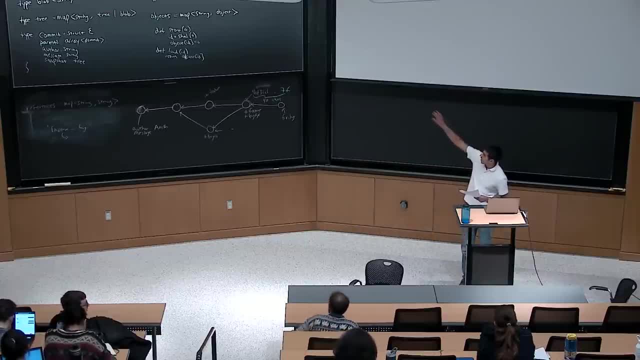 So basically, once we have objects and references, that's basically all there is to a Git repository, Those are just the two pieces of data that it stores And at a high level, all Git command line commands are just manipulations of either the references data. 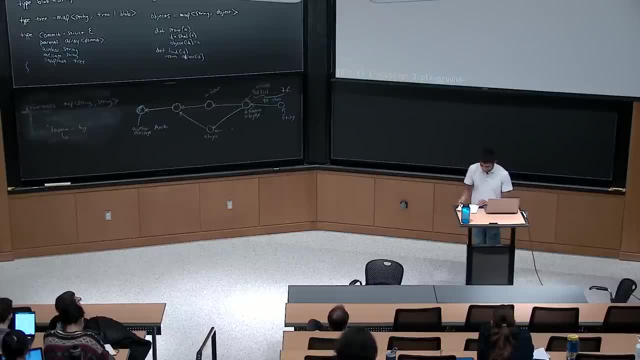 or the objects data. OK, so for the rest of this lecture I'm going to go through some Git commands. It's basically going to be an interactive demo, similar to the Vim lecture, And then you can refer to the nodes for full information. 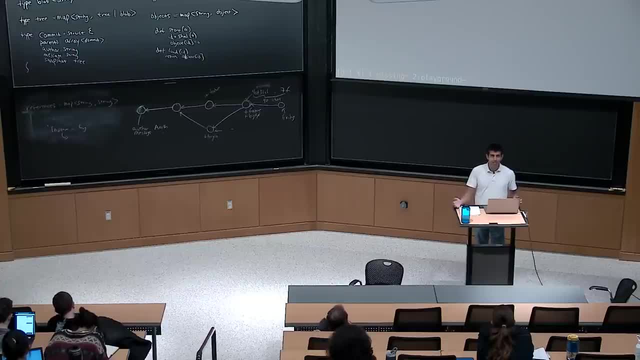 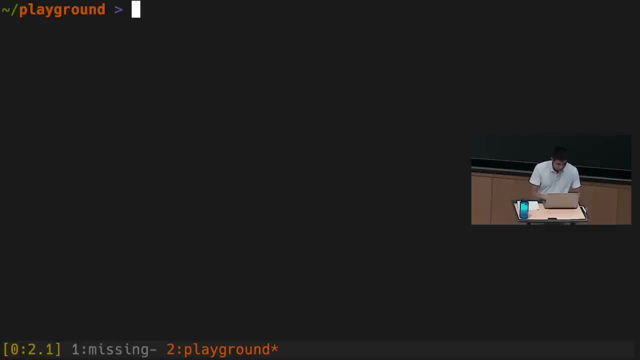 on these commands. Look, of course, this is a really powerful tool. We can't cover everything in what 20 minutes? All right, so I'm going to go over to this folder called Playground And I'm going to make a new directory called 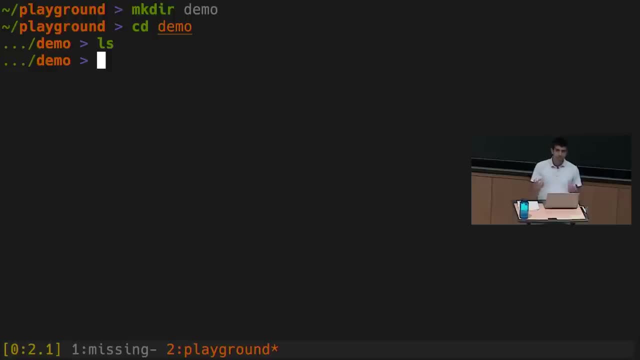 demo cd into demo And this directory is going to represent the top level of my project. It's currently empty Because I just created it. If I want to turn this into a Git repository, I use the git init command. Git init stands for Git initialize. 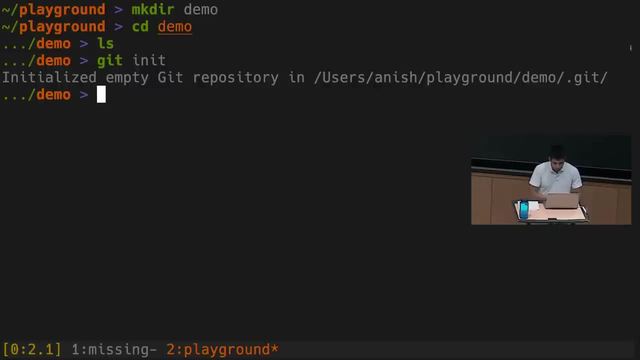 And we see that it says: initialized empty Git repository in blah blah, blah, slash git. If I do ls, I still see nothing, But if I do ls, dash a. there's a hidden file in this directory called git. 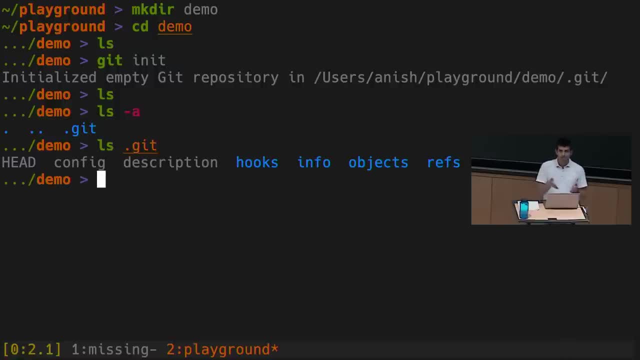 If I do lsgit, there's a bunch of stuff in here. This is the directory on disk where Git stores all of this stuff. It's internal data, Namely the objects and the references, And you actually see here objects and refs. 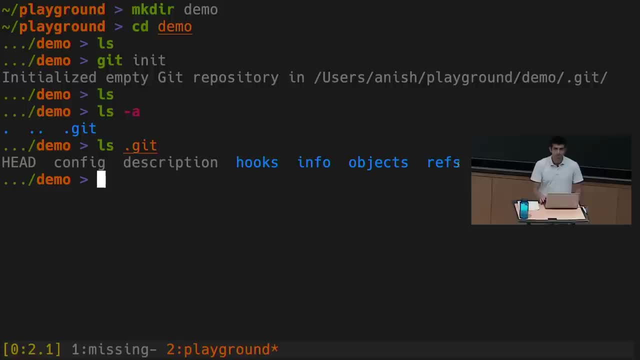 those two directories in here And all the repository data will be stored underneath those two directories. One other command to keep in mind as we're going through these is something called git help. Git help takes a subcommand as an argument and gives you some help on it. 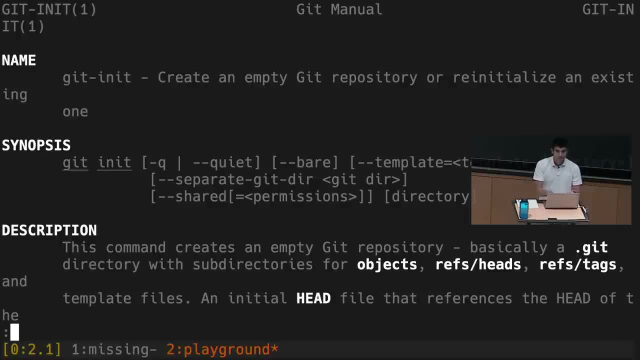 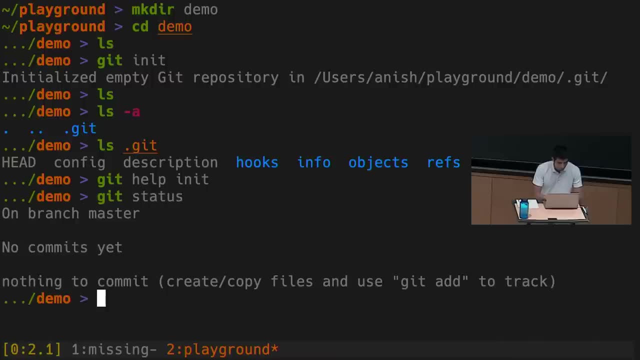 So if I do git help init, for example, it'll tell me about the git init command. So now there are some commands for figuring out what's going on with the git repository. Like git status at a high level says what is going on right now. 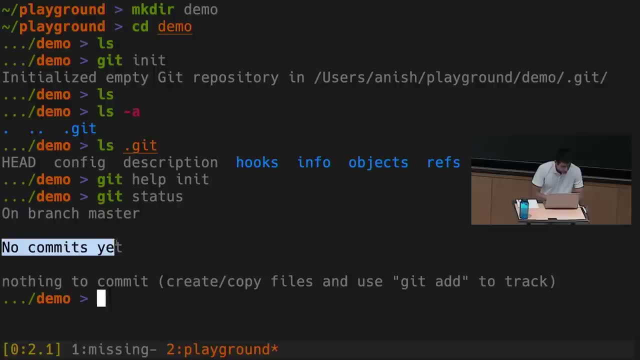 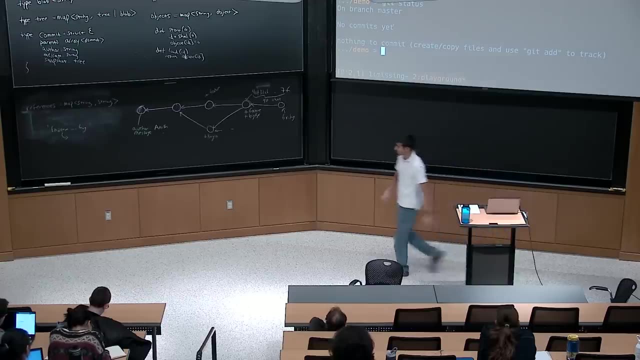 And we see here. let's ignore the first line for now. The second line says no commits, yet That's because we just initialized a fresh repository And so there is no history yet I'm actually going to. does anybody still want this? 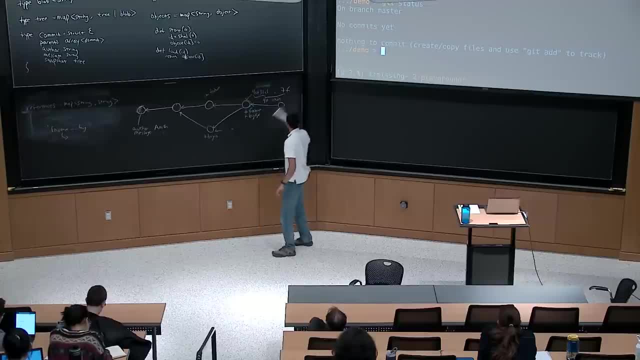 or can I clear this part of the board? I'm going to, as we go along, draw how the underlying objects and references data is changing when I type in certain git commands. So right now, this picture, or lack of picture, represents the current state of our repository. 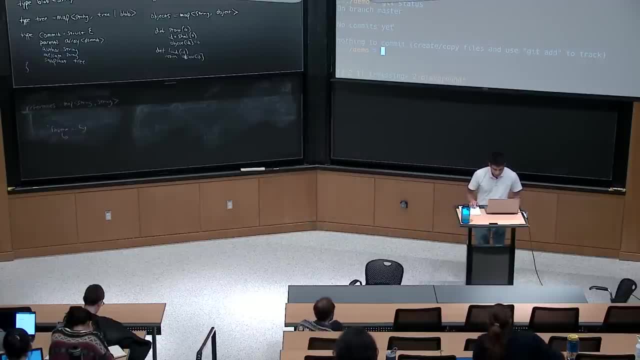 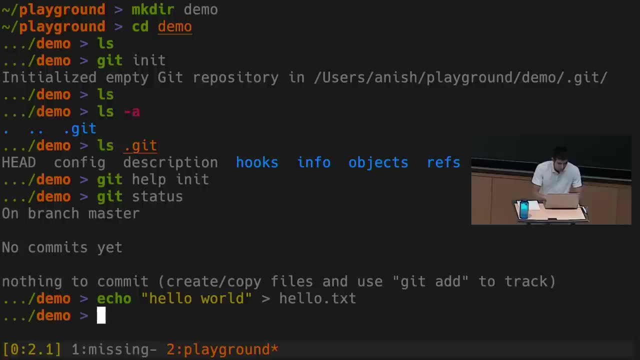 It's empty. There are no snapshots, So let's fix that. Let's add something to our history Here. we have no files, So let me just go ahead and create a file- hellotxt- with the content hello world. Normally you'd have your source code. 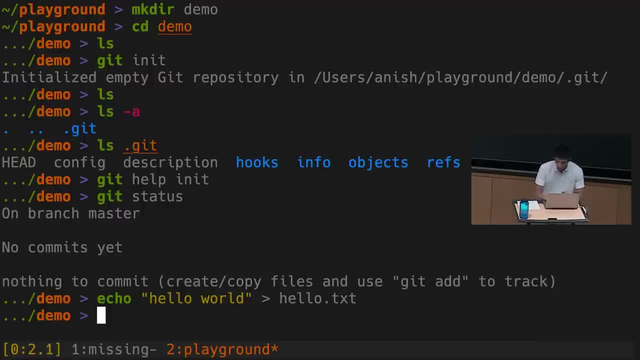 with actually useful stuff in it. Now what I want to do is I want to take the current contents of this directory and turn it into a new snapshot And I want to represent, say, the first state my project was in. You might imagine an interface for doing this. 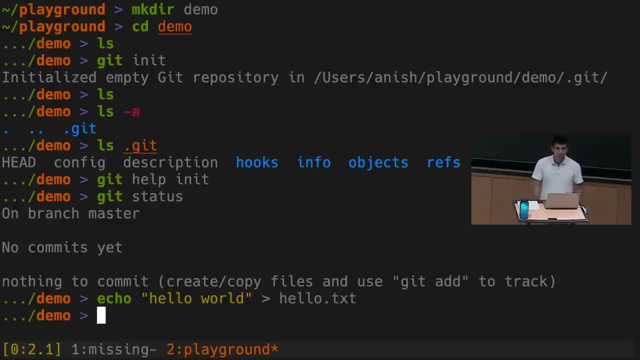 where there's like a git snapshot command or git something else command which takes a snapshot of the entire state of the current directory. For a number of reasons, git doesn't have a command that works exactly like that, because git wants to give you a little bit of flexibility. 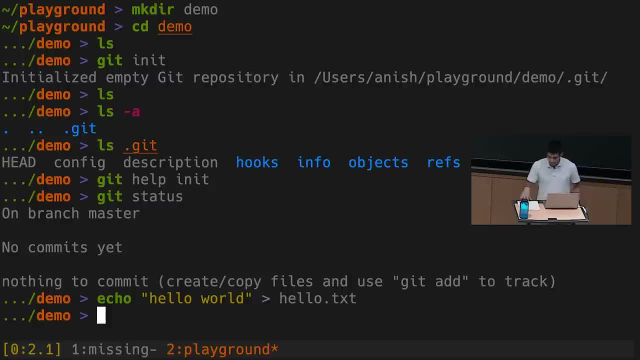 as to what changes to include in the next snapshot you take. This is something that's kind of confusing to beginners sometimes, So I'll try to explain it right now. Git has a concept of something called a staging area, and at a high level it's a way you tell git. 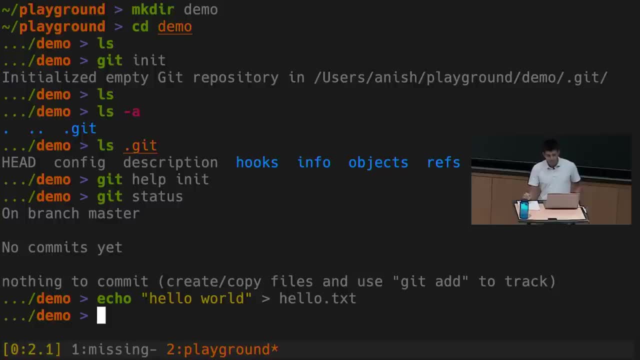 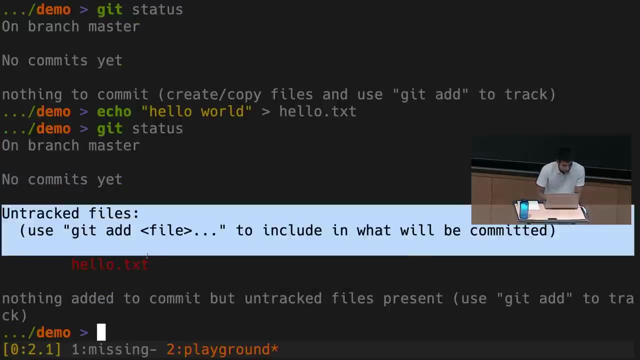 what changes should be included in the next snapshot you take? If we do git status here, we'll see that git says no commits yet, like it said before, and it says untracked files: hellotxt. So this is saying that git notices that there's a new file in the current directory. but it is not going to be included in the next snapshot. Git is kind of ignoring it for now. But if I do git, add hellotxt and if I do git status again it says now changes to be committed. new file: hellotxt. 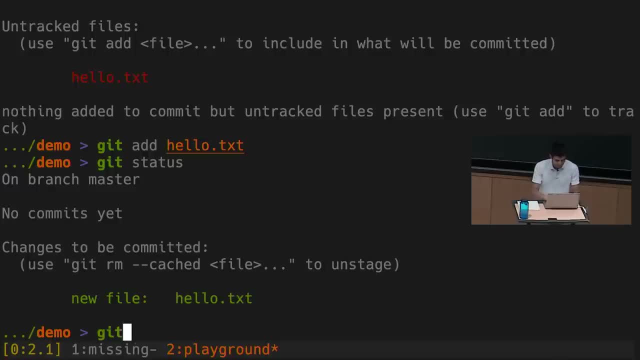 And so now, if I do the git snapshot command, which is actually git commit, which creates a new one of those circles I drew on the board over there, this file will be included in that snapshot I take. So let me go ahead and run git commit. 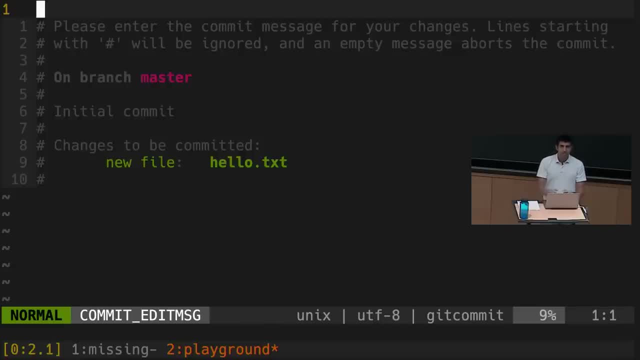 What this does is it pops up my text editor and it lets me type in a message that will be associated with this commit. And it's really good to write high quality commit messages because then later, when you're looking back at your project's version history, you'll know why. 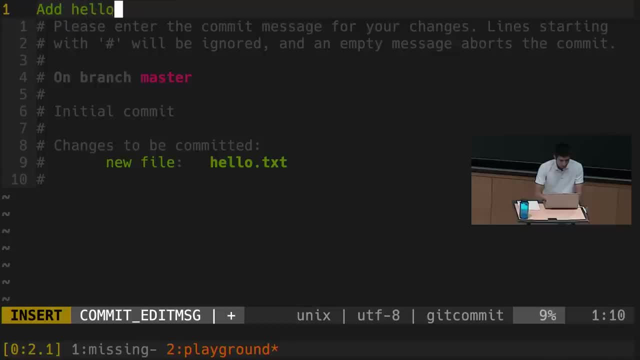 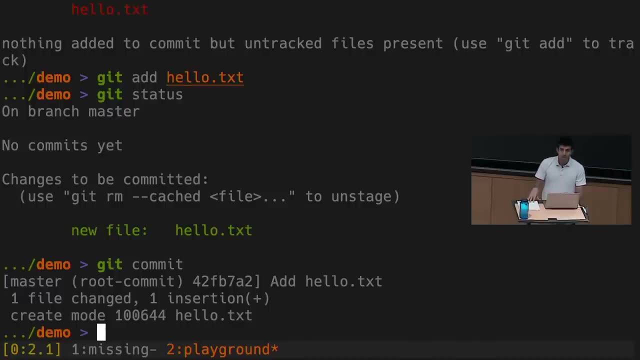 you made certain changes. I'm going to add this relatively useless commit message, but we have a link in the lecture notes for a guide on how to write high quality commit messages. So now that I've done that, git prints out some output. 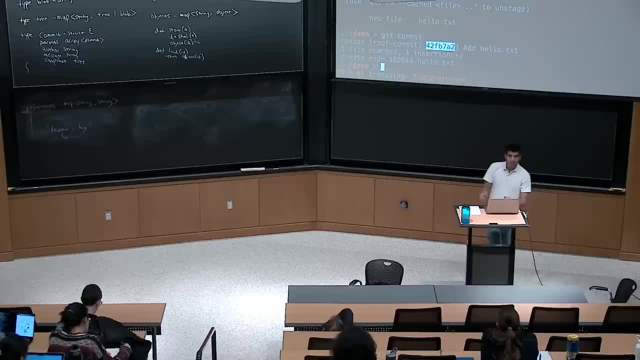 Master or ignore that bit for now. This thing is the hash of the commit I just created. So now I have in my history a single node. This has in it a tree that has a single blob, a single file: hellotxt. with the contents: hello world. 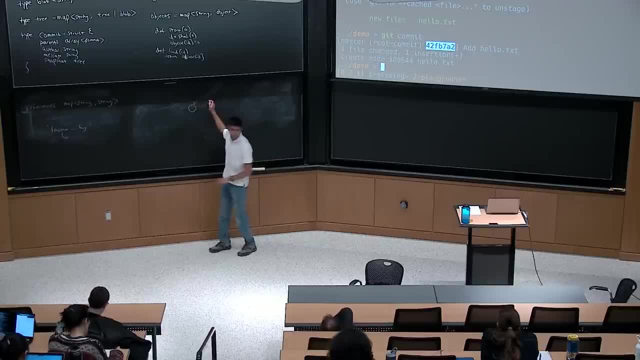 And then this has the sha1 hash 42fb, something, something, something. It's actually truncated in the git interface as well. This is just printing out my commit message again And it says: as a reminder, I just added hellotxt. 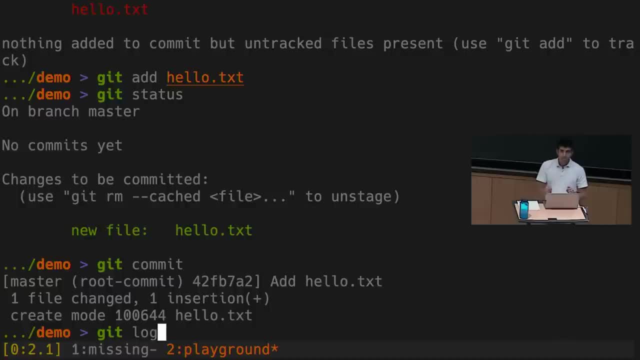 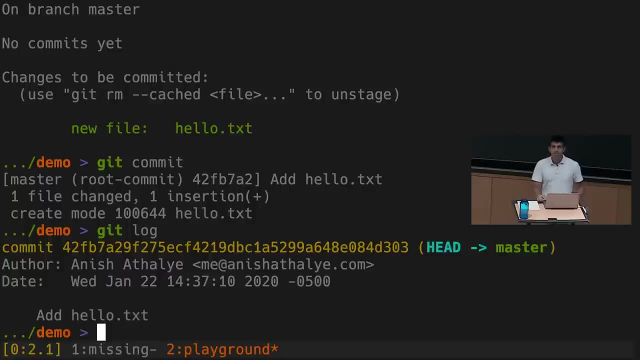 And so now if I use the git log command, so the git log command is really useful in that it helps you visualize the history. the commit graph Question: The hash of the 42f number. is that for the entire tree or just for the function? hello. 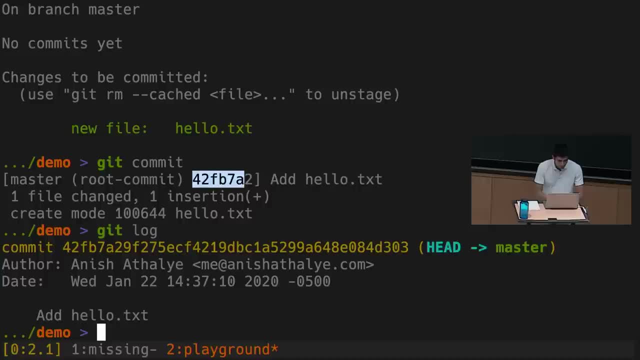 That's a great question. So the question is: what exactly does this hash correspond to? So this is the hash of the commit. The commit contains inside of it the hash of the tree, along with whatever other information. So I can actually use git cat file dash p. 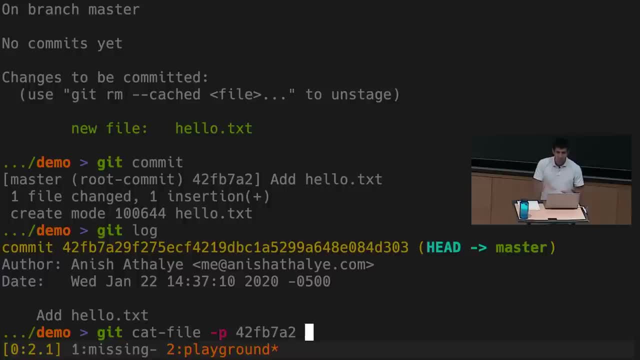 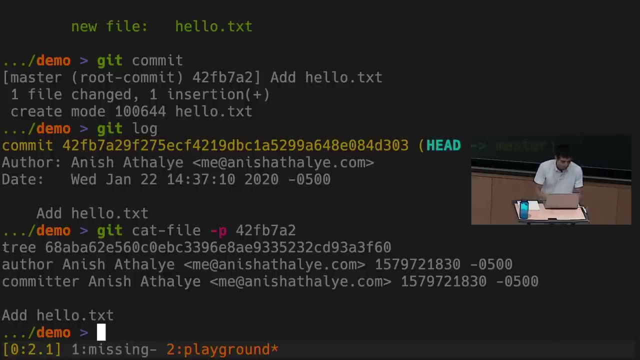 this number. This is kind of like a git internals command that will print out the contents of this commit So you can see this kind of maps to that data structure I drew on the board over there. So this commit has inside of it this tree. 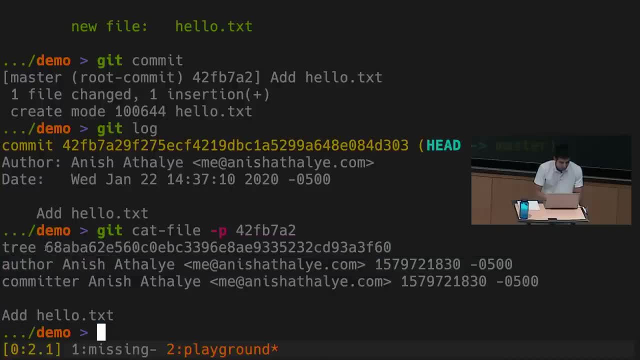 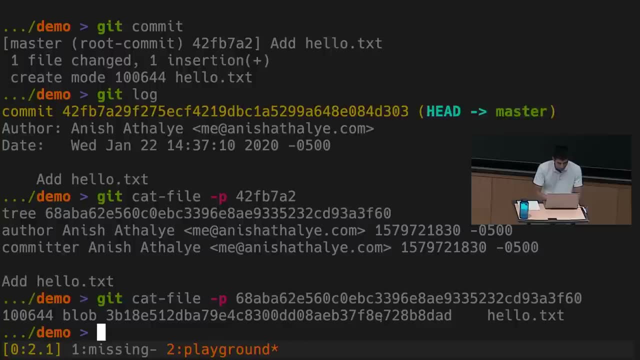 and then I'm the author and this is the commit message and so on And I can continue digging down here. So I can take this hash of this tree and do git cat file dash p. this hash Here it says that this tree has inside of it. 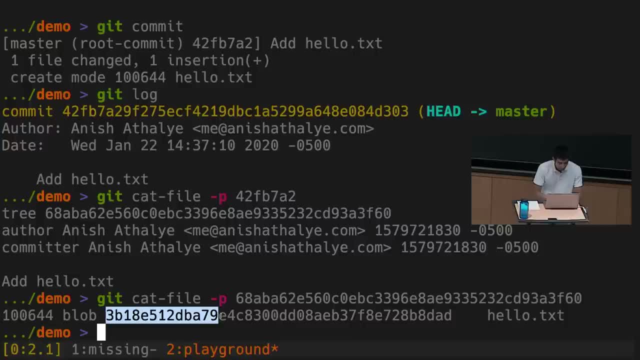 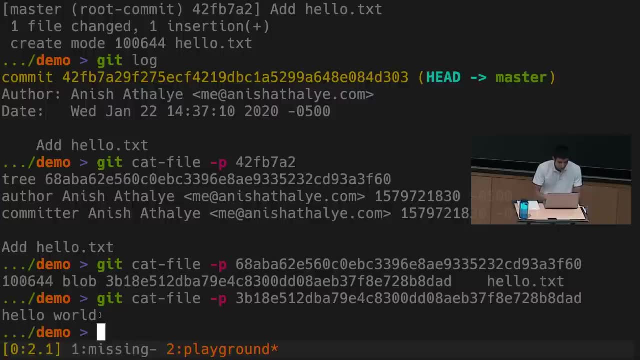 a single entry, hellotxt, and that file has: it's a blob and it has this hash. I can do git, cat file dash, p this thing and it will show me the actual contents of that file. So these are like internal git commands. 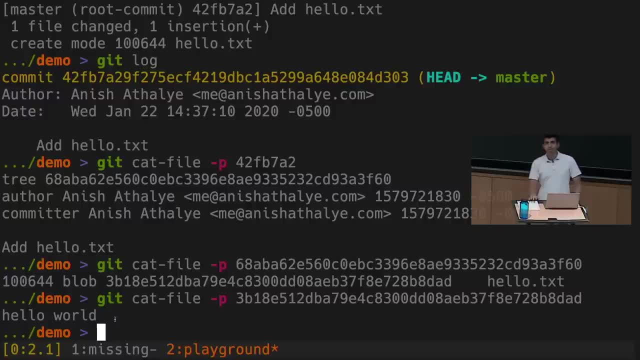 to explore objects in the object store Question. That's a great question. So the question is: why did I have to use git add? Why can't you just commit all changes? And the answer is: well, there kind of is a way to commit all changes. 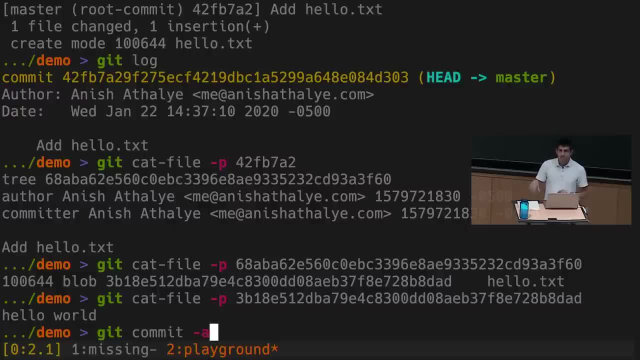 If you do git commit dash a, this commits all the changes that were made to files that are already being tracked by git. so anything that was included in the previous snapshot but has been modified since then, It doesn't include new things. There's also variants of git add. 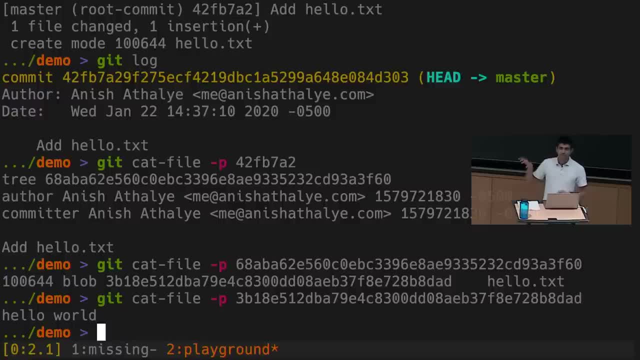 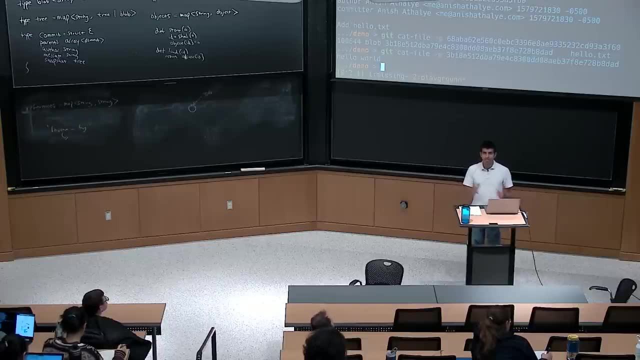 like, if you do git add, colon slash, this will add everything from the top level down of your repository, But at a higher level. the reason we have the separation between git add and git commit and why git commit doesn't just snapshot the entire directory. 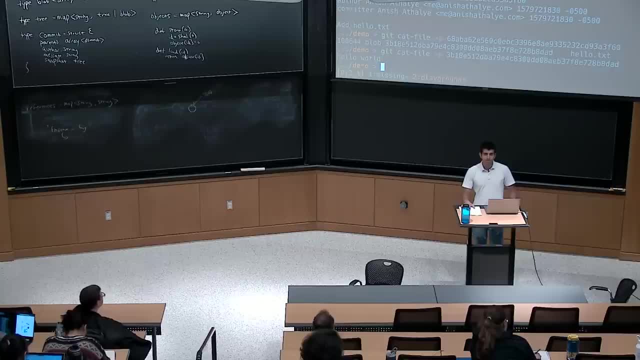 is that there are often situations where you don't want to include everything in the current snapshot, Like. here's a couple examples. One is that I might be hacking on my project and I go ahead and implement two features. Maybe I don't want to have a single snapshot. 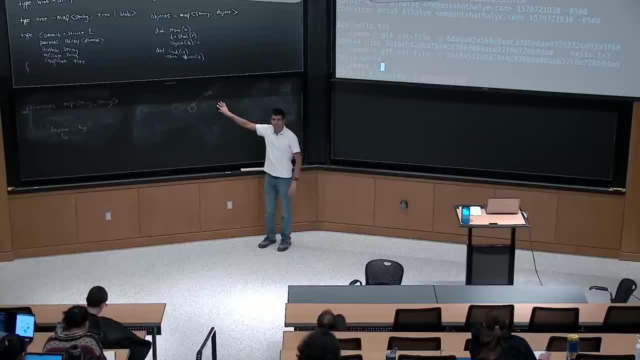 that comes after this one. that's like I implemented feature a and feature b. Maybe I want to create two separate nodes in the history so that it looks like first I implemented feature a and then after that I implemented feature b. So I have one snapshot that only includes a. 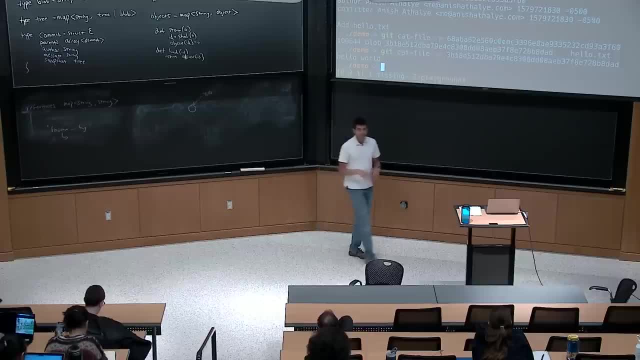 and then the next one includes both a and b. Git add is a tool and, like the staging area in general, is a tool that will allow me to do that sort of thing. Another example is suppose I'm working on a bug fix. 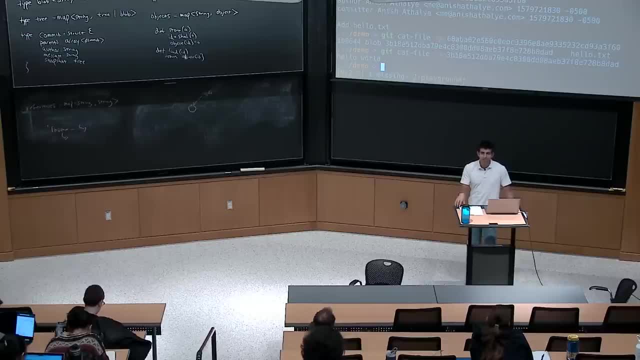 and I have printf statements, I've put all over my code and then finally I find the bug and there's a plus one somewhere where there shouldn't be a plus one. so I go fix that. And then I want to take a new snapshot, right. 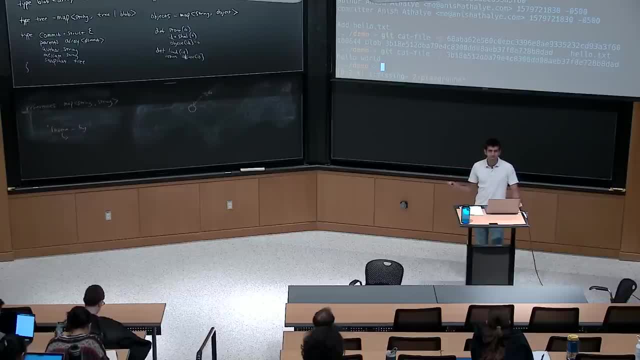 with my fix. But the snapshot probably shouldn't include all of my print statements. It just needs to include the fix of removing that plus one. So one way I could solve that issue is I could go and manually remove all the print statements. but git has a much better way of doing that. 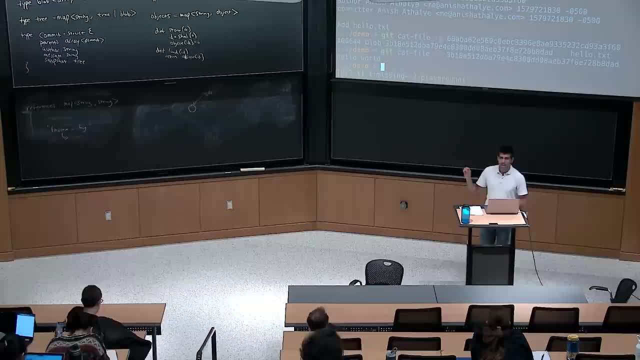 There's actually a way to specify that. I only want to add the change of removing that plus one. then I can commit that, take the new snapshot and then I can throw away all the other changes. There are commands for doing that and some of them are linked in the lecture notes. 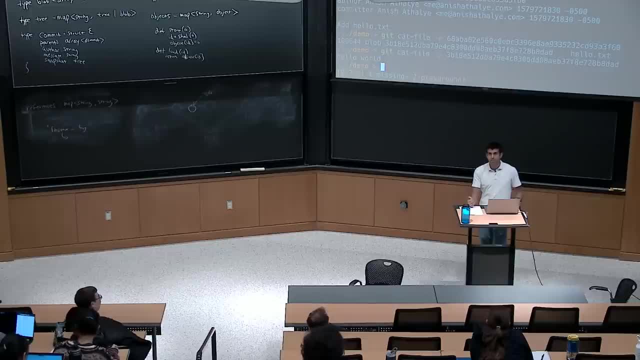 So those are two ways in which you can use the staging area to help you, and why there isn't just like a snapshot everything. command Log files is another example. Yeah, so Log files in your directory. Yeah, John points out that yet another example is. 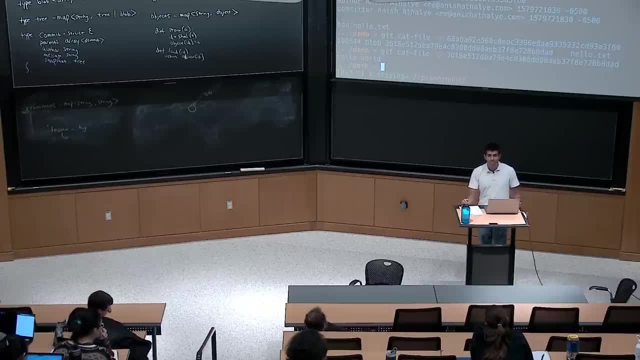 you might have log files in your current directory that your program runs on, but you don't want to include those when you run it and you probably don't want to include those when you take a snapshot. There's probably other things, like if you compile your project. 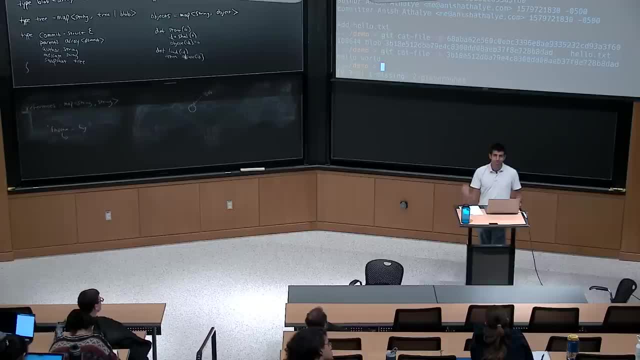 you end up with a bunch of o and f files. You probably don't want those to be part of your history. So, going back to what I was showing you before, I'm going to clear the terminal screen and then show you the git log command. 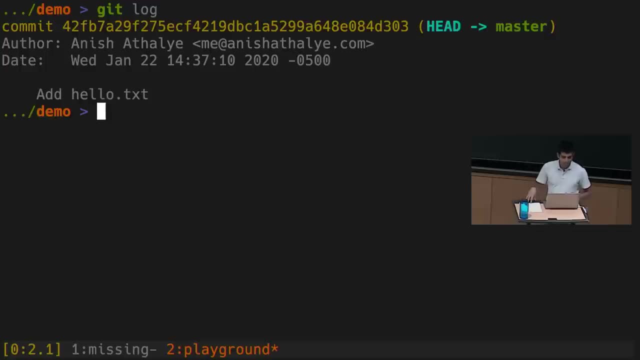 So git log lets you visualize the version history, and this is an incredibly helpful command. By default, git log shows you a flattened version of the version history. So, even though the version history is a graph, this will linearize it and just show things in order. 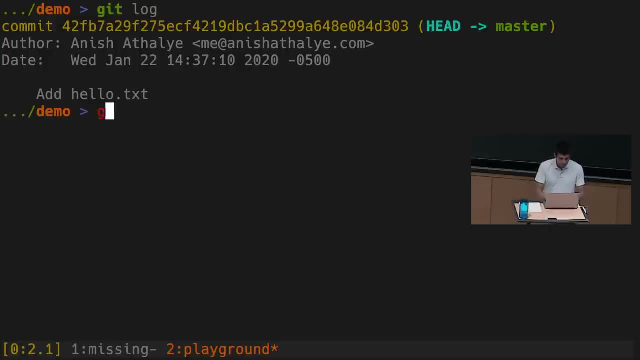 I personally find that confusing, so I almost never use git log And instead git log takes some arguments that actually show the history as a graph. So you can treat this as a magic incantation for now, and you can read the documentation. 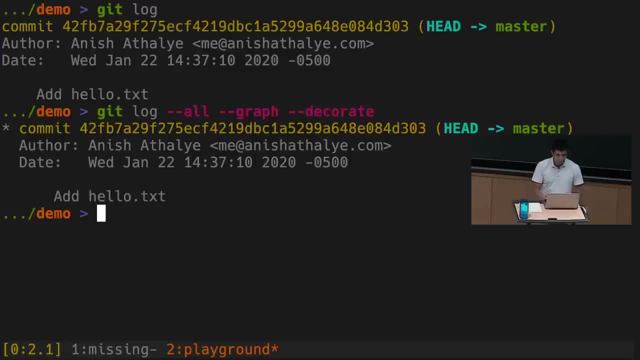 if you want to figure out exactly what each of those flags does. But for now this doesn't look all that different because we only have one node in our graph, So visualizing it as a flattened thing versus a graph doesn't look all that different. 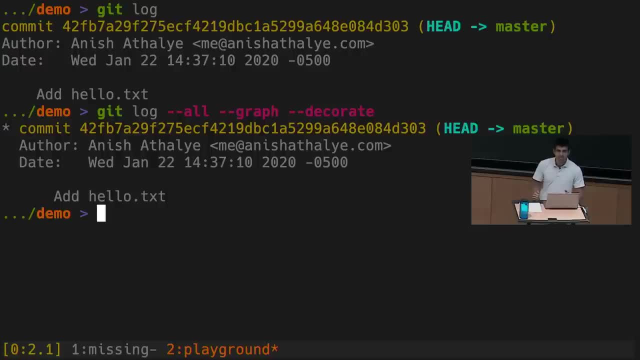 Let me go ahead and create a new snapshot and then we can run this command again and then see exactly what it does. So I will put another line into hellotxt and so if I cat hellotxt, it has the thing it had before, plus this. 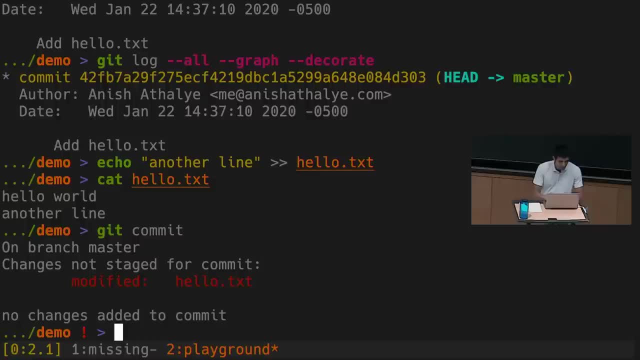 I can do git commit and notice this doesn't do anything. It just says no state, no changes staged for commit. Why is that? It's because I didn't add this to the staging area. I didn't tell git that like. 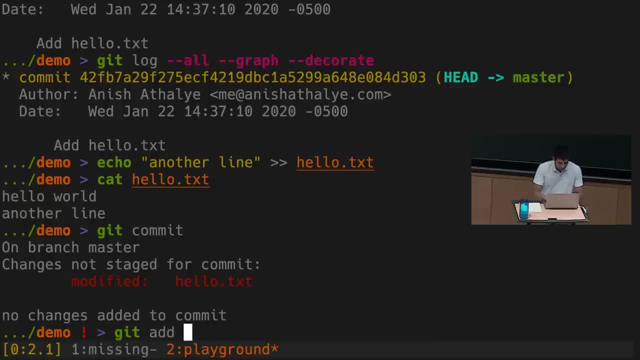 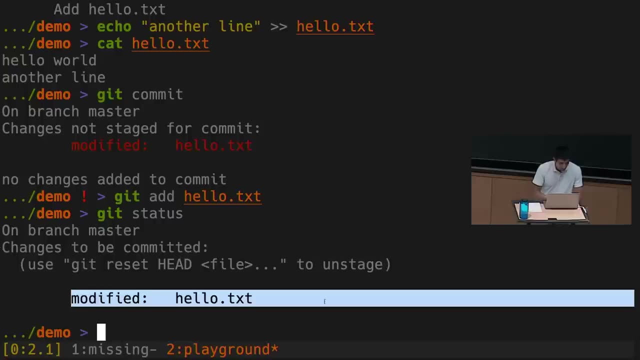 this is something that should be included in the next snapshot. So if I do git add hellotxt git status, it says, okay, this change is ready to be committed, this modification to this file, And now I can do git commit. 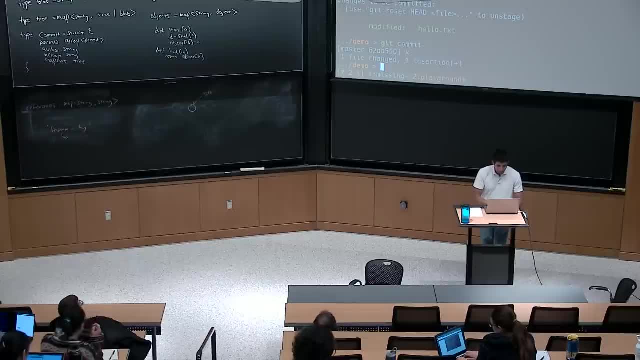 I'm going to put in a useless commit message and the new change has been made, And so now my history has another node in it. and then this node has some hash that's shown on the screen. And now, if I rerun that command from earlier, 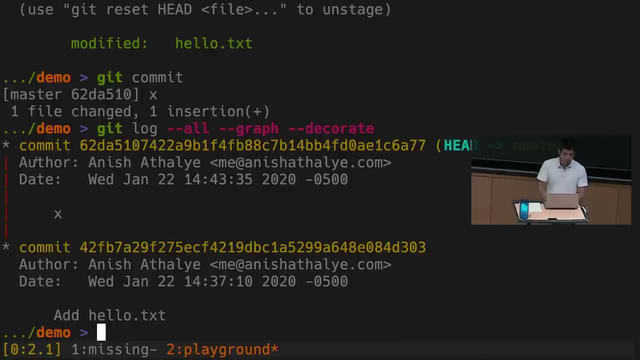 the git log. with all these arguments, it actually starts looking more like a graph here. Notice that this is like that graph turned this way: The more recent, so it's shown vertically, not horizontally, and the more recent commits are shown at the top. 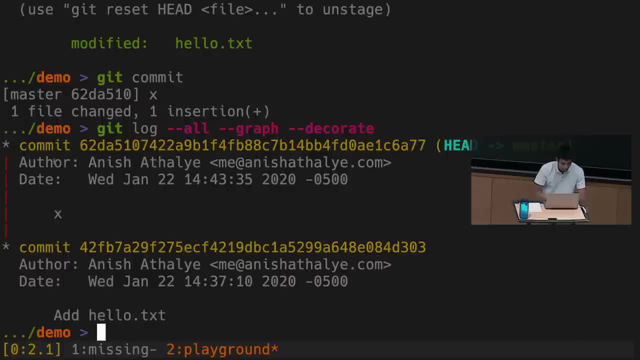 This is showing one commit. This commit hash shows a bunch of metadata, including the commit message, And then this is the part I want to talk about next. So remember, we talked about objects, like the actual contents of your repository, and then we talked about references. 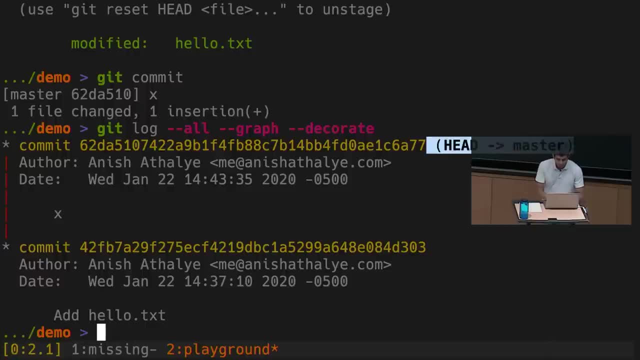 ways of naming things in the repository with human-readable names. So master is one reference that's created by default when you initialize a git repository and by convention it generally refers to like the main branch of development in your code. So master will represent like 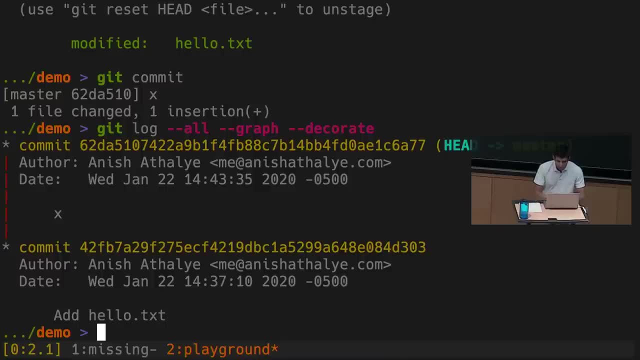 the most up-to-date version of your project. So here you can think of master as a pointer to this commit, And as we add more commits this pointer will be mutated to point to later commits. And we also see here head. This is a special reference in git. 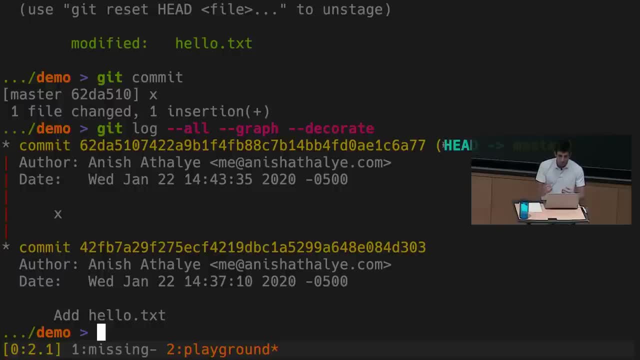 It's a reference like master, but it's special in some way, And head basically is used to refer to like where you are currently looking right now. Any questions so far? Yeah, question, So normally when I've used git. 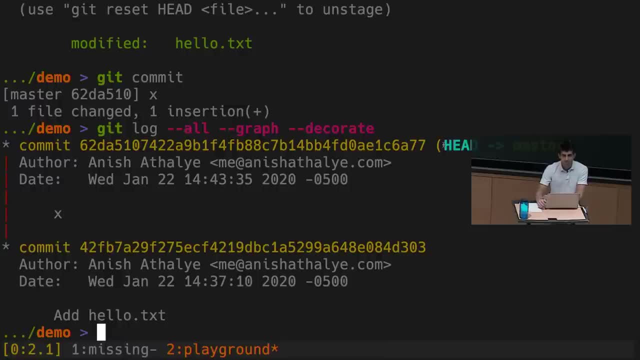 it had to do with git hub and there was like a part where you had to make an account online and you haven't done any of that. Is that like a separate thing, or is it all related somehow? That's an excellent question. 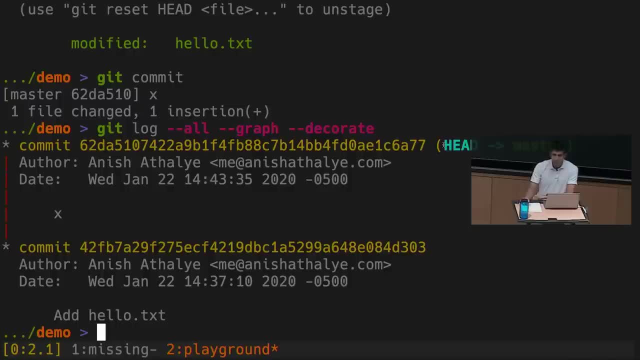 So the question is: worked with git hub before and you had to create an account to do that. How does git hub relate to git? And the answer to that question is: git hub is a repository host for git, So you can create an account on git hub. 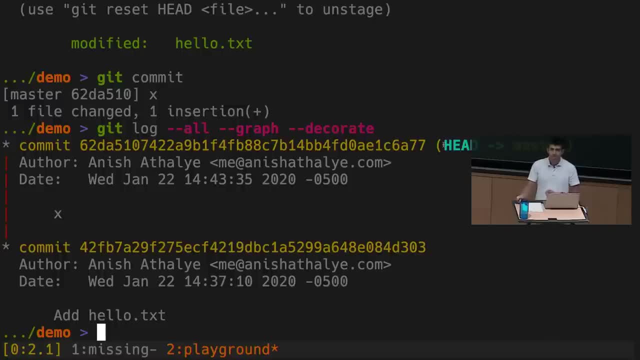 and store a git repository there and use that to collaborate with other people. But git as a command line tool is just independent from git hub, So you don't have to use git hub to use git. You don't have to use git hub. 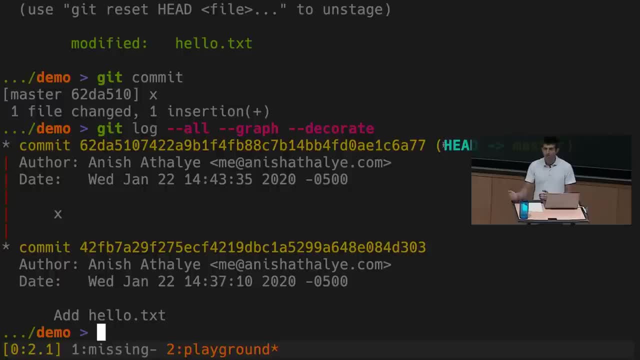 to collaborate with git either, Like there are other providers of git repositories, like bitbucket or git lab or things like that, And so, yeah, git hub is a host for git hub repositories. Any other questions? So, after we make this, 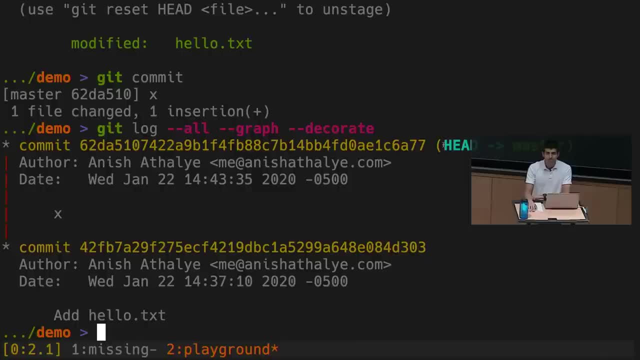 after we commit and make this git hub not git hub, we make this git right ahead in the master and we have two things in it shown in the graph. if we want to put it up on git hub, that's a separate set of commands. 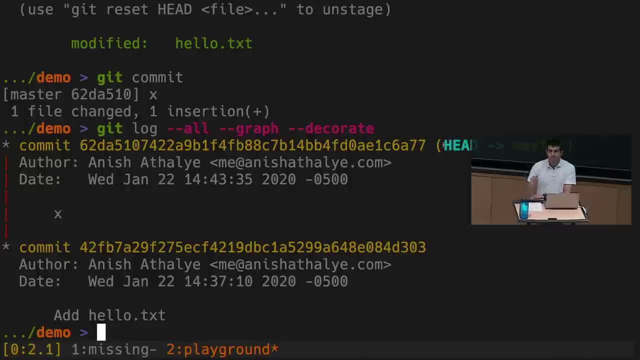 and a need for login and stuff like that. Yeah, so the question is: if you want this repository to end up on git hub, how do you do that? Yeah, there's a separate set of commands for doing that. There's a. 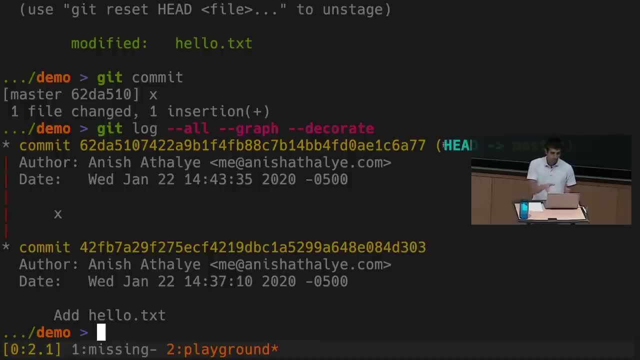 so that concept of having your local copy of version history interact with another copy, so the other copy's called a remote. and then there's a set of commands for interacting with git remotes and sending data from your remote or from your copy to git remotes. 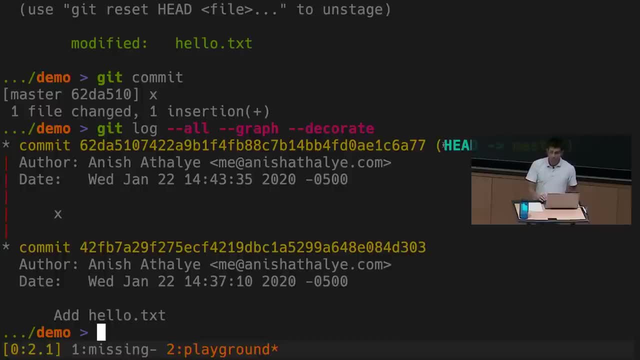 and getting data from git remotes into your local copy, and we'll cover that later in this lecture or maybe in the lecture notes. John might make a supplemental video to go along with this lecture. Any other questions? Okay, A couple other basic commands to show you. 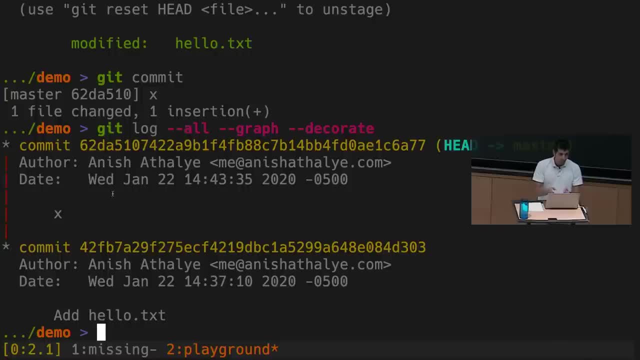 So so far I've shown you a version history and we've taken a file and modified it, but we haven't really made use of the history in any way besides reading the messages. so one useful git command is something called git checkout. 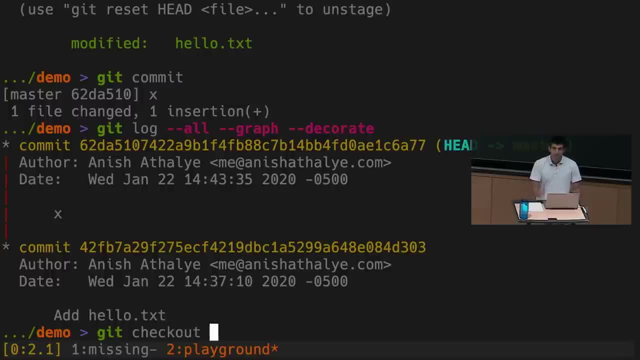 and this is a kind of wacky command. It lets you do a bunch of different things, but one thing it lets you do is move around in your version history. so one thing I can do is give git checkout the commit hash of a previous commit. 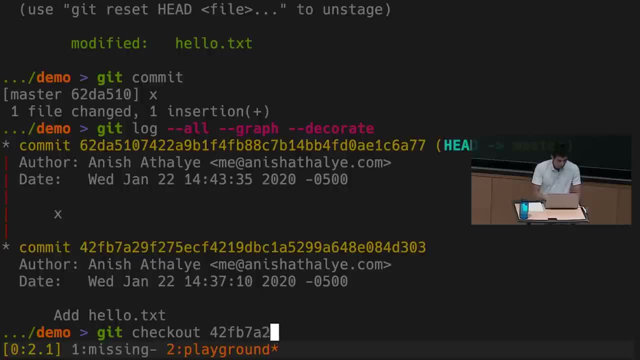 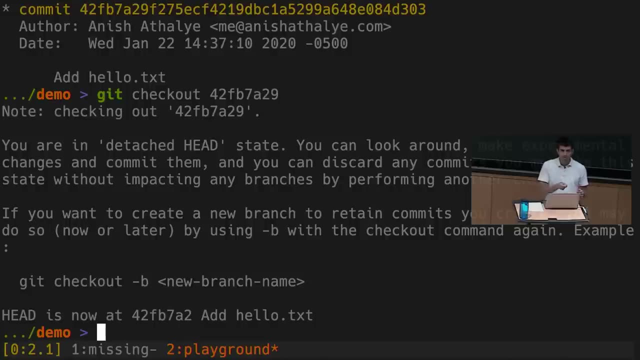 and I don't need to type the whole thing. I can give it a prefix and it's smart enough to figure out what I'm talking about. and what this will do is it will change the state of my working directory to how it was at that commit. 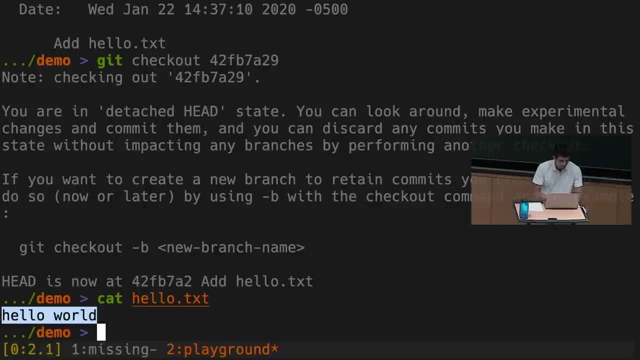 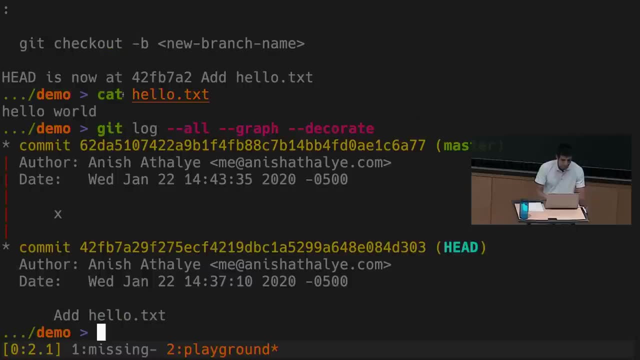 so here, if I do, cat hellotext recall that I had only one line in here before at the first commit and later I added that second line. Now, if I do that git log command and this command is super helpful. 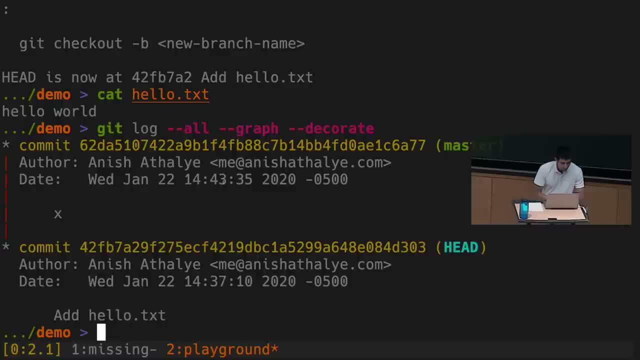 It shows you all the things. If I do this command. notice that this output looks a little bit different than before, Like my actual history contents, the commits themselves and the way they relate to each other and all that have not changed. 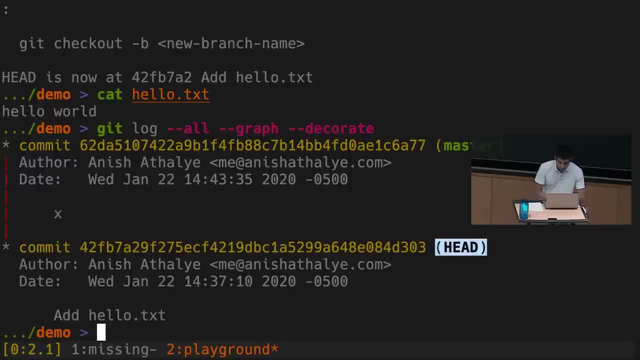 but the references have so notice that head is down here, even though master is still up here, so at high level. what this is telling me is- this is what I'm looking at right now, If I want to go back here. 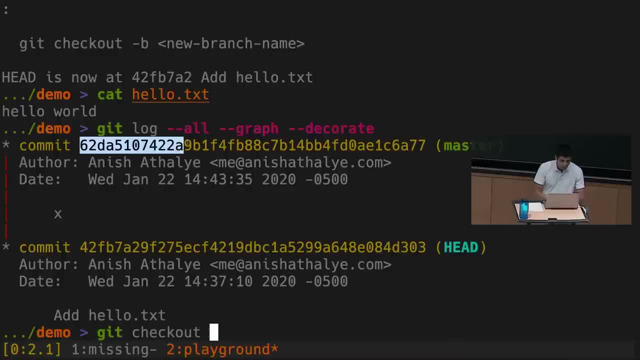 I could type git checkout and this commit hash. Does anybody know a different thing? I could type here instead of this long hash in order to go back to this commit: Yeah, You can give it the name of this is a branch colored in green here. 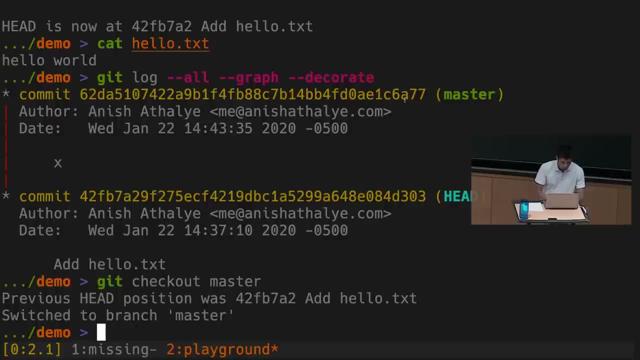 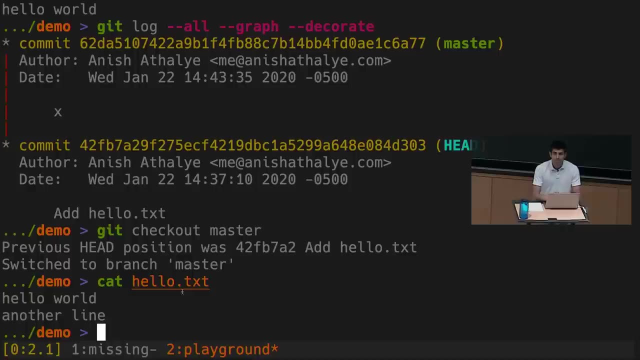 and it refers to this commit, so I can give it the short name or the human readable name instead. And now, if I do cat hellotext, notice that it has that second line. So when you do checkout it is actually working, it is actually replacing the files. 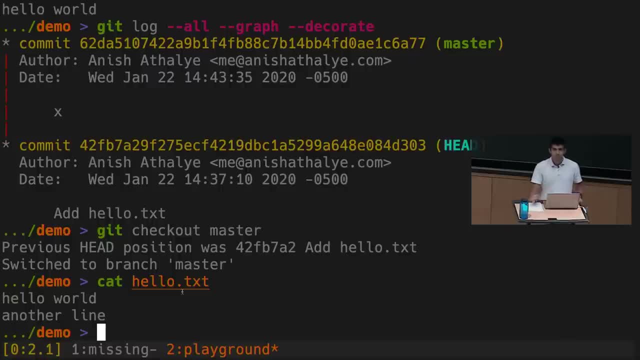 in your current directory with the files of lots that it has stored. Yeah, So all your files. so it's like you could change a whole bunch of files without even realizing it. Yeah, so to repeat that git checkout actually changes the contents. 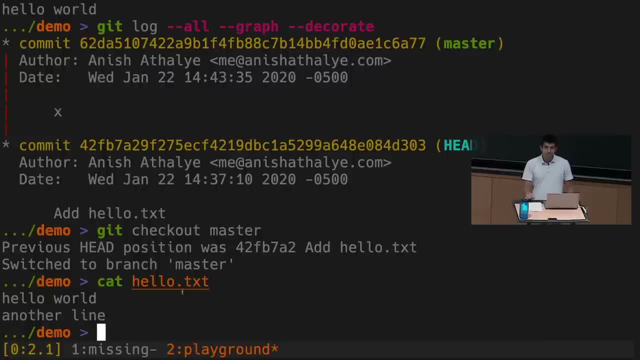 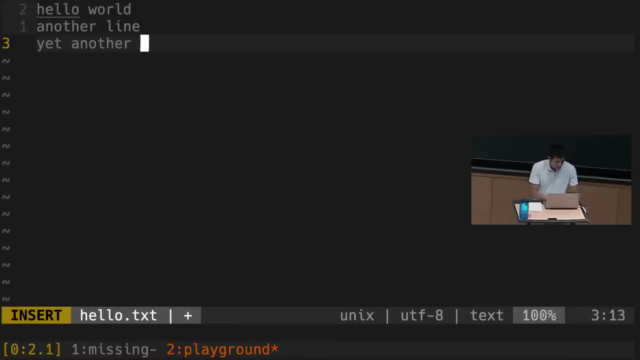 of your working directory and so in that way it can be a somewhat dangerous command if you misuse it. For example, you can see if I modify hellotext and then try that git checkout command from earlier, actually notice here that it says error. 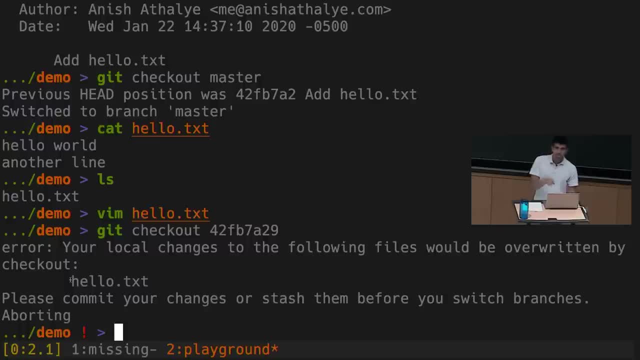 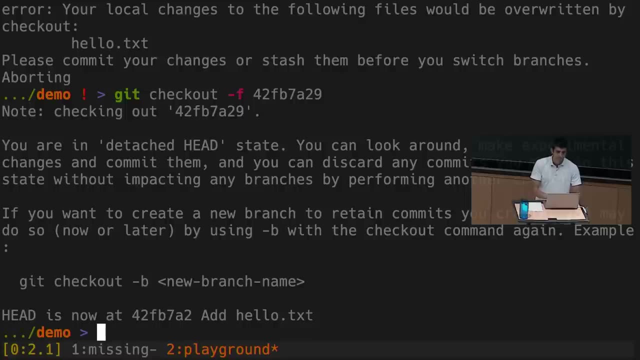 It says there's a file that's been modified and the git checkout would destroy your modification. You probably want to do something about that. But there are flags like, for example: git checkout, dash f does this forcibly, and now it's thrown away my changes. 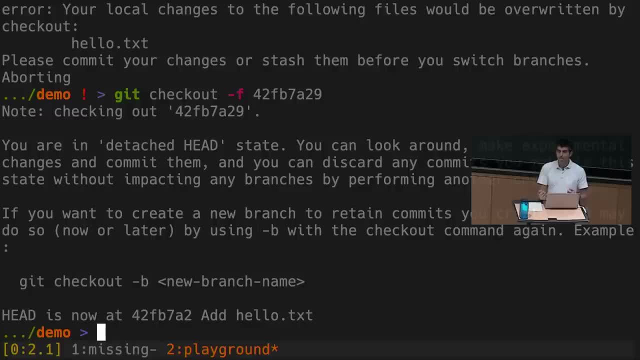 So yeah, git, checkout has the potential to well. it certainly does modify things in your working directory and it can actually destroy changes if you're not careful Question. So then in the lingo here, checkout moves where head is. 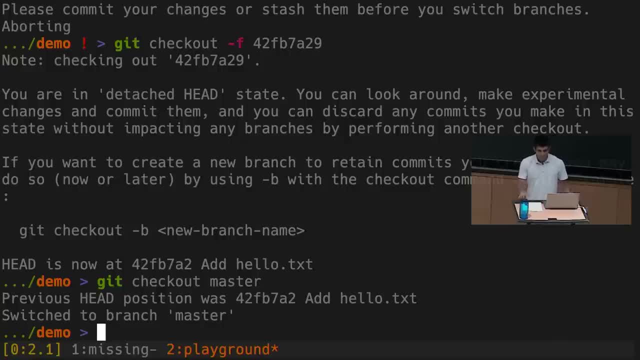 Exactly Okay. Yeah, this is exactly what I want you to be thinking about: How these, like the crazy git interface commands correspond to mutations to this graph and mutations to the reference, or like additions to the graph and mutations to the references map. 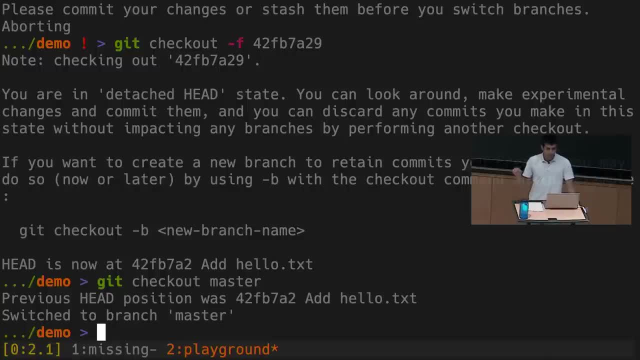 So yeah, exactly, Git checkout moves the head pointer and then also mutates the contents of your working directory with the contents that the head pointer now has, And so that the head pointer now points to corresponding to that commit. Any other questions? 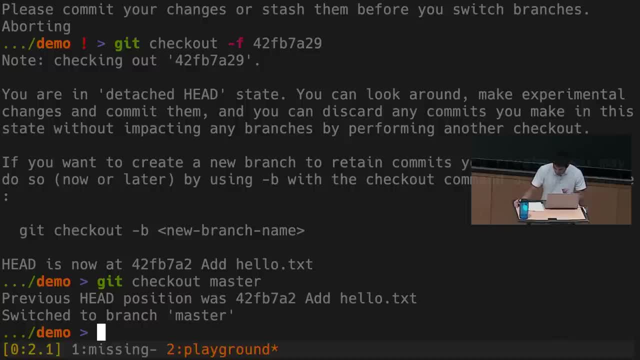 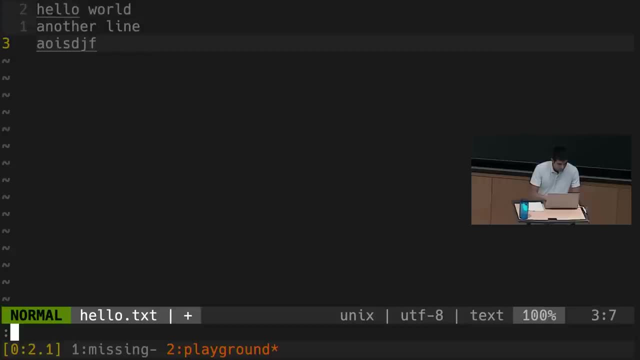 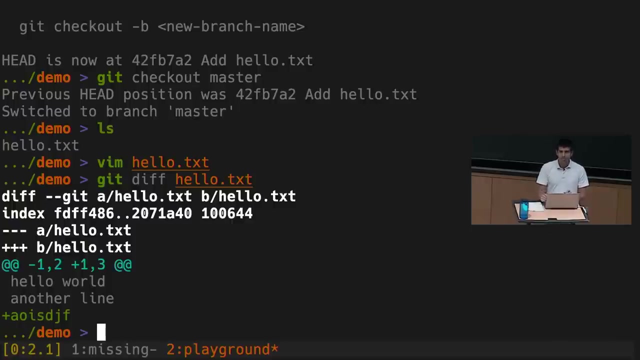 All right. So one other basic command I want to show you is the git diff command. So I'm going to modify this file and put some changes in it. The git diff command can show you what's changed since the last snapshot. It's just helpful for like knowing. 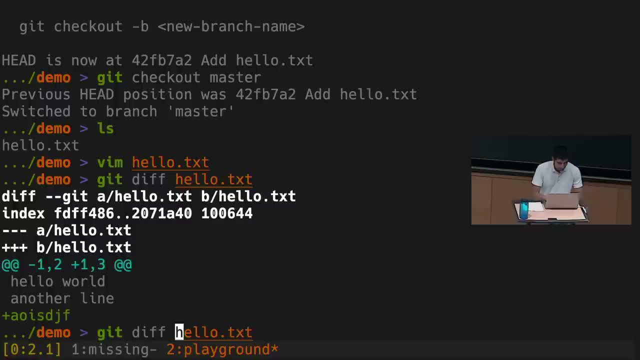 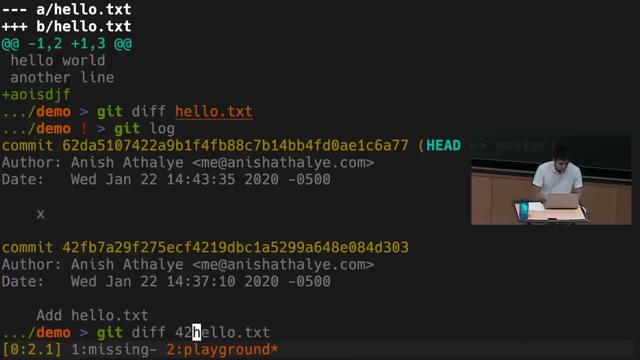 what's going on with your project. Git diff can also take extra arguments, like you can do git diff and say: compute a diff not with respect to the last snapshot, the last commit, but with respect to this. And this will say: 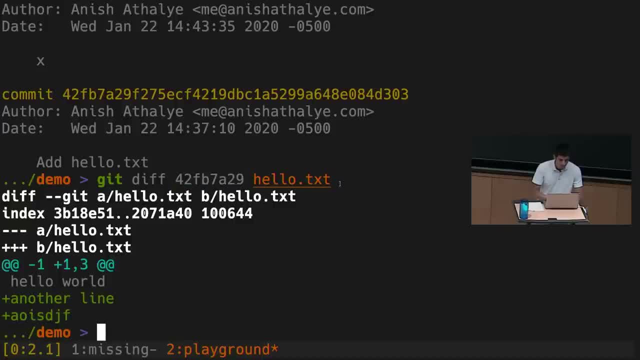 okay, two lines have been added since this point to hellotxt Question. So if you don't supply like a hash, what is it? Ah, so the question is: what does this command do without this extra argument here? That's a good question. 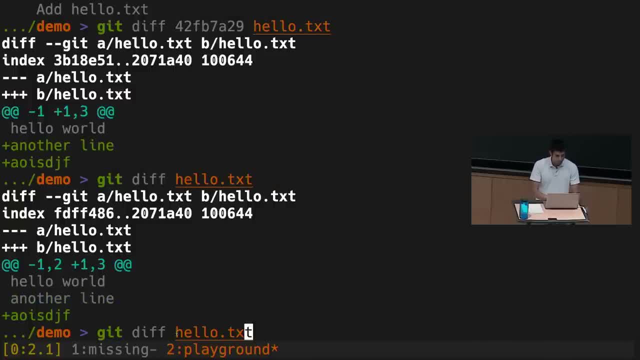 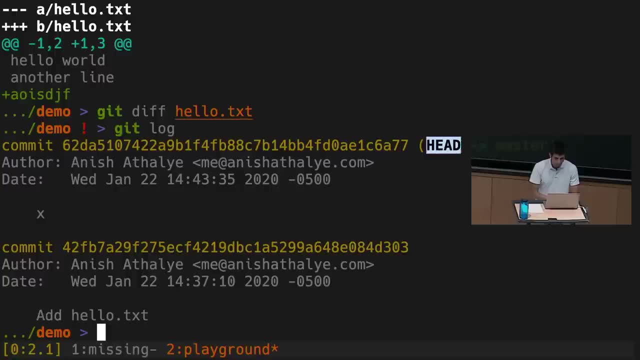 So what this does is it computes a diff with respect to head And looking at my git log, head is pointing to here. so it's doing a git diff with respect to this commit And you can actually specify that explicitly. You can do git diff head hellotxt. 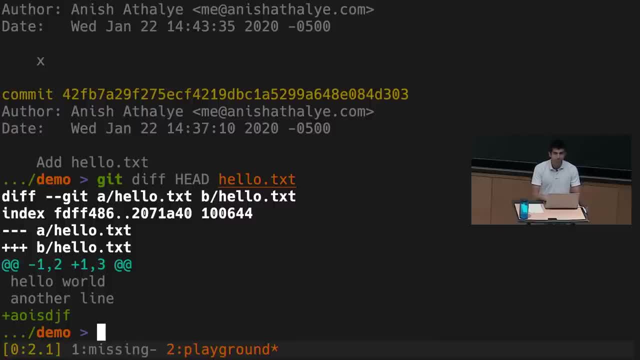 and it will do the same thing. Isn't head? wherever head is? isn't it going to like, modify hello to? I guess I don't understand how head can be somewhere and hello can be different from like where head is on the ground. 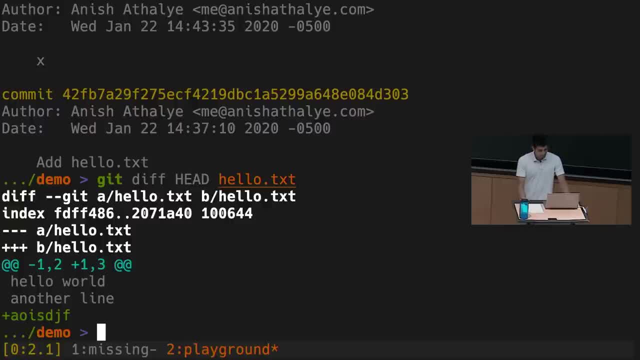 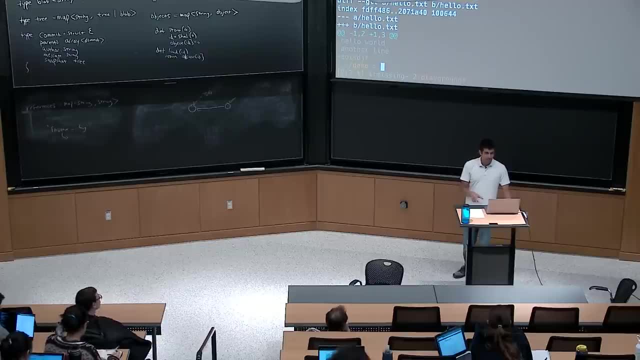 Does that make sense? I am confused. Okay, yes, So that's a good question. It's like: how can hellotxt be different than head? because head refers to where you currently are. So, to clarify, head refers to the last snapshot. 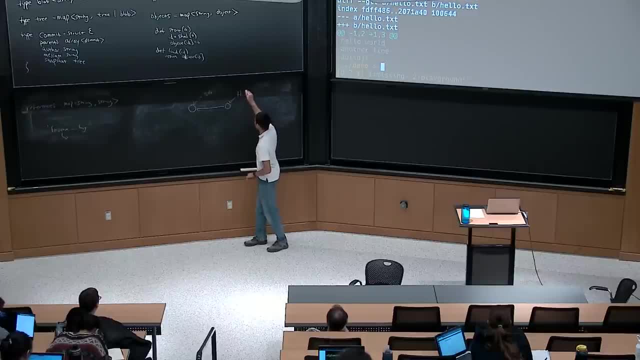 So, like in my picture here, head and master are both here And the current working directory is kind of independent of this, Like I could go and delete all the files in here. It doesn't change the history graph or the references, And so yeah. 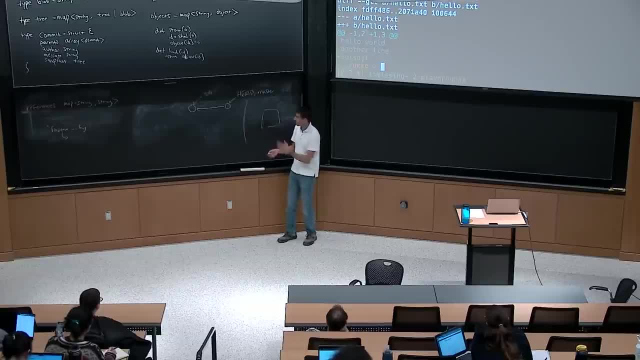 you can have differences between here and here And at a high level. this is how you work on a project Like. you make some changes here, you git add them to stage them, and then you git commit and that creates a new snapshot here. 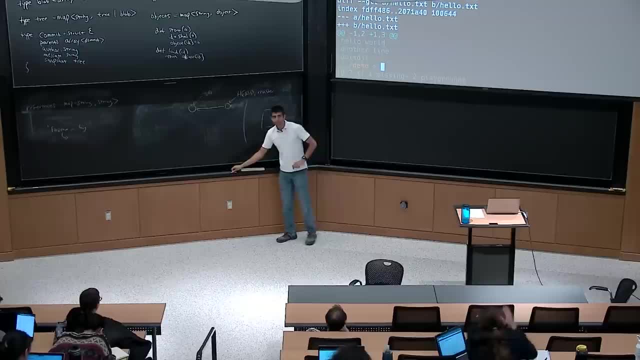 Good question. Any other questions? Yeah, So is git actually saving all of these different versions, like the way I would if I, you know, saved version one, version two, et cetera, or is it somehow just keeping track of certain references? So the question is: does git actually save all this stuff kind of in the obvious way, or is it doing something fancier? The answer is it is doing something a little bit fancier, but you can, it has an interface that lets you think of it. 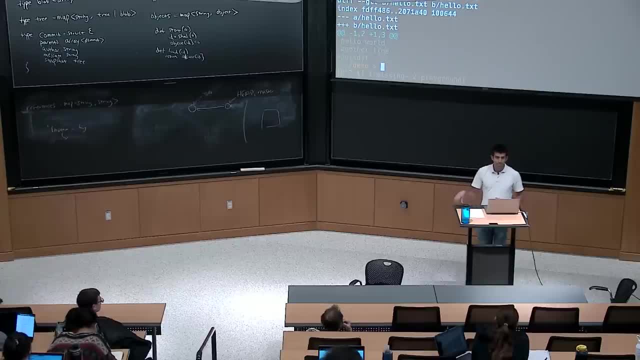 like it's stored that way In practice. git uses delta compression. It also does some other stuff, But yeah, the on disk representation is actually reasonably efficient Question. So like just with that example that you had there, say I want to compare two. 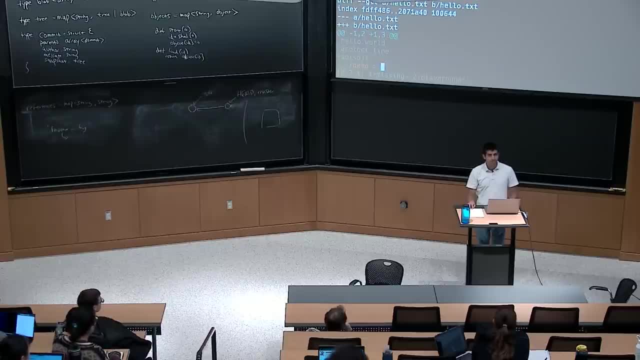 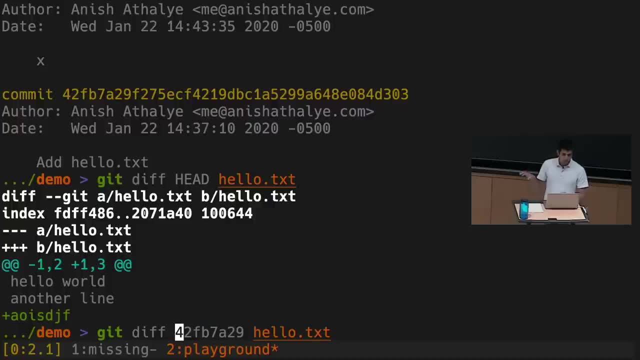 do a difference between two different things that are somewhere back up my history? Can I pick just two of any other two points that are different? Yeah, that's a good question. So the question is here. we were comparing the current working directory with a particular snapshot. 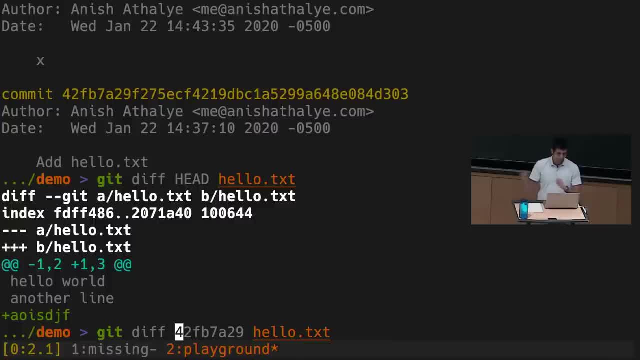 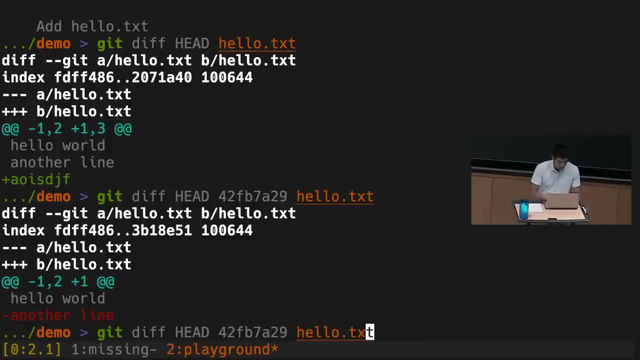 in the past. Can we compare two snapshots with each other like two different points in the history? And yeah, git diff can take yet another argument here, So I can. with I did it in the wrong order. I can compare what changed. 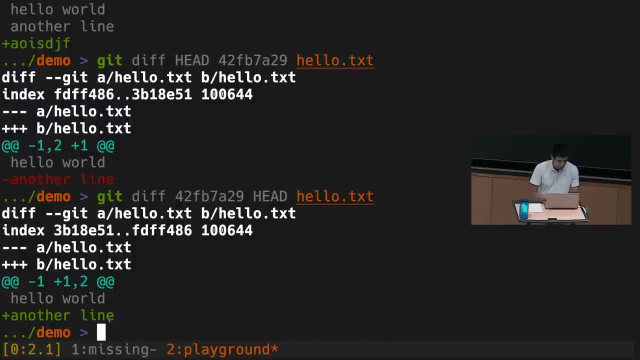 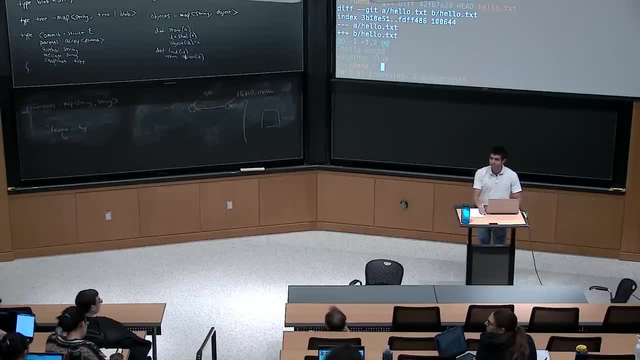 from here to head in hellotxt and it shows me that I added the second line in there. Any other questions? Yeah, So you're working on a project with people in a shared Dropbox folder. Do you want this or do you have control? 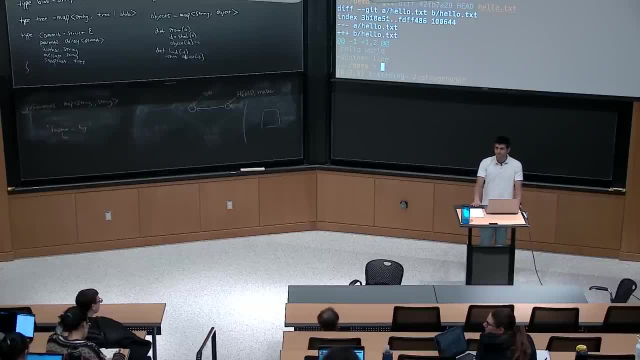 does it make sense to keep the code outside of Dropbox or is there some benefit like integrating them? Yeah, so the question is: if you're working on a shared project and you want to migrate to Git, does it make sense to turn the Dropbox folder? 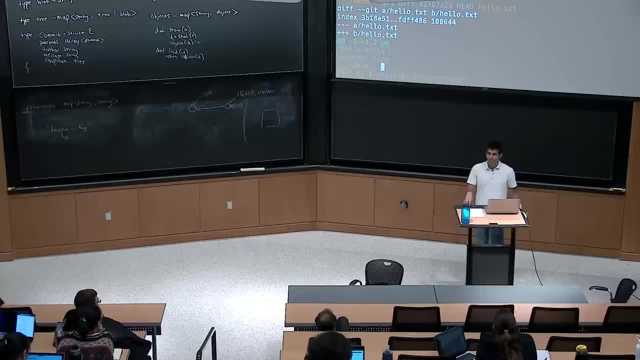 into a Git repo. Do not use Git inside Dropbox. Dropbox will corrupt your Git repo. There are good solutions to doing that. One is just use GitHub. Otherwise, talk to me after class. and there are ways of using Dropbox as a Git remote safely. 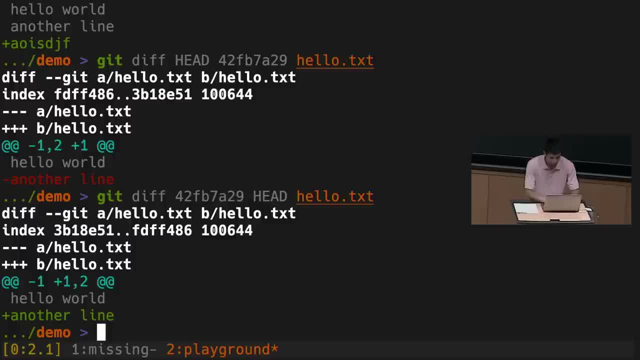 Any other questions? Next, we're going to talk about branching and merging, which is another powerful feature of Git that you almost don't use, both when working on your own projects and when collaborating with others. For this series of demos, we're going to 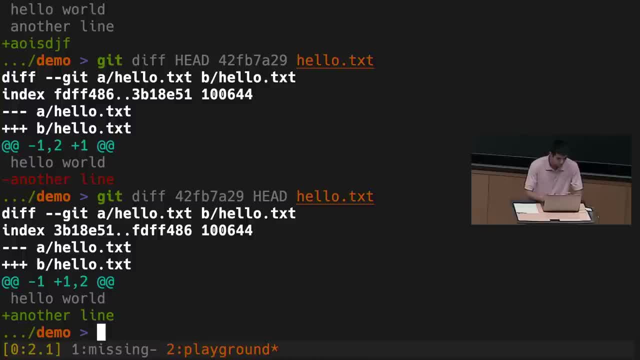 rather than work with a simple text file, actually write a simple computer program, because it'll better illustrate the concepts of branching and merging. And as we go through this demonstration, we'll keep in mind how the Git interface commands connect to the underlying data model. 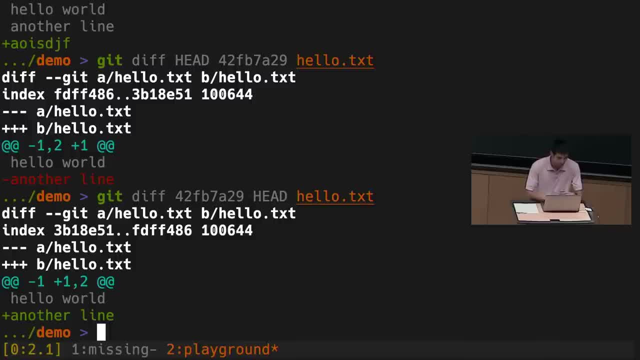 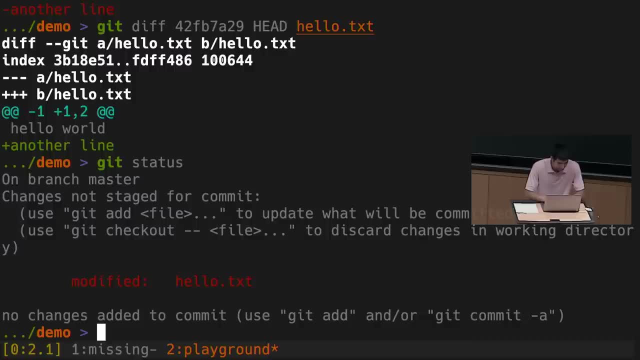 connect to objects and references and how these commands modify those two data structures. Let me do a Git status to see the current state of my repository. Here I've modified hellotxt. I actually don't really care about this modification anymore. This is just. 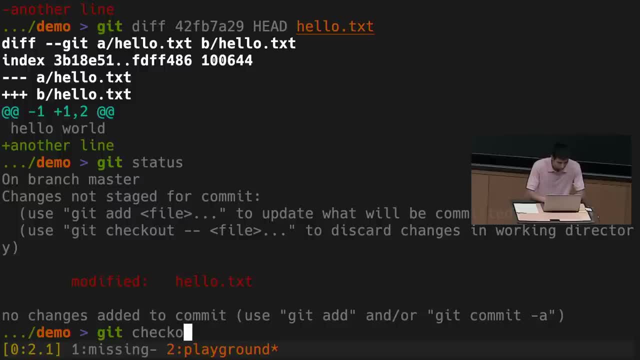 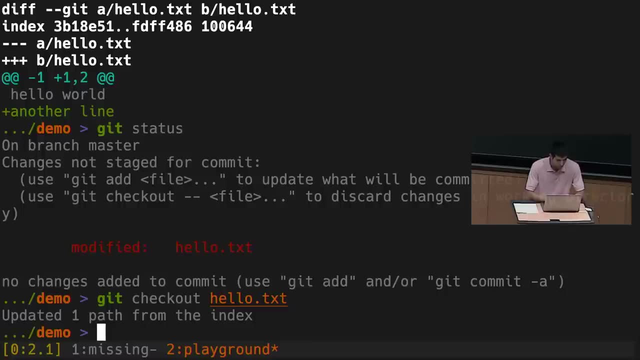 some random file If I do git checkout, hellotxt. this is another different use of the checkout command, which basically throws away the changes that I've made in the working directory and sets the contents of hellotxt back to the way it was in the snapshot. 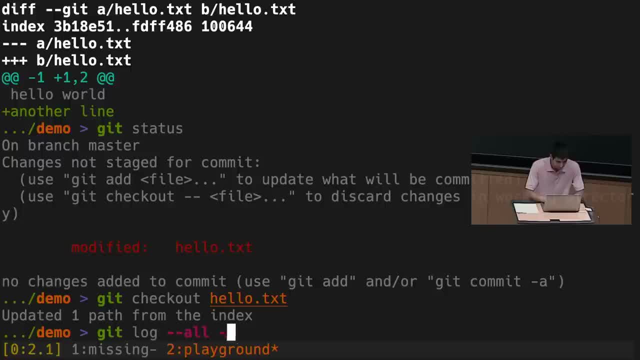 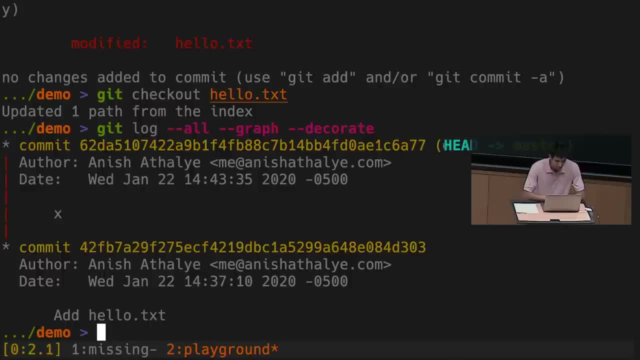 that head points to. If I look at git log: dash, dash, all dash, dash graph, dash, dash, dash, then I start dead decorating. it will show me that here I've added the initial hellotxt and I've added that single line here. and so now. 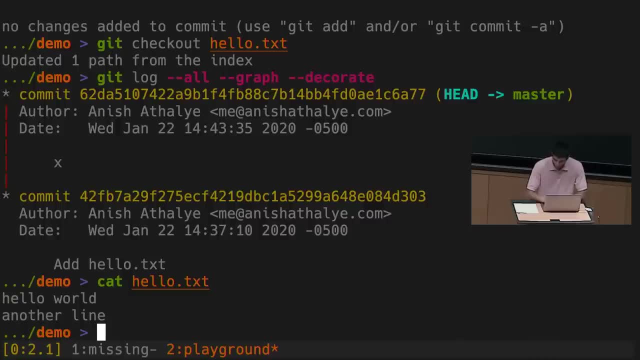 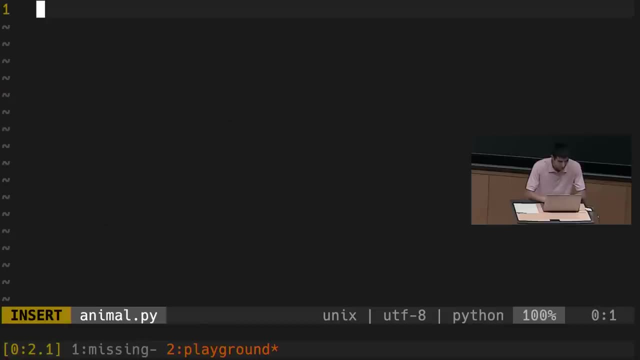 hellotxt doesn't have that third line I've added. it just has the original two. Next, I'm going to write a very simple program. I'll call this program animalpy and let me just go ahead and write a program. that's a principle. 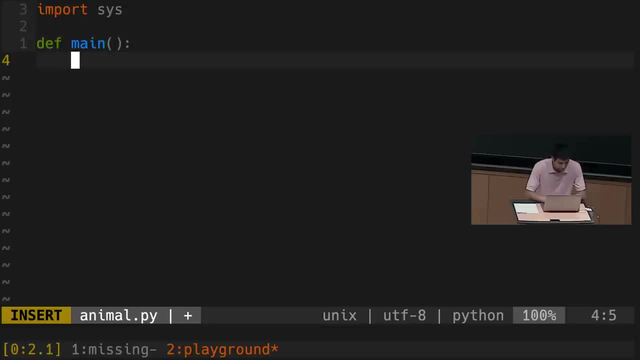 output when I run it. Let's see Intent and hellotxt. So when I run this program it runs main, main calls default, and then let me go ahead and define default, and default is just going to print hello. so this is a program that 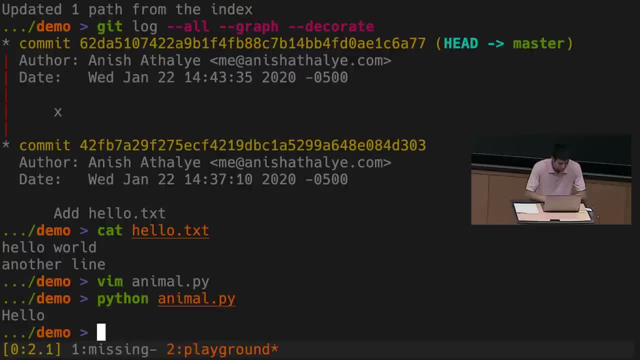 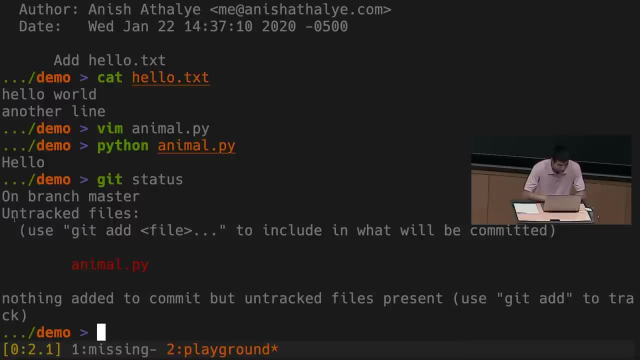 greets its user, and so if I run animalpy I'll see that it just prints hello. so that'll be our starting point. If I do a get status, it shows me that animalpy is an untracked file To begin with. I want this to be part of the snapshot, so I'm going to get add animalpy. 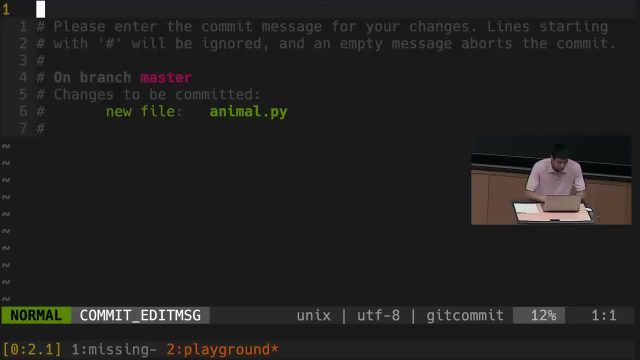 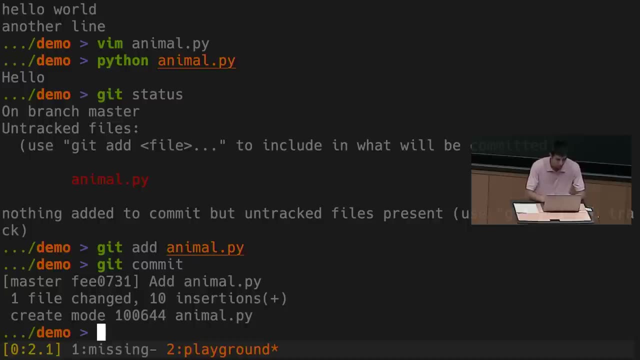 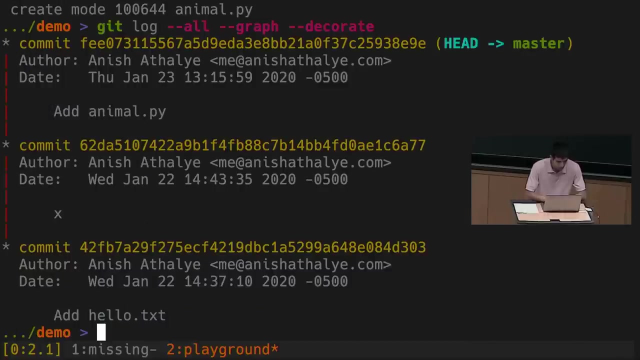 to add it to the staging area and then do a get commit. Here I'm going to write yet another useless commit message. Don't actually write commit messages like this in real projects, but for now this is fine. So now I have this basic animalpy and if I look at my get history now I have this: 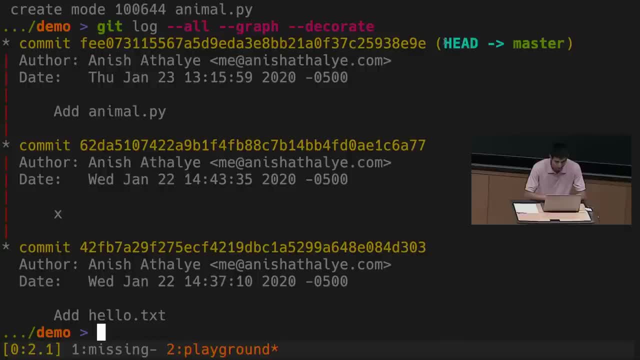 latest snapshot, This is the commit hash and this is where the master branch is pointing. Now we're actually going to demonstrate how to use get branches to have parallel lines of development. The get branch command or the branch subcommand is used to access functionality related to. 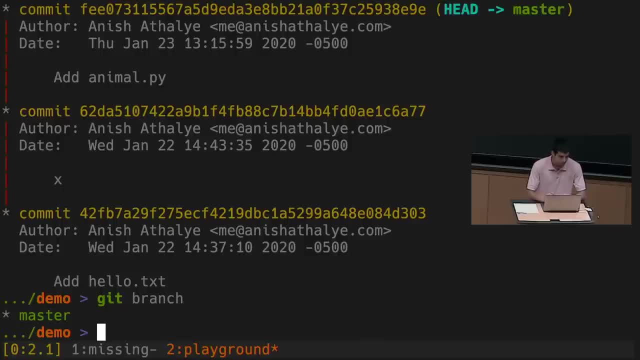 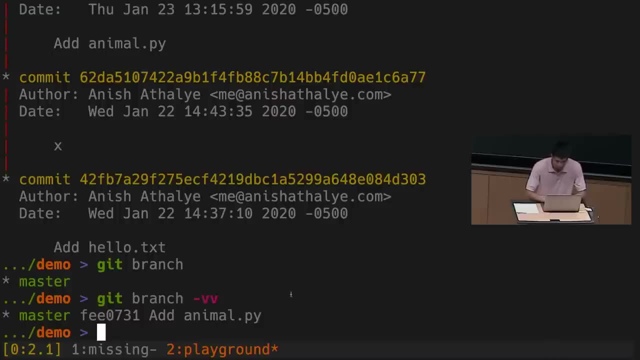 branching Just running. get branch by itself lists all the branches that are present in the local repository. It can also take an extra argument, dash vv to be extra verbose and print some extra information. If we do get branch, we're going to get the branch and we're going to get the branch. 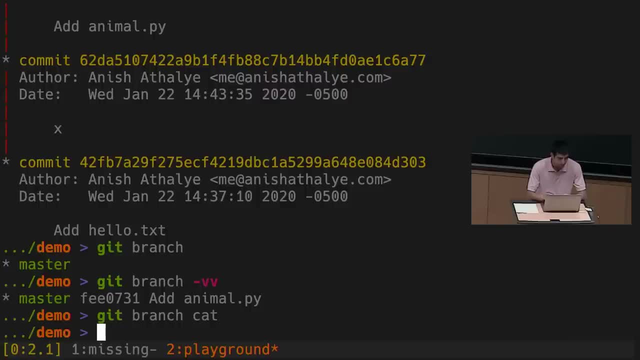 and then specify the name for a new branch, Get will create a new branch, which is just a reference that points to the same place where we're currently looking. So now there's a new reference called cat. A reference in this case is the same as branch. 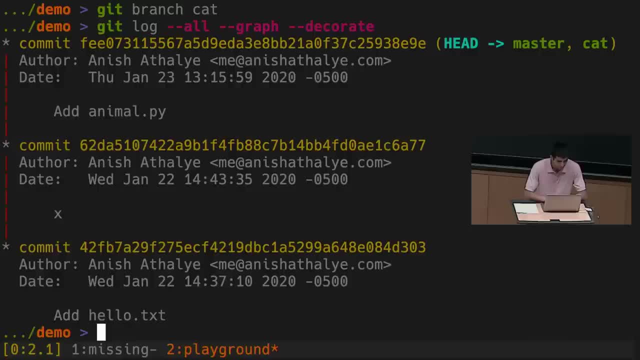 There's a new branch called cat, which points to wherever head was pointing. If I look at the get log again, I'll see that here head points to master. master is over here and this is also where the cat branch is. So now I have two branches, two references that resolve to the same commit. 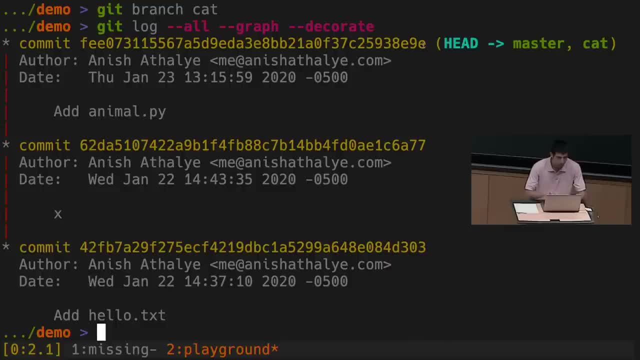 Get is actually aware of not only which snapshot in the history you're currently looking at- so head points to this commit- but it's also aware of head kind of being associated with a branch. So here head is associated with master and it's the case that if I create a new snapshot, 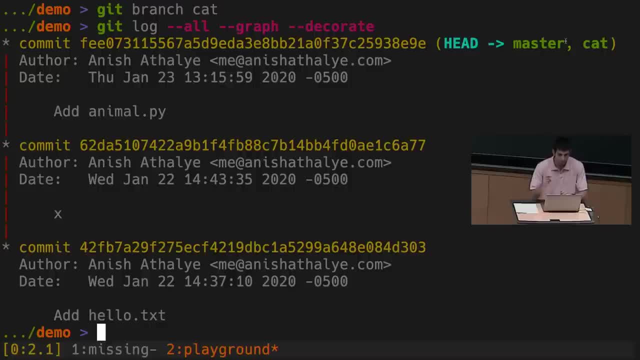 if I type get commit at this point, the next snapshot will be created and then master will point to that new snapshot. Master will be updated along with head. If I do get checkout cat, what this does is it switches to the branch cat. 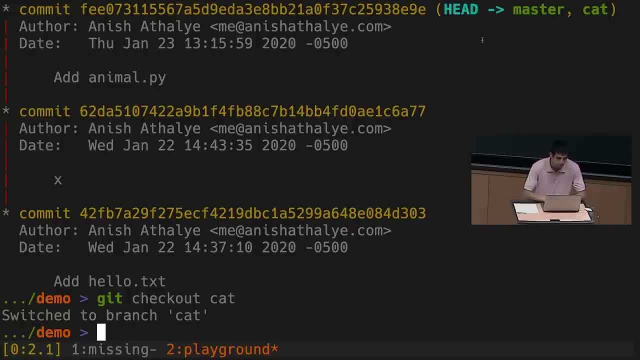 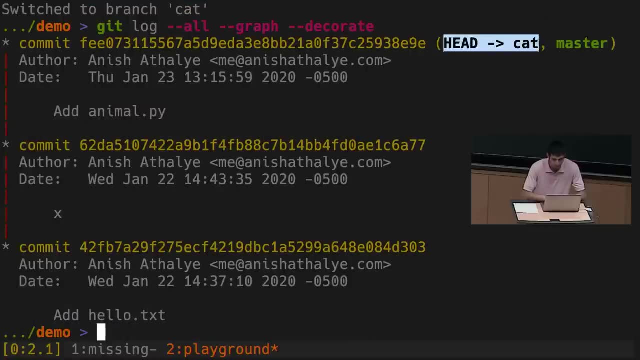 It replaces the contents of the working directory with whatever cat's pointing to, which, in this case, is the same as the contents before. but now, if I look at the get log again, now I have head pointed to cat instead of master, and then master also points to the same place. 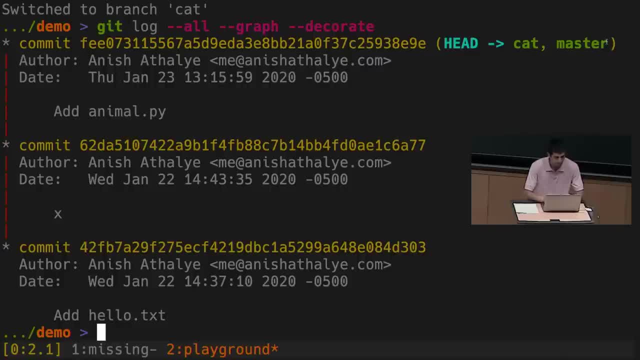 the same underlying commit. And now, at this point, if I make changes to my current working directory and make a new commit, the cat branch, the cat pointer, will be updated to point to the new commit, whereas master will continue pointing wherever it pointed before. 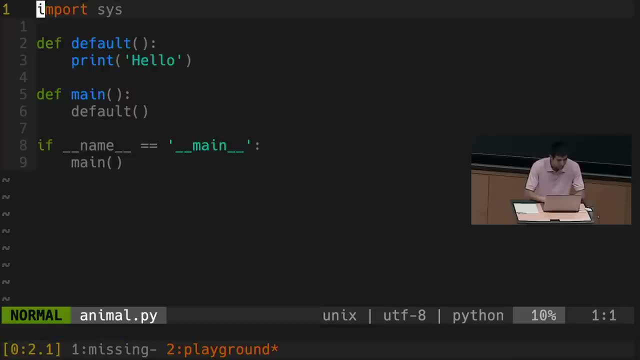 So let me go ahead. I'm going to go ahead and modify animalpy to add some cat-related functionality. So I'm going to say that if sysargv1 is cat, then run the cat function, otherwise run the default function. and then let me go ahead and define the cat function. 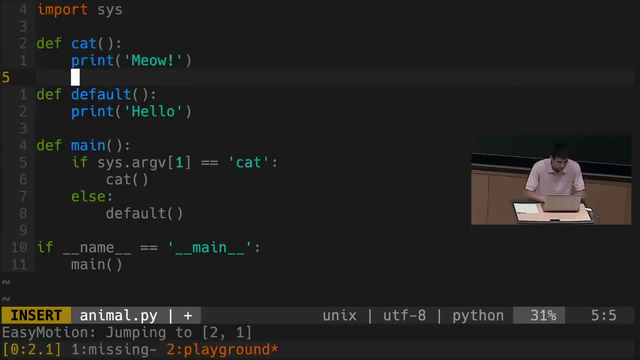 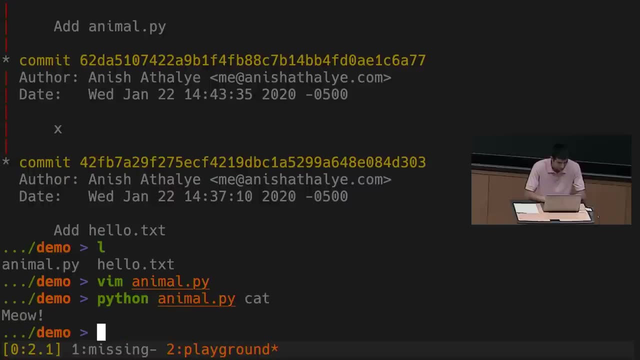 So cats don't say hello, they meow. so cat prints meow Straightforward enough. So now if I run animalpy and give it the cat argument, it says meow. If I give it some other argument, it defaults back to the hello. 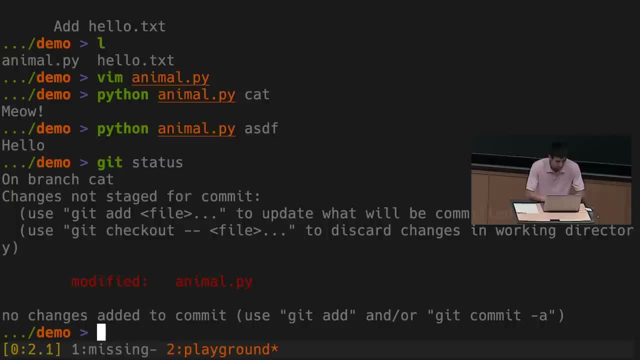 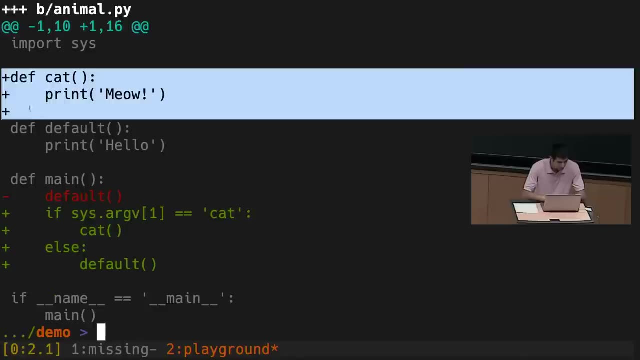 All right. so a simple change I made. If I do a get status, it says that animalpy has been modified. If I run get diff, it'll show me what's changed since the last commit. So here I've added this cat function highlighted in green, and then also changed the main function. 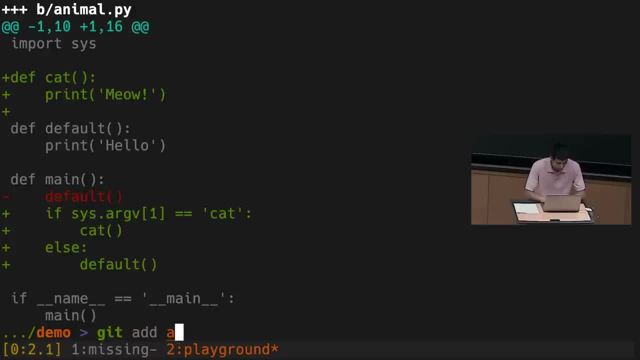 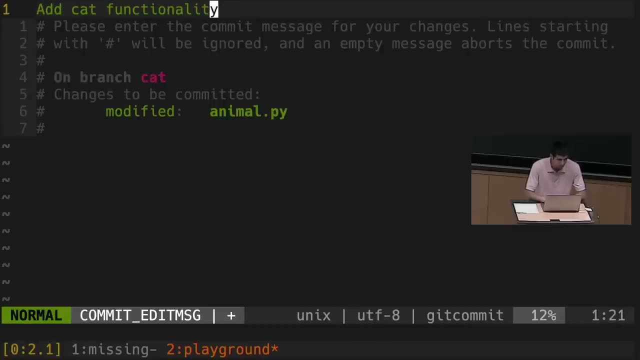 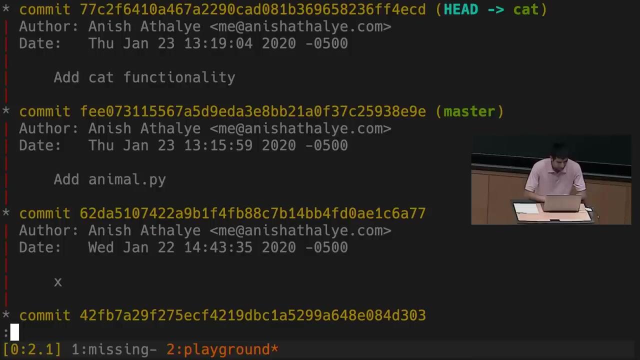 a little bit Now here. if I do get add animalpy, get commit, I'm going to actually write a slightly more useful commit message. this time I'm going to add cat functionality. And now if I look at the get log I see a little more stuff. 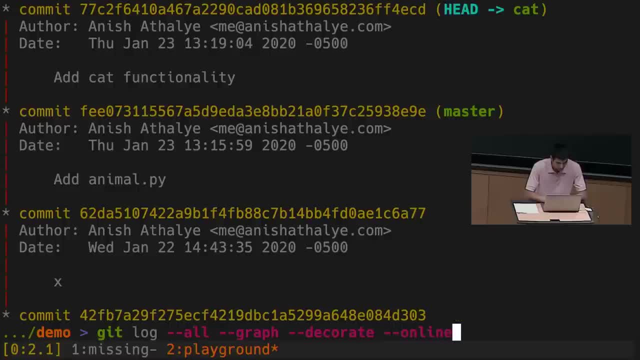 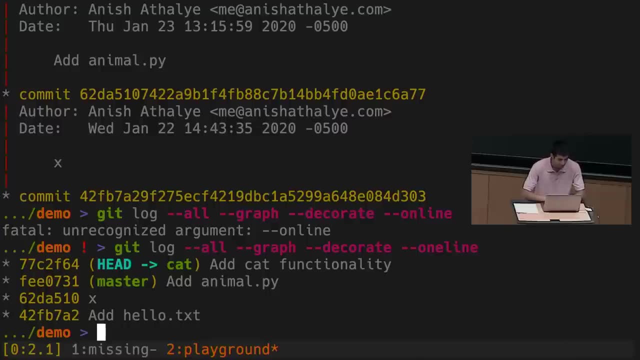 I'm going to show you one more argument to this get log command. There's an argument, dash, dash, one line, one line spelled correctly, which shows a more compact representation of the graph. So this will be a more useful thing to use, because we're super zoomed into the screen. 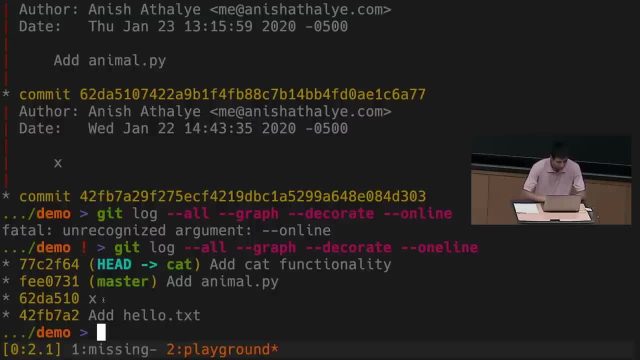 and there isn't that much space to show a long commit history. So here we see the sequence of commits. This is still linear And we have master still pointing wherever it pointed before, where we just had the basic underlying animalpy functionality. But now we have this cat branch which adds the cat functionality. 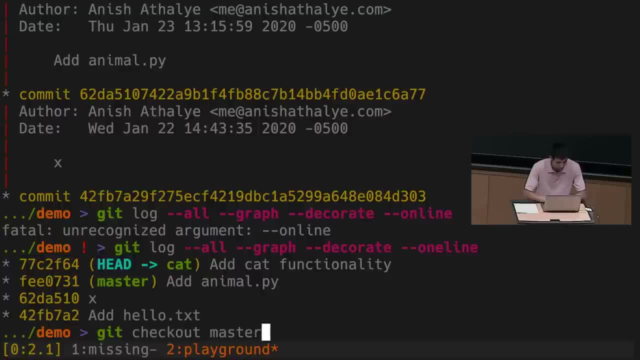 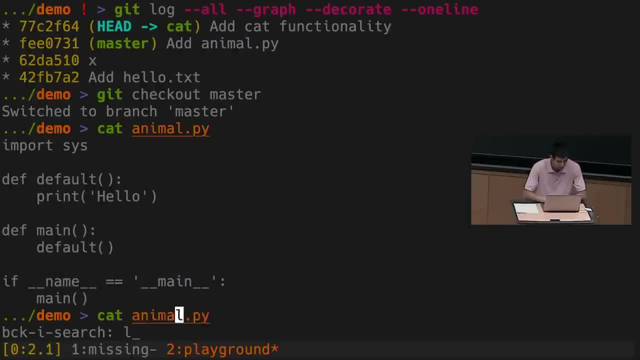 We could, for example, get checkout master to go back to the master branch. And then here, if we look at animalpy, it doesn't have the cat functionality anymore. And if we look at the get log, we'll see that head is pointing to master. 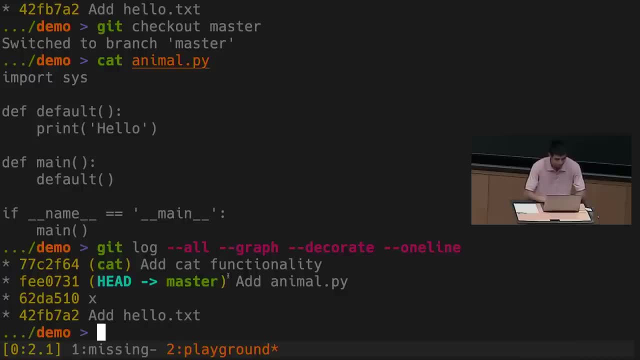 So this way we can jump back and forth between parallel lines of development. So now that we have the cat functionality, suppose that we want to work on adding dog functionality in parallel And suppose that in this case, like the cat, functionality is under development. 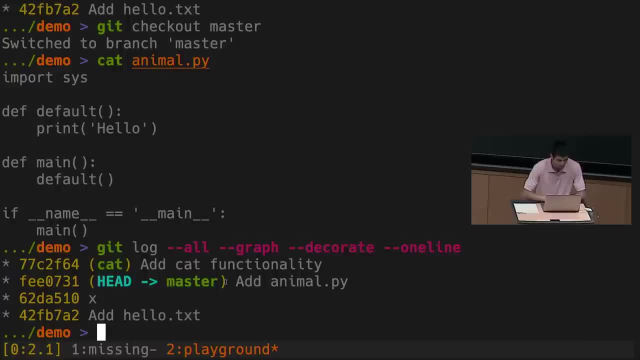 Or maybe somebody else is working on it. So we just want to start from the base- master commit and build the dog functionality starting from there. So now, what do I want to do? I want to create a new branch dog for adding the dog-related functionality. 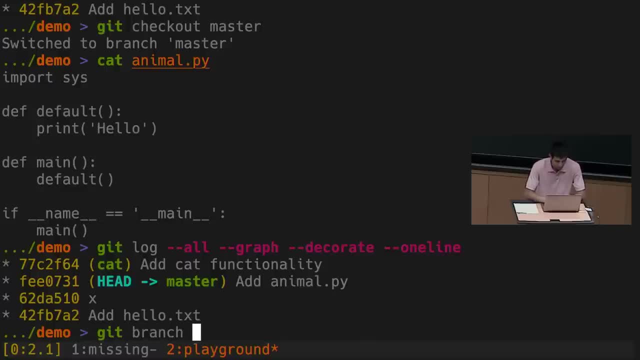 And I'll eventually merge it in later, So I can use the get branch dog command, followed by the get checkout dog command, to create a new dog branch and then check it out. There's actually a short form for this: get checkout dash b dog. 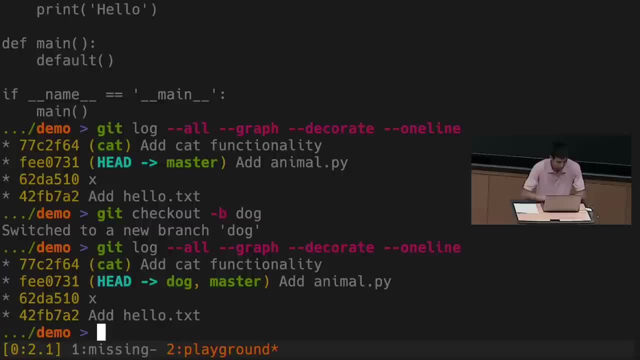 So this does get branch dog, get checkout dog. Now, if I look at my graph, I have cat where it was before, master where it was before, But now head, instead of pointing to master as it did before, now head points to this newly. 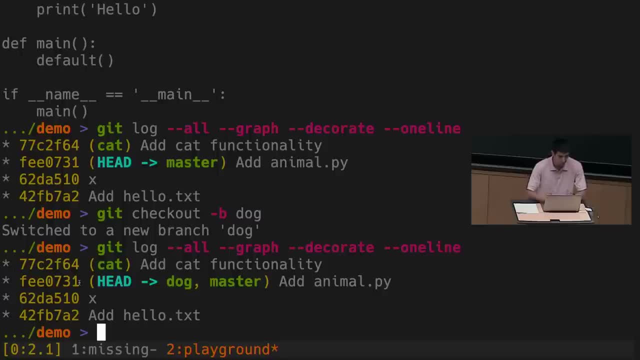 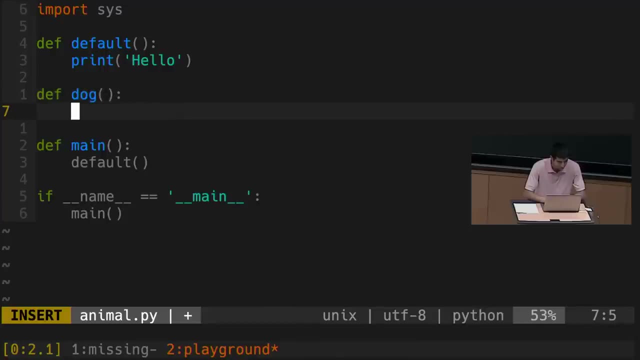 created dog reference, which is also at the same commit, so at this base commit, And now I'll go ahead and add my dog functionality. So let me go and define my dog function. Dogs don't say hello, they say woof. 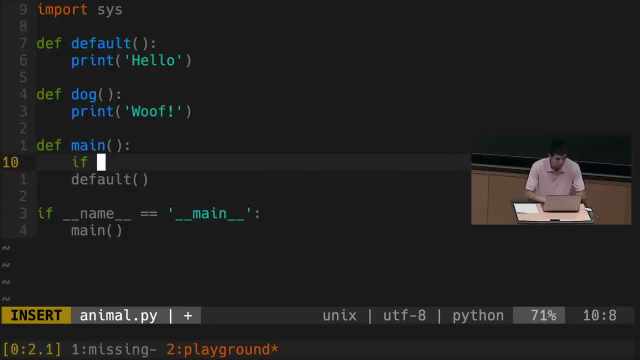 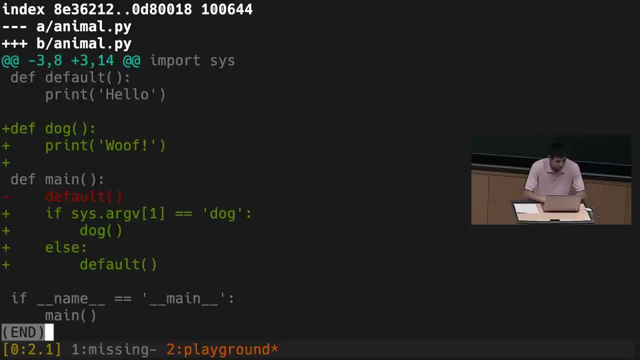 And then I'll add some similar functionality here to decide whether to run default or dog. So if the first Argument is dog, then I want to run the dog function. Otherwise I want to run the default function. So here's what I've changed. with respect to the base commit wherever master is pointing. 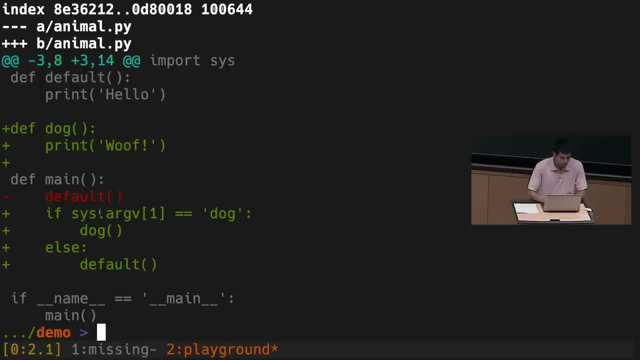 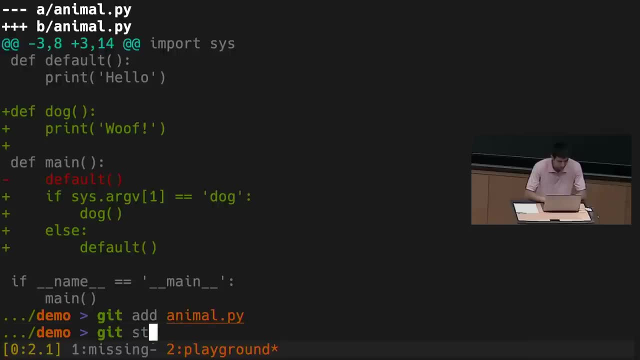 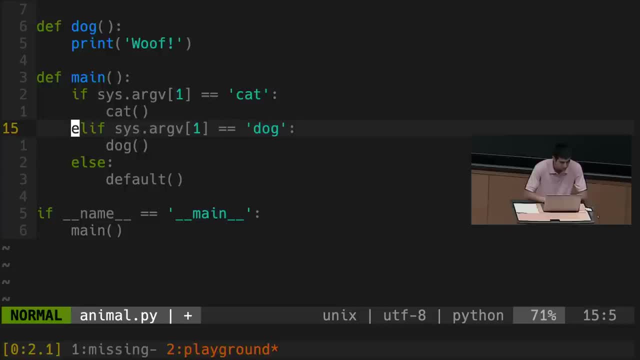 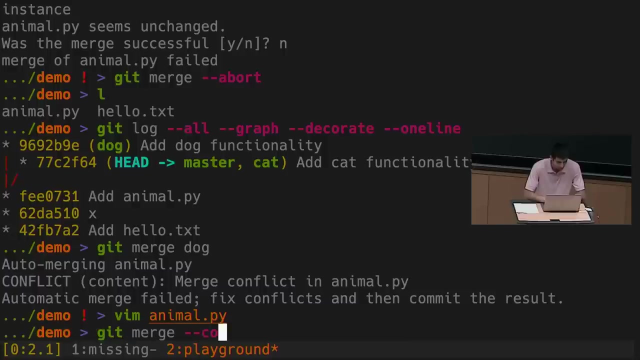 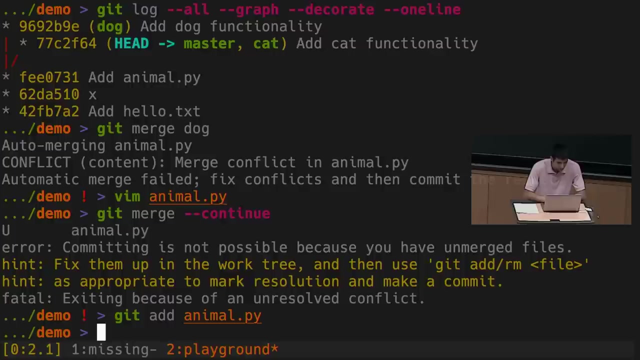 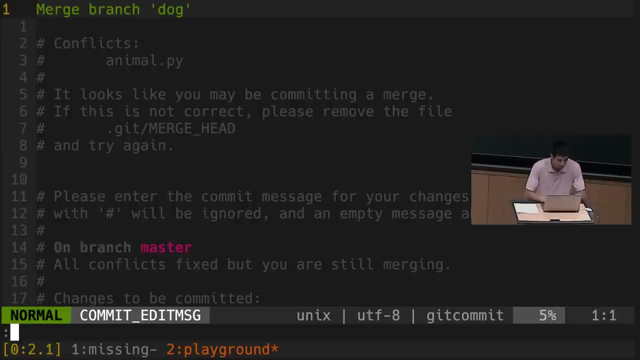 If I do get status, I'll see that this change will be committed when I get the dog function. If I do get status, I'll see that this change will be committed when I get the dog function up an editor and we can give a commit message for this new commit that we're about to create. 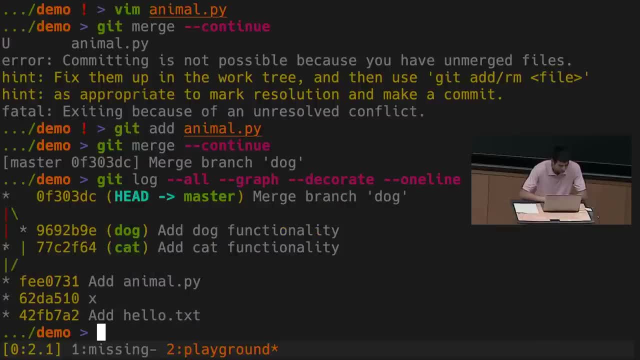 And now, if we look at the git history, we have the single commit that represents our merge commit that we just made, which merges in the dog functionality, and here this has as parents both the dog commit and the cat commit. So both these branches appear in our history from this. 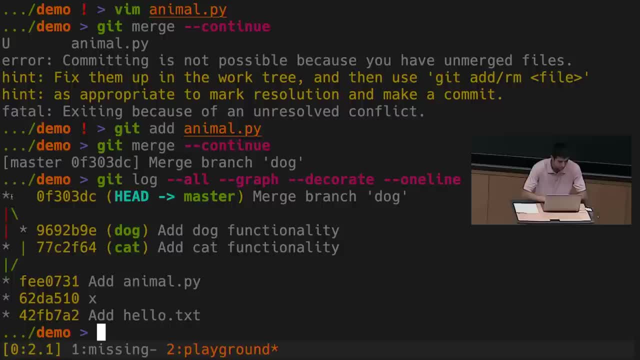 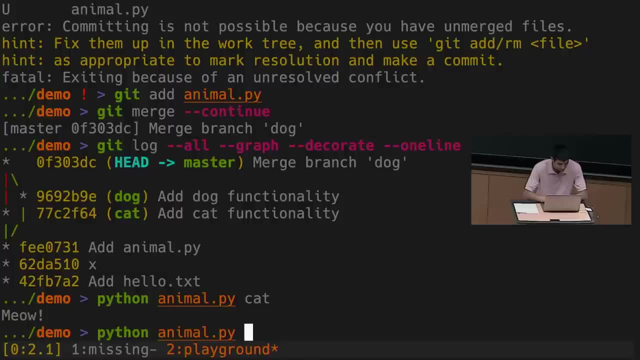 point backwards, and this current commit that we're on incorporates the functionality from both of these branches. So if we run animalpy with cat, it does the cat thing, if we run it with dog, it does the dog thing, and if we run it with anything else, it falls back to the default implementation. 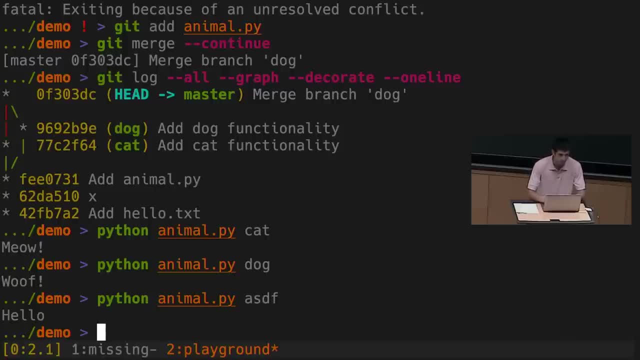 So this is a demonstration of how you branch in git to do development on different things in parallel, and then how you can use the merge command in git to resolve those different branches and combine them together into a single snapshot that includes all the functionality that was developed in parallel with each other. 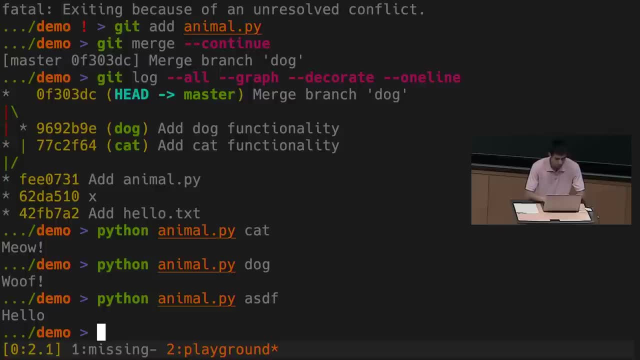 Then one thing that can happen when you're doing git branching and merging is you run into merge conflicts and these conflicts show up as conflict markers and text files. you can manually resolve them, and git also has some tools that can help with this, though these tools are kind of advanced. 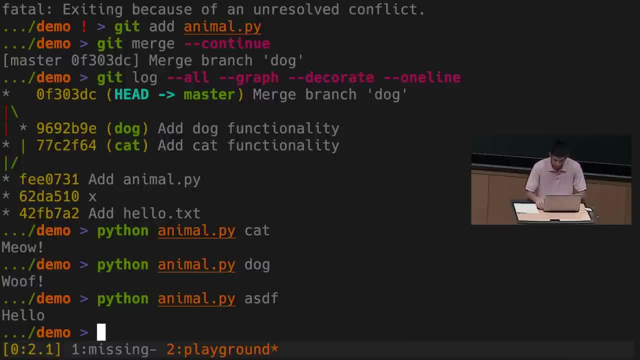 and we'll only refer to them in the lecture notes and not actually demonstrate them for you. So that's git branching and merging. Any questions? No Great. So, moving on to the next topic of this lecture, we will talk about git remotes. So this is basically how you collaborate with other people. 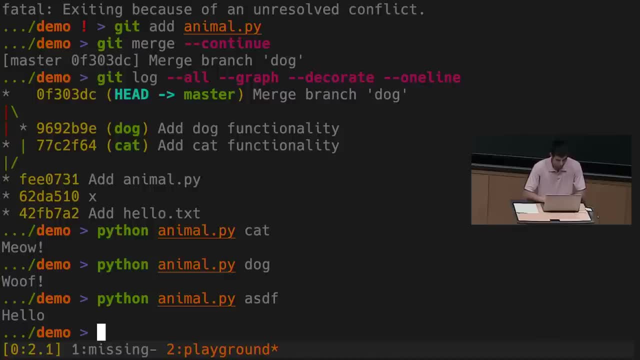 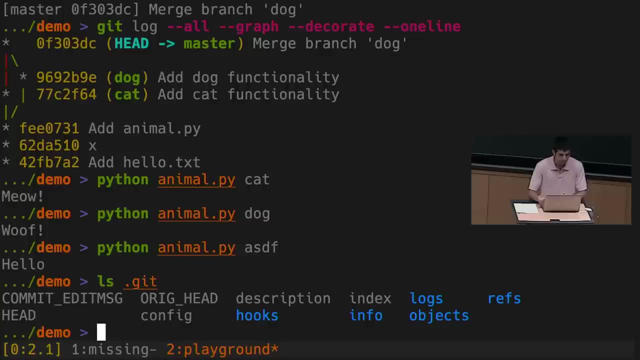 using git, A git repository. the stuff contained in this git folder represents kind of an entire copy of the history. It has the objects and the references and contains all the previous snapshots. and the way you collaborate with other people using git is that other people can also have. 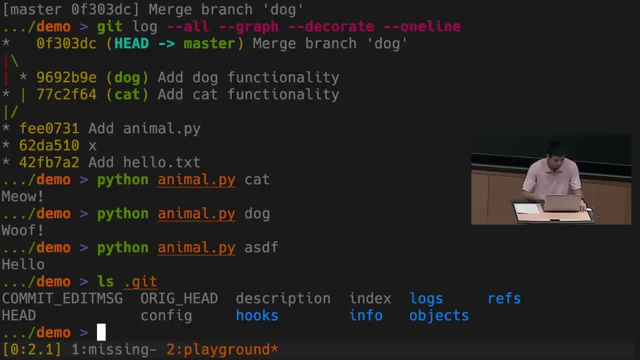 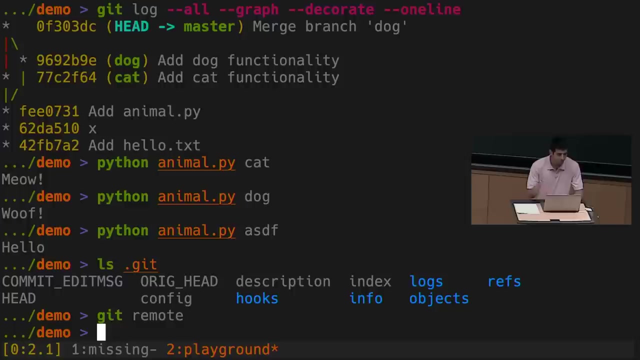 copies of the entire git repository. and then your git copy, your local instantiation of the repository, can be aware of the existence of other clones of the same repository, and this is a concept known as remotes. So the git remote command will list all the remotes. 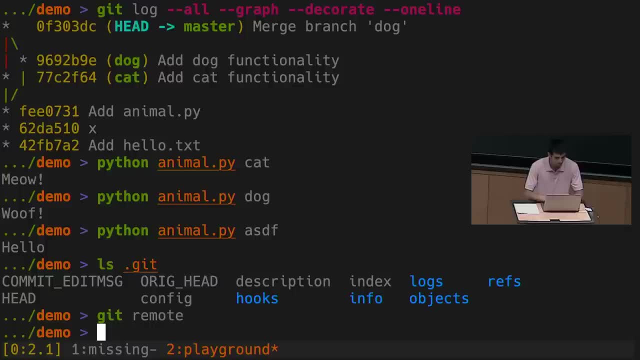 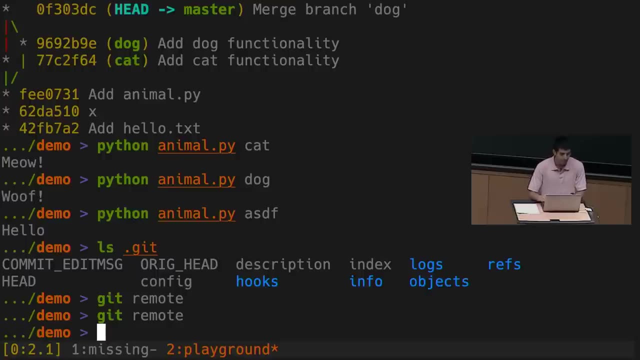 that git is aware of for the current repository, and in our case, with this repository right here, this command git remote just doesn't print anything because we haven't configured any remotes. Git is only aware of the single local copy of the repository that we're working with here. 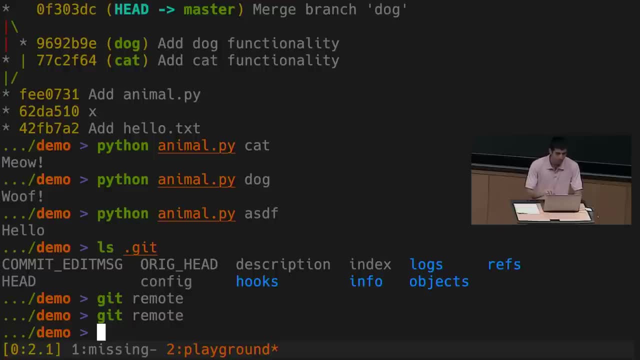 but in practice, if you're collaborating with other people, your git might be aware of the copy of the code that is on github. and then there's a set of commands to send changes from your local copy of the repository to a remote that your git is aware of, So sending stuff from your computer to github, for example. 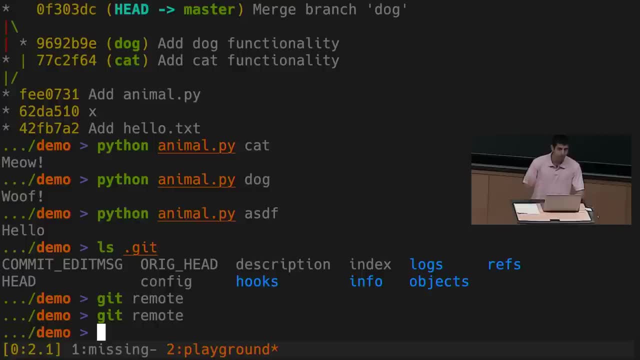 and there's another set of commands for fetching changes made in a local repository, to get changes from github into your own local copy. In this demonstration here we actually won't go and configure a github account and log in and create a new repository on there. You can. 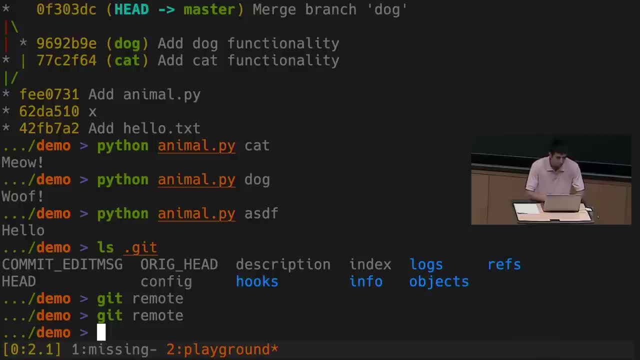 find other tutorials for doing that. We'll actually just use a separate folder on the same computer and treat it like a git remote. So let me- I'm in the demo folder here. let me go up one directory. I have a directory called playground that has this demo folder. 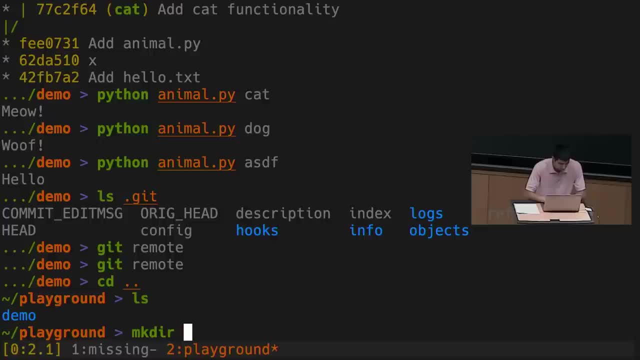 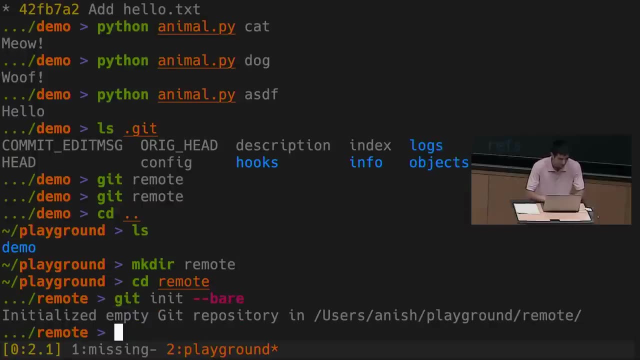 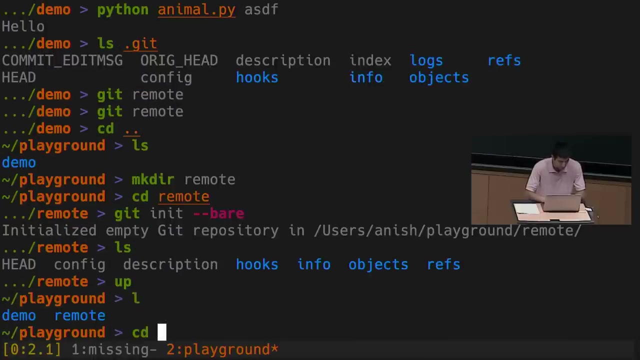 and I'll go ahead and create a new directory in here and I'll call it remote and then do git init dash, dash bear in here. This is a command that you'll probably never need to use in regular usage, but now what I've done is made remote into a folder that's appropriate to use as a git remote. 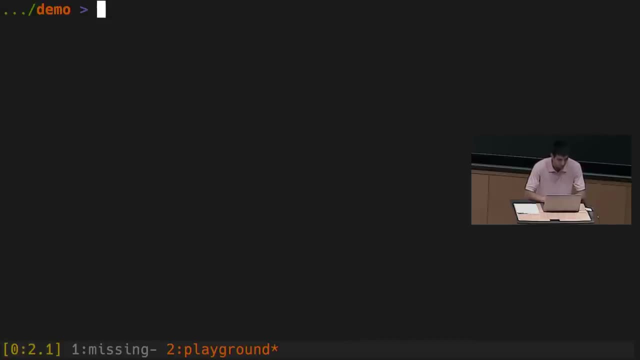 So now, going back into my demo folder here, my main repository, I can do git remote to list the remotes. There's nothing yet, but I can use the git remote add functionality to make my local repository aware of the existence of a remote. So I can do git remote add and then the format for this is that remotes have names. 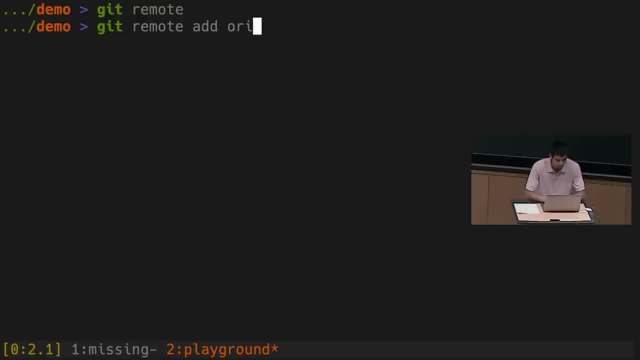 and then they have a url. So in this case I'll use the name origin- that's often used by convention- as the name of the remote. if you're only using one, And then for the url, normally this will be like a github url or. 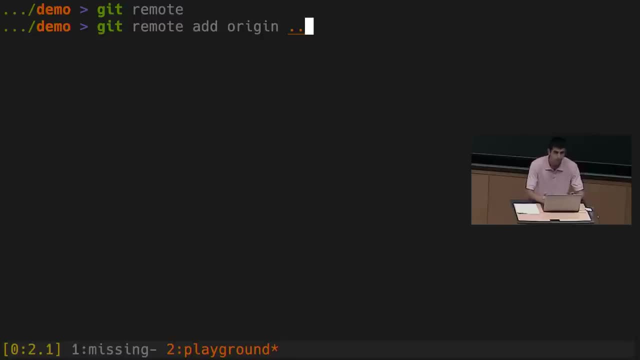 something like that, or bitbucket url or git lab url if you're using an online repository hosting service, But in this case it's just a path to a folder on my local machine. There's a folder in the parent directory called remote that will act as the git remote for this repository. 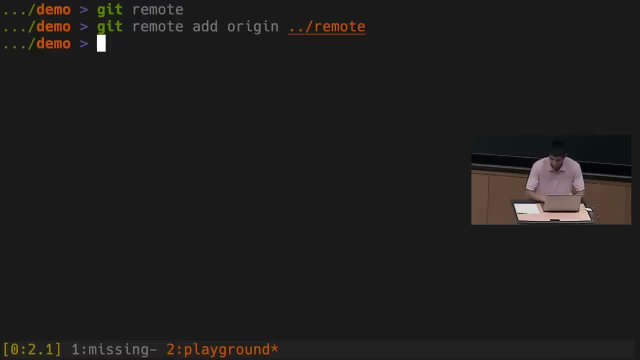 So now, once I've done that, there's a set of commands for for interacting with this remote. One command that's useful is the git push command. This command can send the changes from your computer to the remote, And the format for this command is that. 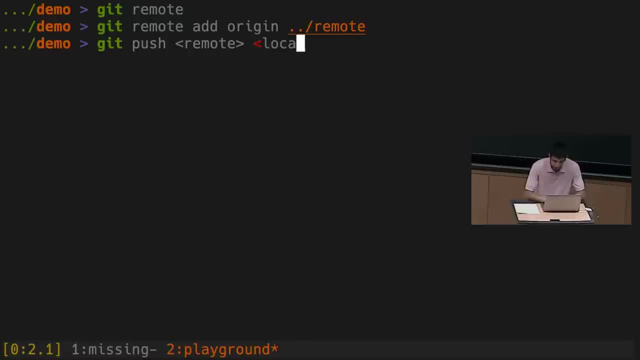 git push takes in the name of a remote and then it takes in a local branch name, colon, a remote branch name, And what it does is it creates a new branch or updates a branch on the remote with the name specified here and sets it to the contents of the branch specified here. 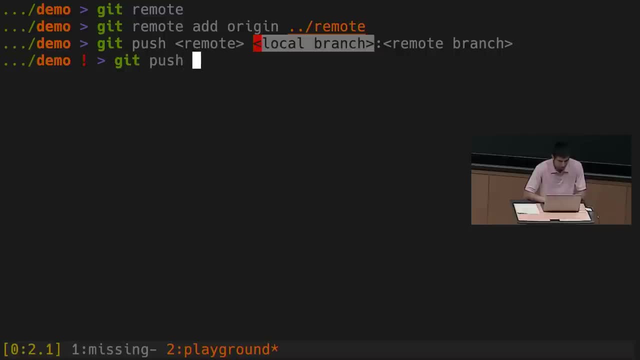 So a concrete use of this might look like git push. I have only one remote called origin. And then what should I push? Let me look at my history graph. I have a bunch of things I could push. Let me git push to origin, the master branch. 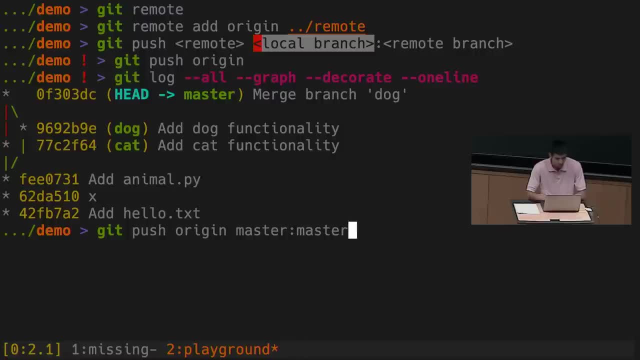 from my local machine, colon master. So I want to create a branch on the remote machine with the name master. that is going to be the same as the master branch on my local machine. So let me go ahead and run that command. It prints out some stuff and it says: 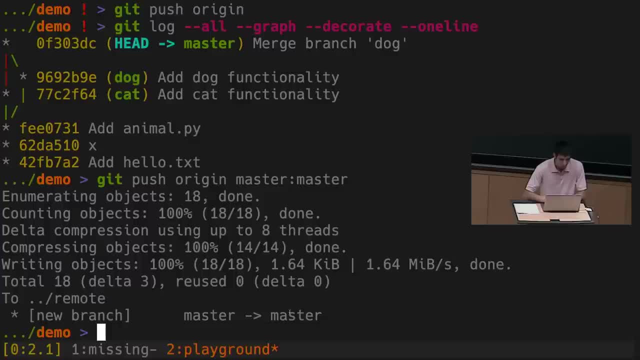 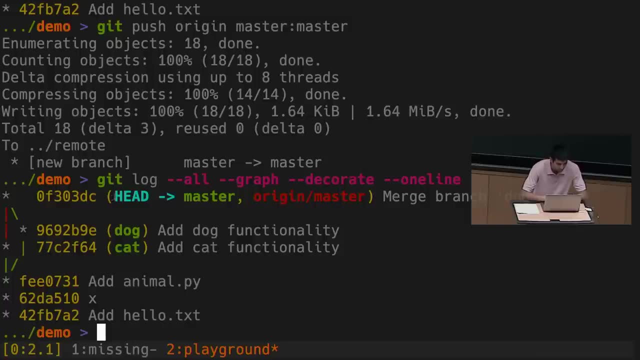 on the remote. I created a new branch. Remote master points to the same branch as master on my local machine And now if I do a git log it shows me so. in blue is head, where I currently am. In green are all the branches in my local git repository. 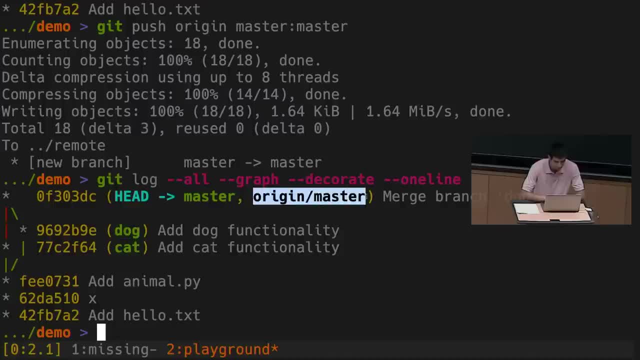 And now we see one new color here that we hadn't seen before. So in red, git shows references that are present on the remotes that my local copy is aware of. So on the remote origin, there's also a branch that happens to have the name master. that. 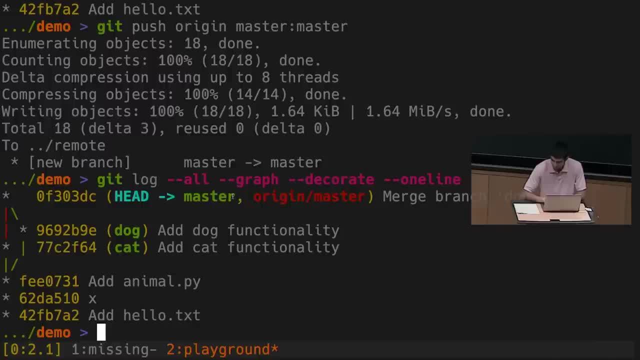 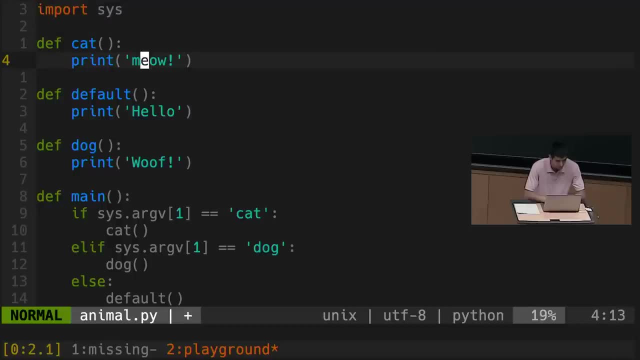 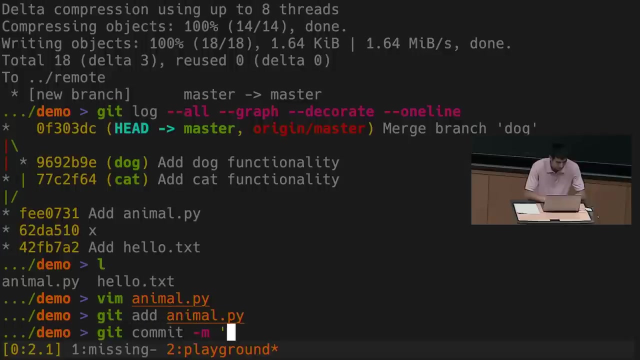 points to the same place as my local branch master points. And so now if I make updates to my local copy, like suppose here I go in and change the capitalization of these things and then git add animalpy, git commit- Here's a short form for commit with a message. 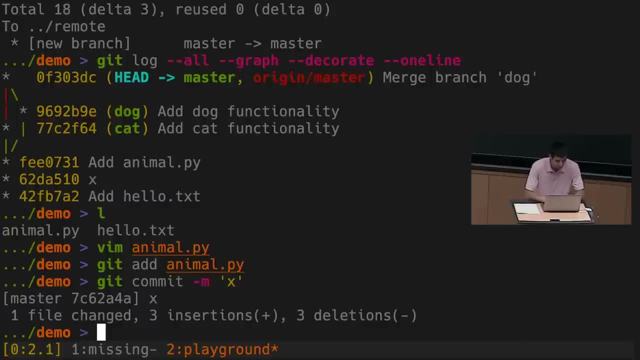 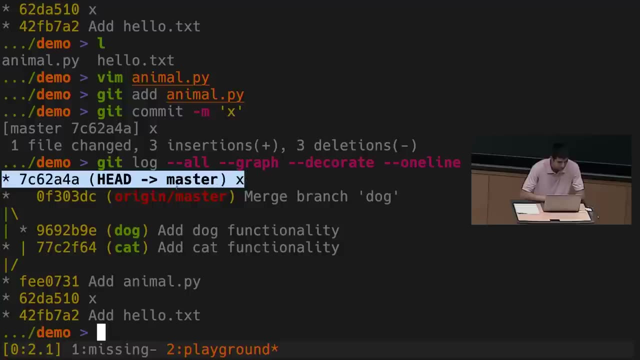 so it doesn't pop up the editor, I'll give it a lame commit message. And now, if I look at the git graph now I see that I've created this new snapshot Here that has this lower casing stuff in it, But origin master is still back here. 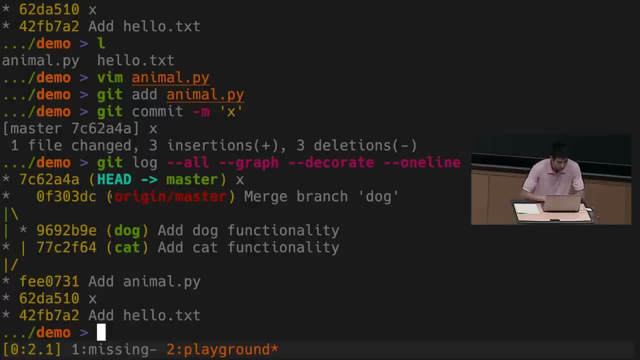 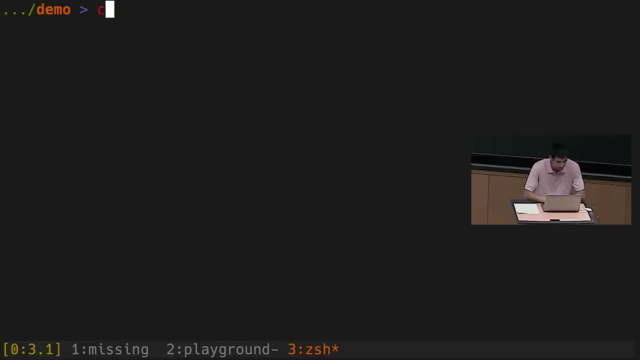 So if somebody else looks at the remote, they will only see the changes up to here And we can actually demonstrate this functionality. So let me go ahead and open up a new tab here and go into my playground directory. The git clone command is a command. 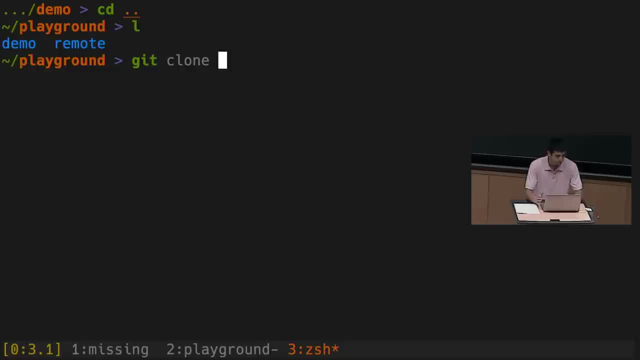 that somebody can use to start from some copy repository somewhere and make their own local copy. So this is often a command to use when starting out with a git repo, Like there might be something available on GitHub and you want to copy it all on your machine. 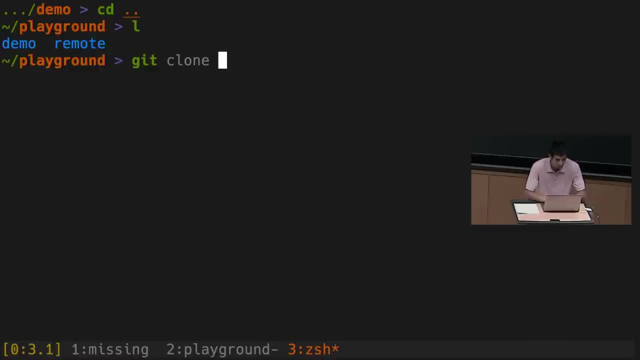 in order to look at it or start doing development, And so the format for git clone is that it takes in a URL and then it takes in a name for a folder for where to clone it. So in our case, here we're just going. 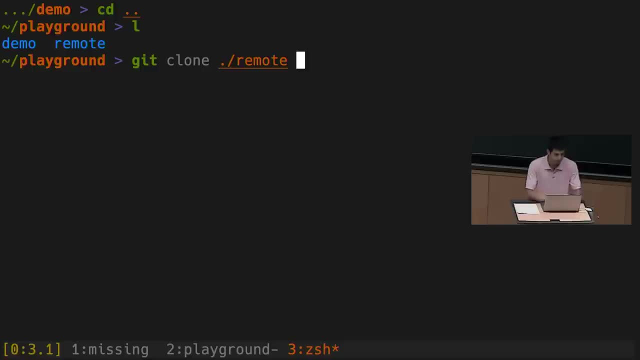 to clone from this remote directory. We're pretending that this remote folder is actually a remote machine And then we'll clone it into the folder called demo2.. So cloning into demo2, done, And I'm going to cd into that directory. 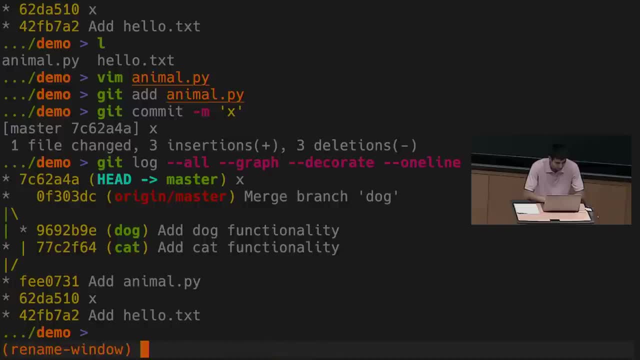 And then now here I'm going to rename these tabs. at the bottom We'll say this one's machine1, and this one's machine2.. So you can think of these as two different people on different machines with their own copy of the repository. 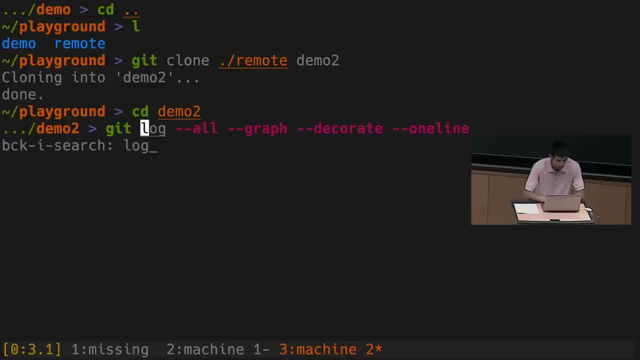 and they're both interacting with the single remote. So if I do my git log command that I've been doing on machine1,, I see on machine2, I see this portion of the history, So master on machine2.. And I'm going to cd into that directory and then now here: 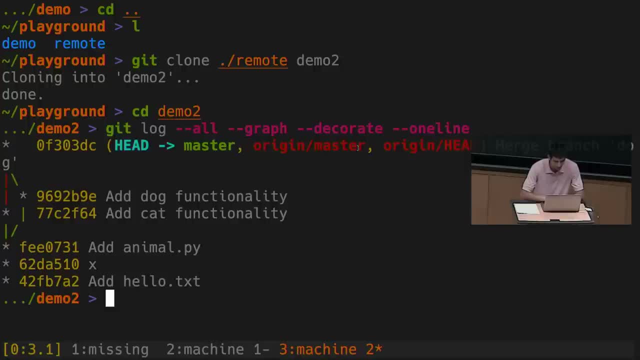 I'm going to rename these tabs at the bottom And then I'm going to cd into that directory. So you can see, here on machine2, is pointing to the same place as origin master And it says merge branch dog. So if I look at animalpy here, it 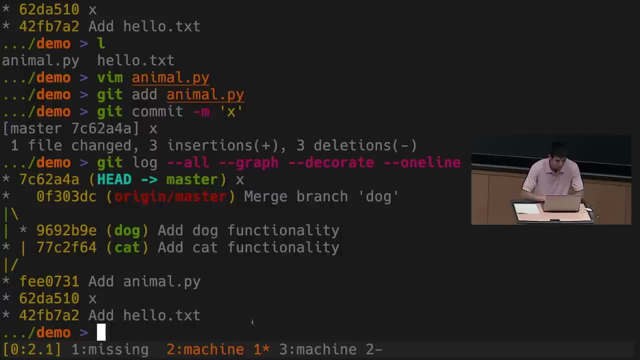 doesn't have the changes that I made on machine2, even though they're- or sorry- on machine1, where I have this new commit that is only present on this machine but not on the remote and not on machine2.. So if I want to fix that, if I want, 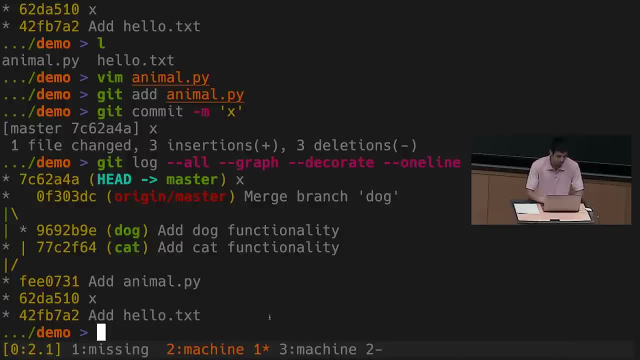 to send these changes up to the remote like- think of it as sending it up to GitHub or up to the machine that's holding or maintaining the source code. I can use the git push command again- Git push, origin, master, colon, master, And this will work. but this is kind of annoying. 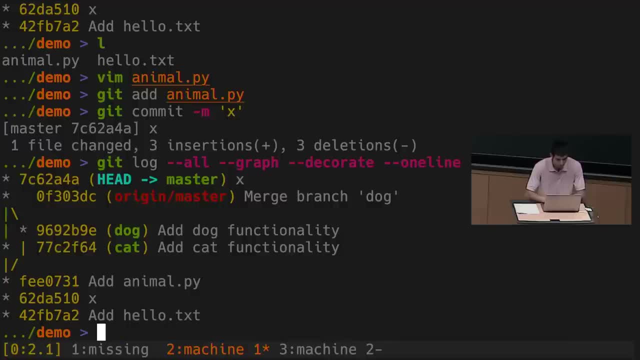 to type every time you want to do this, Like this is a really common operation. So git has a way of making this a little bit simpler. It has a way of maintaining relationships between branches on your own local machine and branches on remote machines. 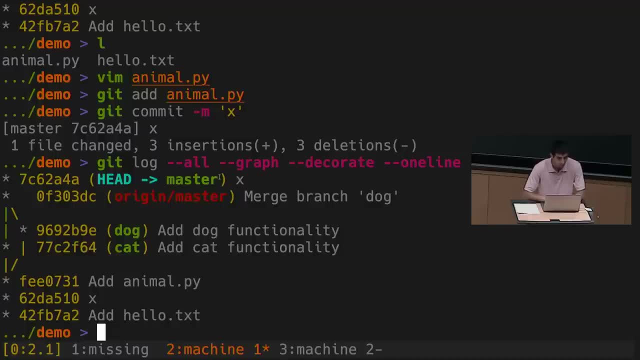 It is a way of knowing what branch on a remote machine a local branch corresponds to, so that you can type in a shortened version of git push and it'll know what all the arguments to the expanded form would have been. And there are a couple different syntaxes for doing this. 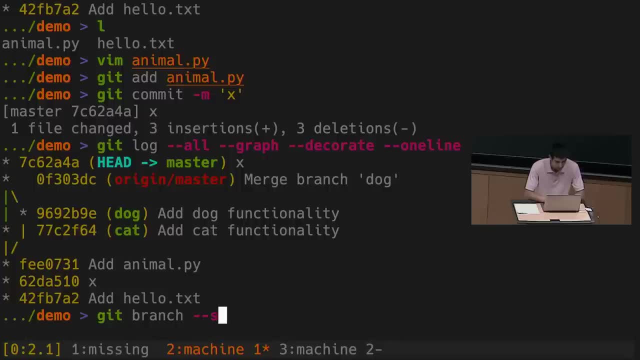 One way is to use the git branch dash- dash set upstream to command, And what this does is for the branch that's currently checked out, which is master. it will set the upstream to and I'll type in origin master And see. now it says branch master set up to track. 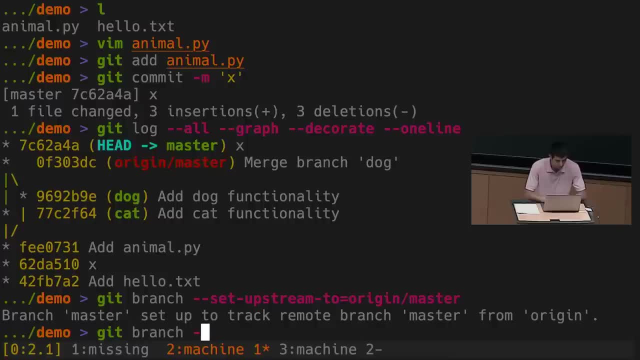 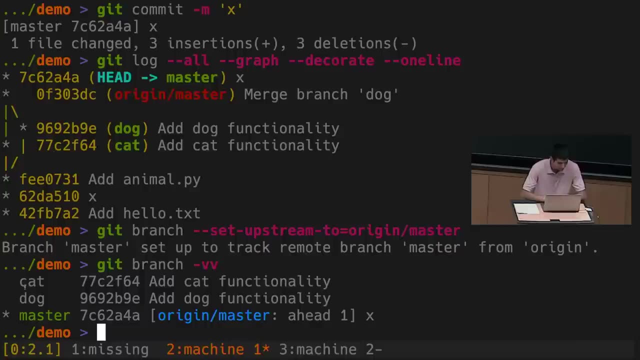 remote branch master from origin. Now, if I type in git branch dash vv, remember, this is tell me about all the branches that I know about in a very verbose way. That's what the dash vv means. I have three branches: on my local machine, on machine one. 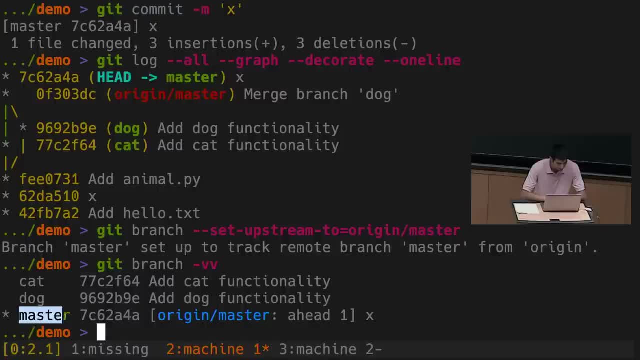 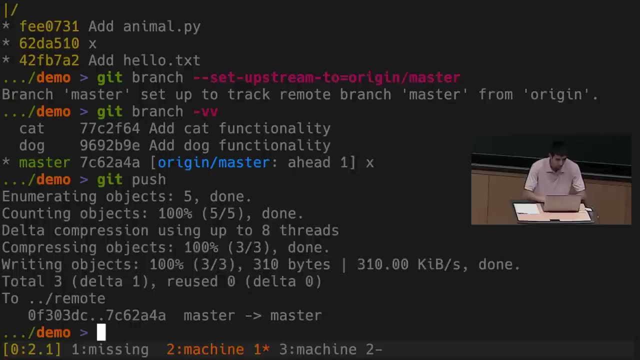 I have cat, dog and master, And master on my local machine corresponds to origin master, So now I can type in just git push without all the extra arguments. I could have done this as git push, origin master, colon master, but it wasn't necessary. 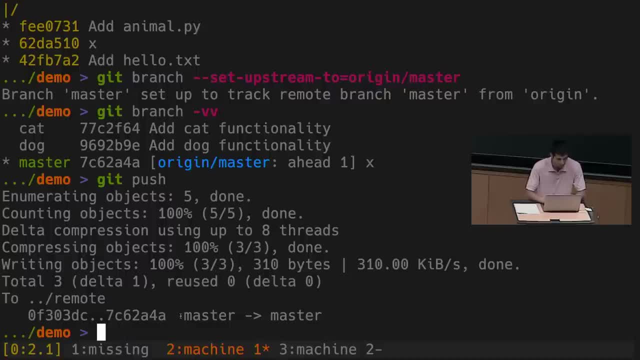 It'll know that I want to push to origin master and it'll know that I want to push to origin master And it will make that change. So now these changes are present on the remote, We can go over to machine two. pretend we're the other guy interacting. 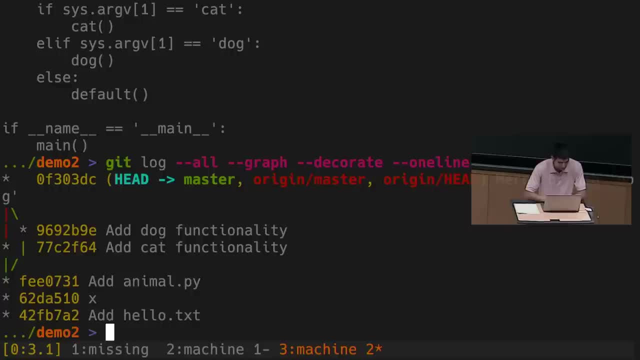 with this repository And if I do my git log command, I still don't see the changes. So what's going on here? Well, it's necessary in order to run a separate command, or it's necessary to run a separate command in order to have these changes present here. 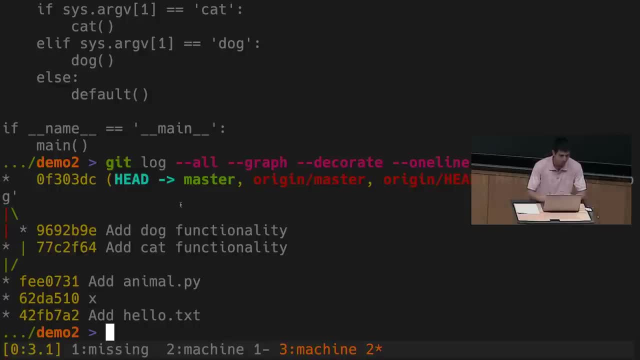 By default, all the git commands don't talk to the internet. It all works locally, which means it works very fast. But then there are special commands for saying that you want to retrieve changes that have been made somewhere else And the command that's used for doing that. 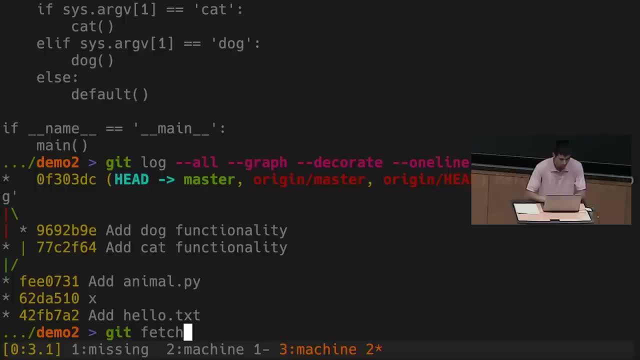 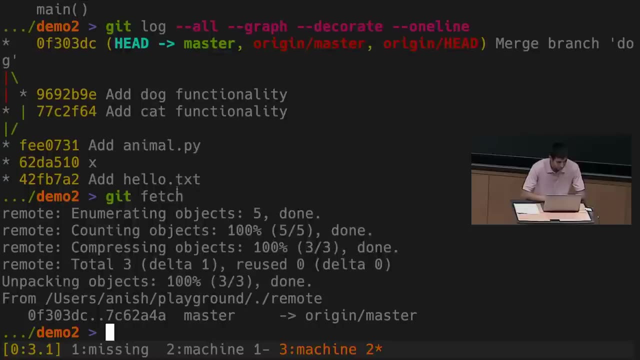 is a command called git fetch. Git fetch takes as an argument the name of the remote, But if there's only one it'll just use that, So you can type in git fetch And then it's talked to this remote repository. 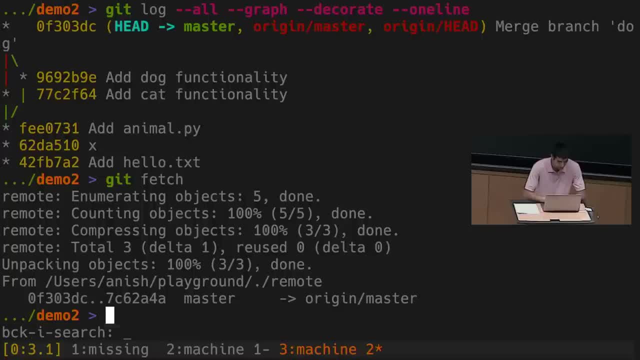 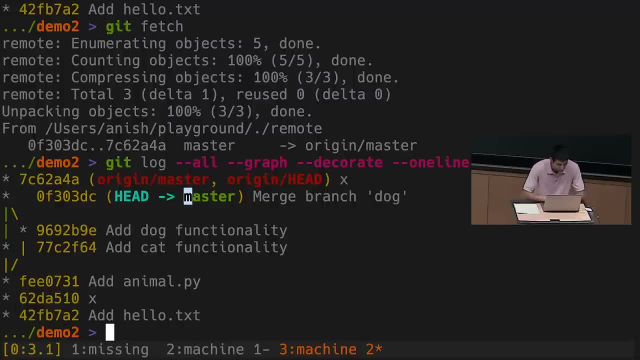 And it says that there is some update on the remote and we can visualize it by running git log. And now we see here, We see here another situation that we hadn't seen before. We have master On our local machine. the master branch doesn't change. 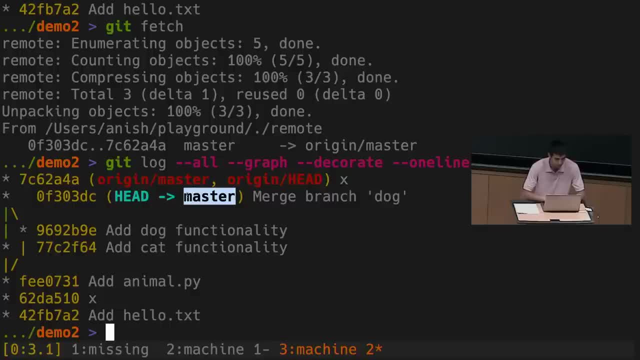 The git fetch command doesn't change any of our local history or our local references, like our branches. But now it's aware that origin master has been updated to point to this new commit And there's a separate command. We can do git merge in order to move master up to here. 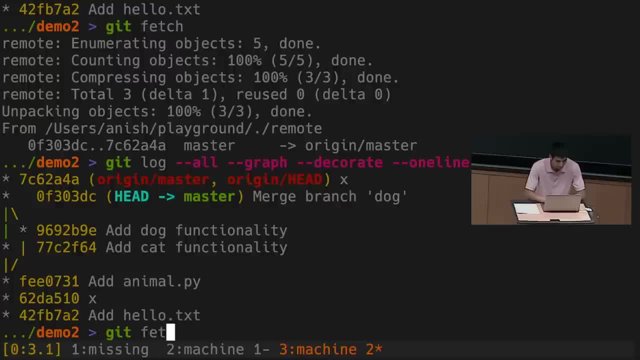 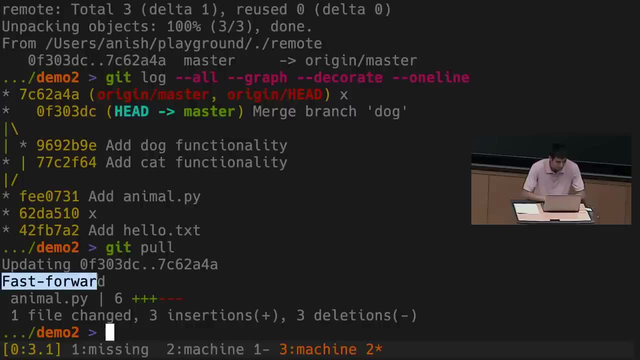 Or there's another command called git pull, which is the same as doing git fetch And then git merge. So if we just do git pull here, for example, it will say it's fast forwarding, It's merging in origin master into our master. 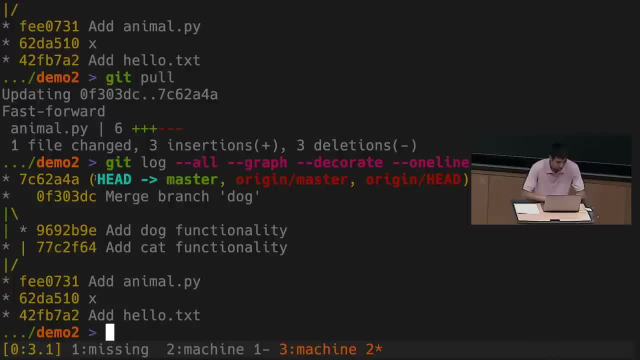 And now if we look at the git history graph we've currently checked out, master Master points to the same place as the origin master that we're aware of And all the changes between machine two and machine one are in sync. So those are the basic commands for interacting with git. 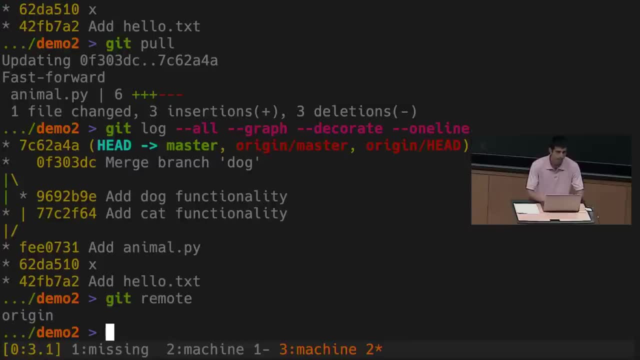 remotes. So there's the git remote command for listing remotes and adding and removing them And things like that, And then there's the git push command for sending changes from your local copy of the repository to the remote, And then there's the git fetch command. 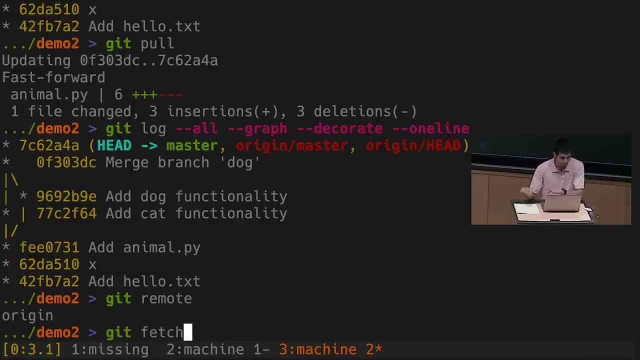 which is for retrieving changes to a repository that are present on a remote and getting the changes on your local machine. And once you retrieve those changes, you can use git merge to update your local branch to point to the same place where the remote branch does. 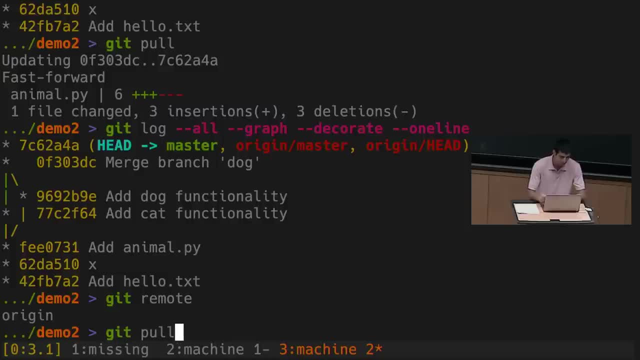 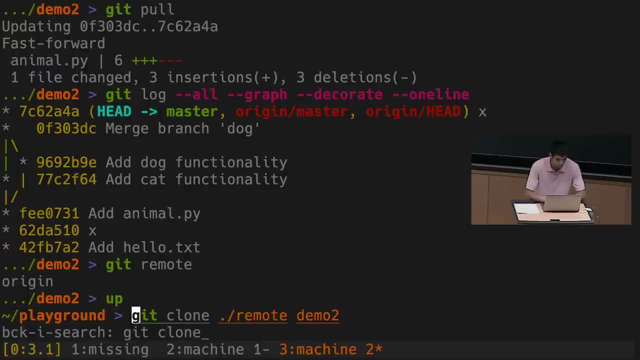 Or you can use the git pull command, which does basically the same thing as git fetch, And then, of course, separate from all these commands, is the git clone command that we talked about a little while ago, which is for taking a copy of a remote repository. 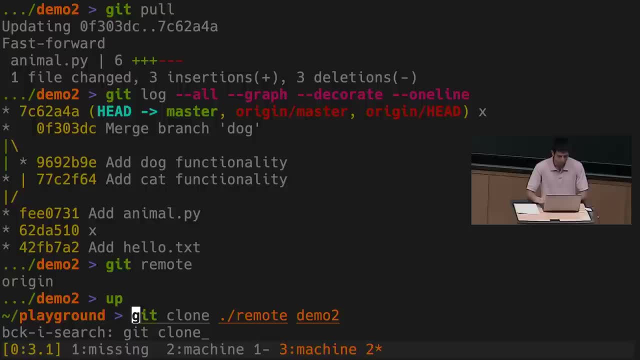 and initializing a local repository from that copy. So that's a quick overview of the different commands used to interact with git remotes. And now these are kind of complicated And it takes a while to master all the different variations of this and understand how they're actually. 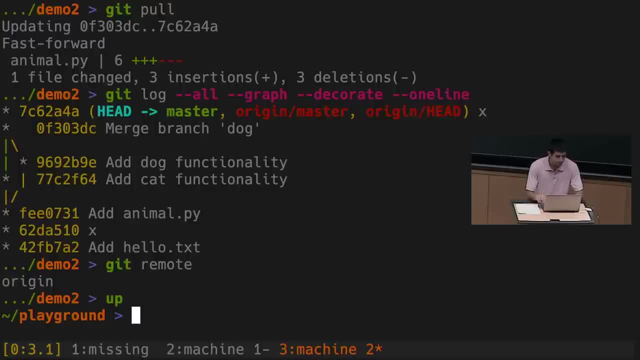 used in practice. But hopefully this acts as a quick introduction And you can see how the different commands relate to the underlying data model. All of these commands: all they do is fetch new objects from other places or send objects from the local machine to other places. 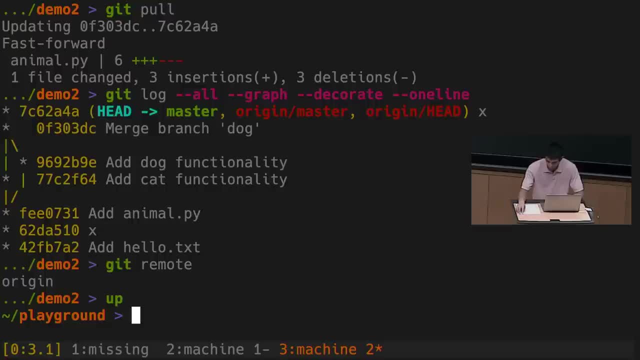 And these commands mutate references. So relating the interface of git and some of these kind of badly designed commands to the underlying data model can help it make a lot more sense. The final topic we're going to cover today is just a kind of overview of other things that git can do. 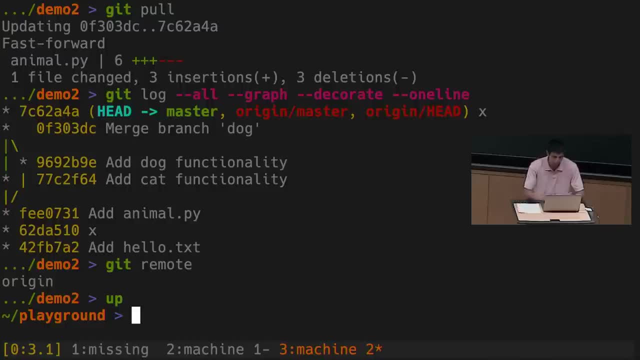 that we're not going to go into detail in teaching you how to do, but we just want to tell you that these functionalities exist. in case you need to do these things yourself, You can look up the documentation and find out exactly how to do it. 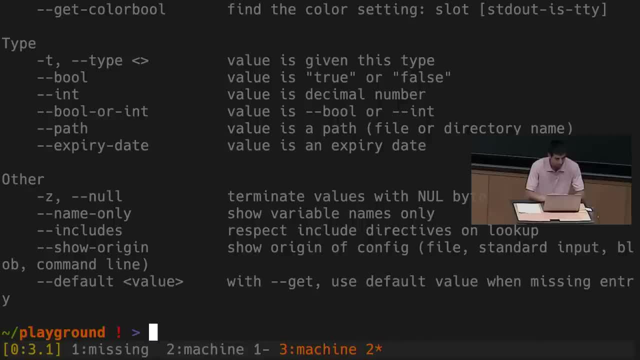 One thing is the git config command. Like a lot of tools we've looked at, like the shell and tmux and things like that, git is highly configurable And it's configured using a plain text file which can be edited either through the command line interface, so git. 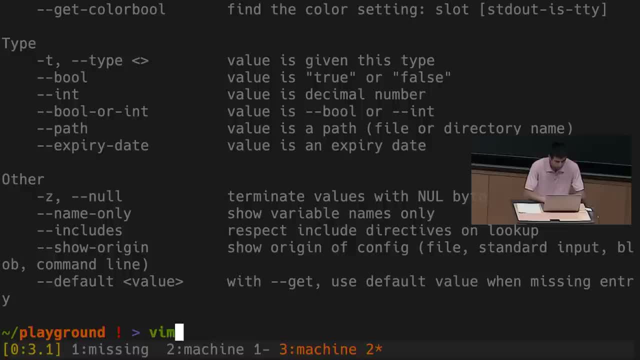 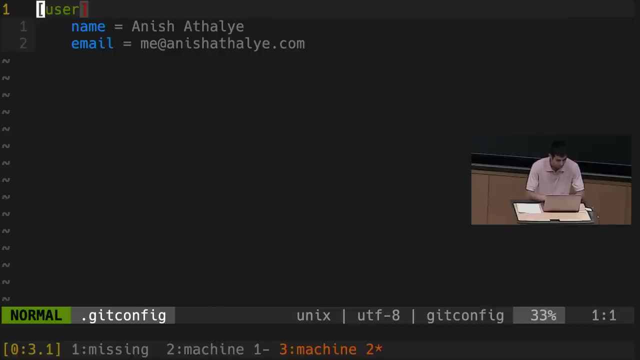 config And flags that will modify this text file, Or you can edit the gitconfig file in the home folder with plain text configuration, And so for this lecture I've actually cut out most of my git config and only left in my username. 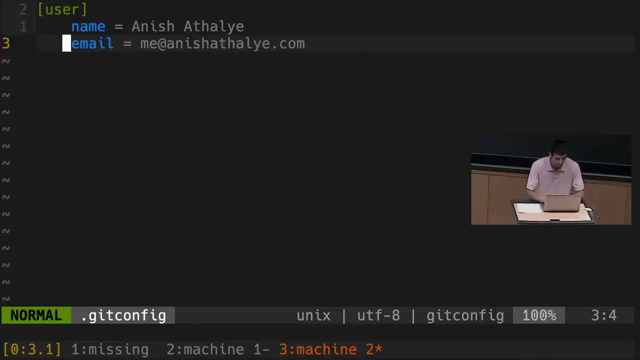 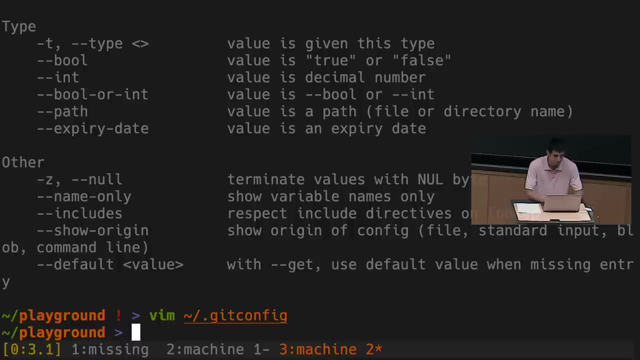 and email for what will go into git commits. But there's a lot of stuff you can put in here which will make git behave nicer or behave the way you want it to, And you can look online for different ways. people have configured their git configs. 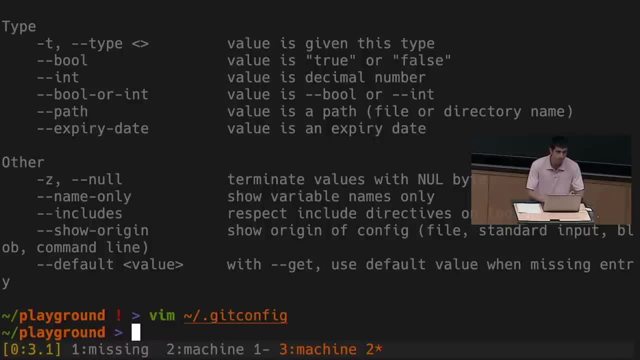 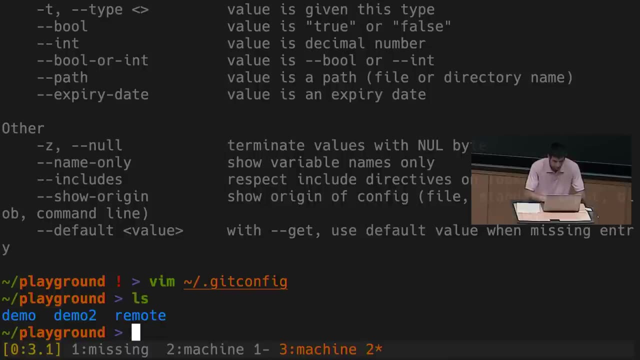 Oftentimes people have config And you can look at their documentation in their git configs, which can be found on GitHub. There's a couple other random commands that could be useful. One is for when you want to clone a repository with git clone. 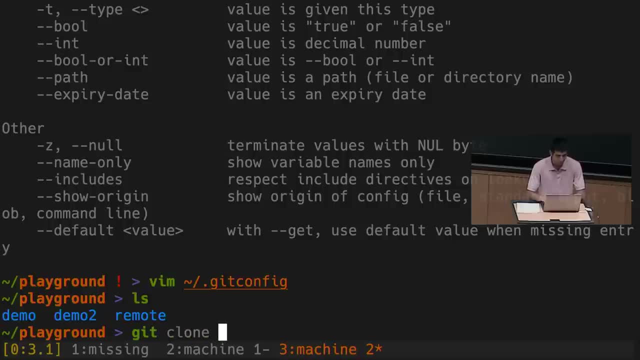 that's really gigantic. Git clone by default copies the entire version history from the remote it's downloading the repository from, But there's an argument you can pass it which is dash, dash shallow, which will avoid doing that. So if there's some copy of some code on GitHub, 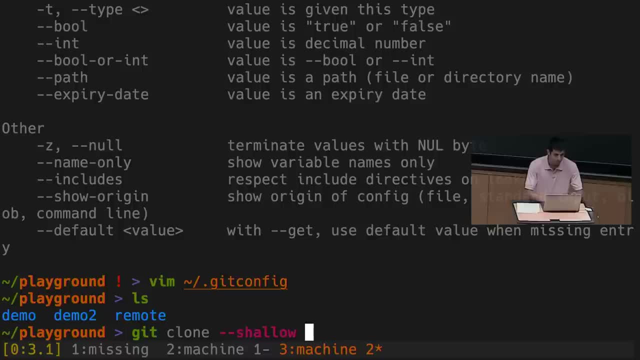 say that you want to get a copy of on your computer or you want to get a copy of on your local machine, but that repository is really gigantic and has a billion commits. if you use git, clone, dash, dash, shallow, this will be much faster. 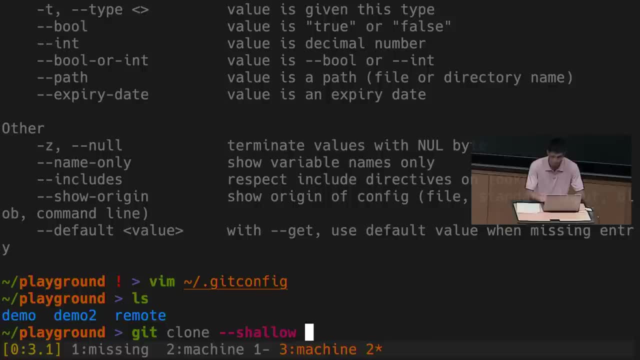 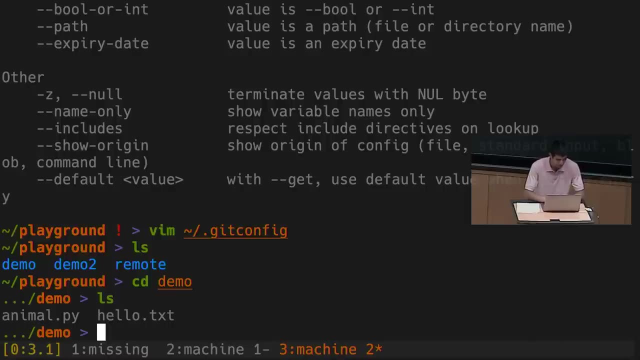 But then of course you won't have the version history on your local machine, You'll just have the latest snapshot. Another command that we find really useful when doing development on real software projects is an interactive version of the git add command. So to demonstrate this, I'm going. 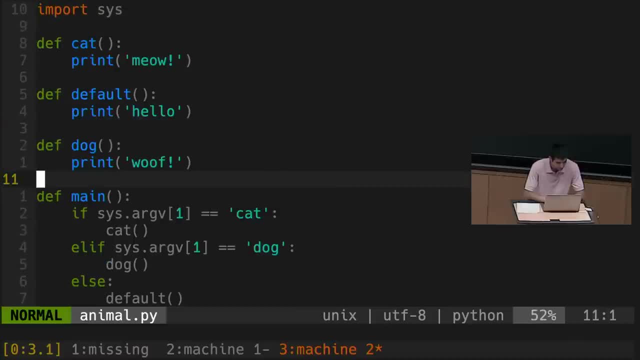 to go ahead and make a couple different changes to my animalpy. One change I'll make here, I'll change some text Here and then I'll put a new print statement here. So let's pretend that this first change was some real change. 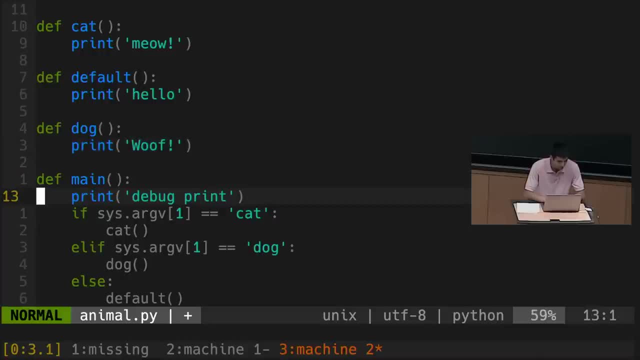 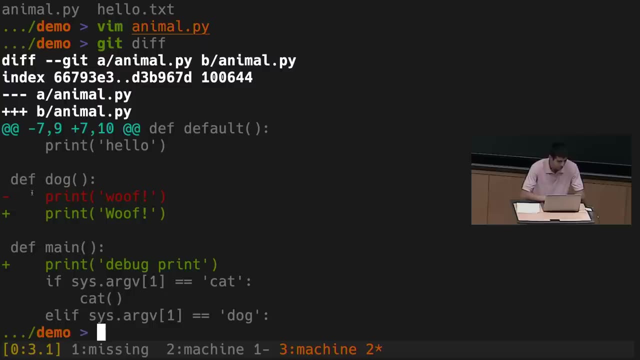 I wanted to make. Say it's a bug fix And this other change here was a printf that I added for debugging, but I don't actually want to commit in the next snapshot. If I do a git diff, it'll show me that, yes, I've. 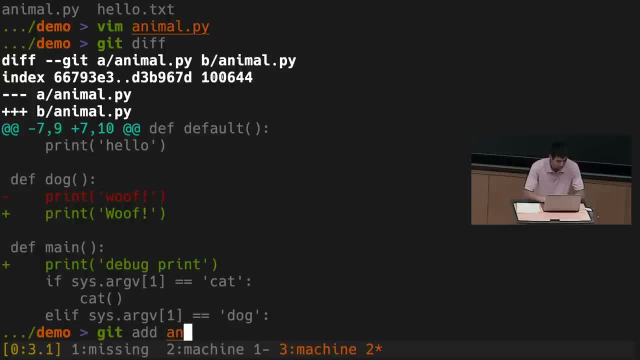 made these two changes And if I do git add animalpy it will stage both of those changes for a commit, And that's not what I want. I could go manually remove this debug print and then do this git add animalpy, But there's an easier way to do it. 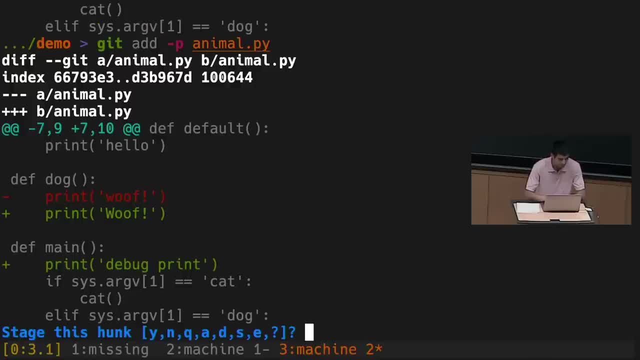 There's this git add-p command which lets me interactively stage pieces of files for a commit, And so there's some interface for working with this. So here it's saying: do I want to stage both of these changes? And no, I don't. 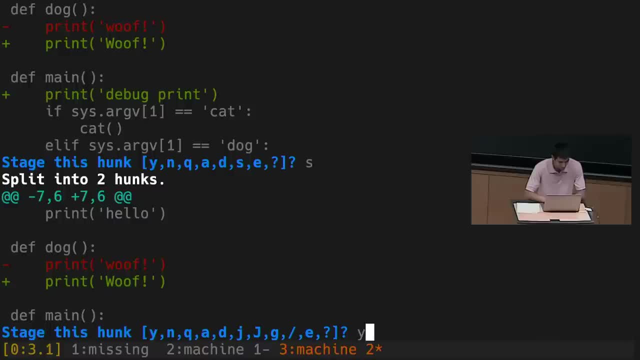 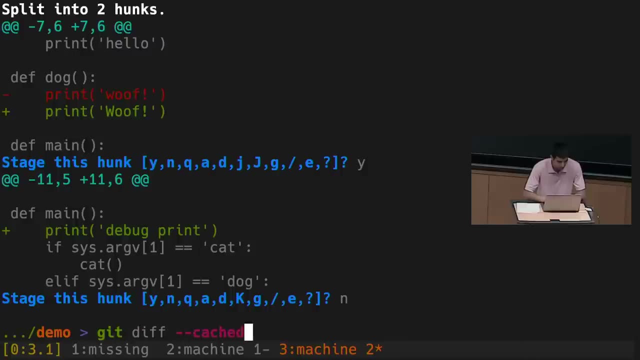 But I want to split it into two smaller changes. This one I do want to keep, so I say y for yes, And this one I don't want to keep, so I say n for no. And then, if I do git diff dash, dash cached. 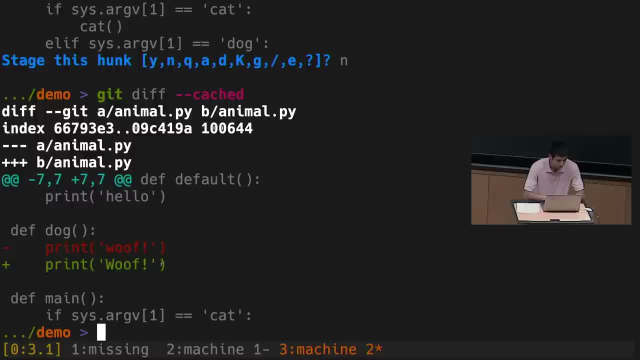 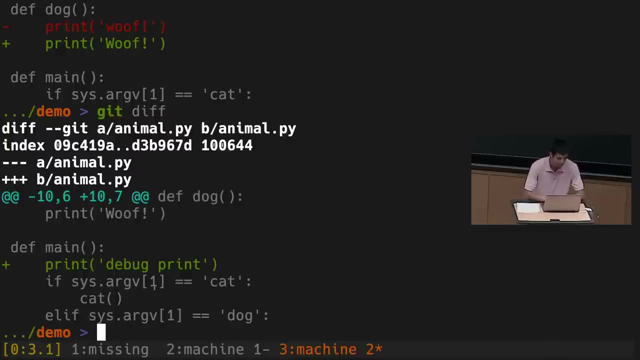 this will show me what changes are staged for a commit. So now it shows only the actual commit. This is all change I wanted to keep. If I do git diff, it'll still show me the other change that is not going to be part of the next commit, which is the change I. 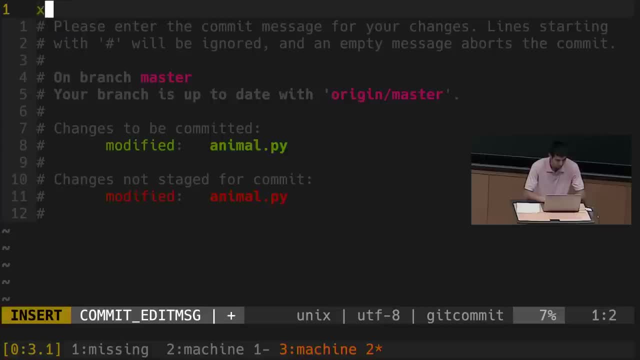 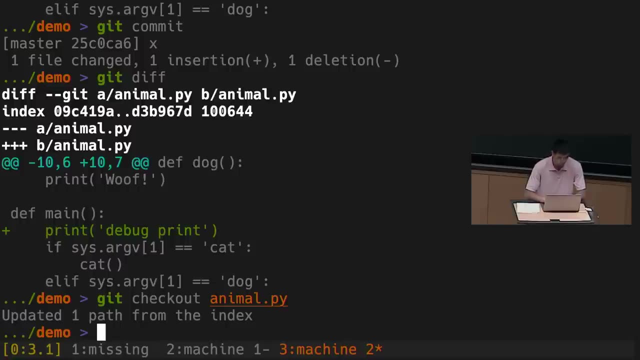 didn't want to keep. And then with this I can do git commit, specify some commit message. Now I only have this change left And then I can do git checkout animalpy to throw away this change. So git add dash p for interactive staging. 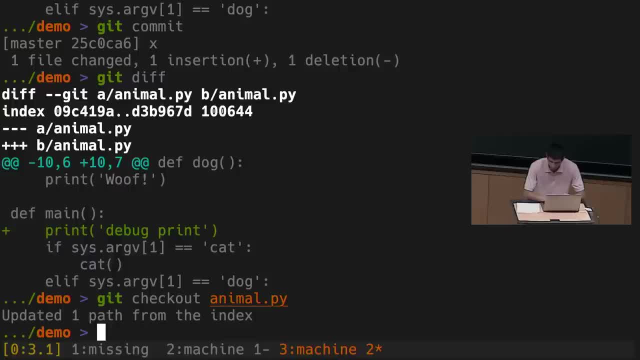 is a useful thing. A couple other commands that you can look up on your own are the git blame command. So this command sounds kind of ominous, but it can be used to figure out who edited what line of a file, And you can also find the corresponding commit. 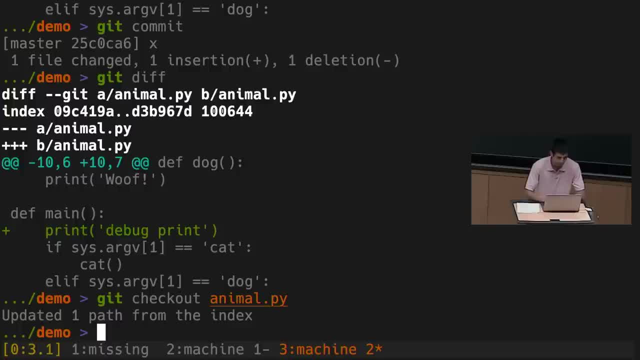 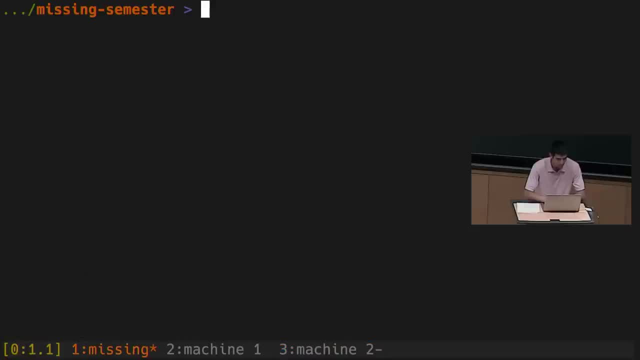 that was responsible for modifying that particular line of that file, And then you can look up commit messages associated with that and whatnot. So this is not that interesting to do in our current toy repository, But I'll go over to the repository for the class. 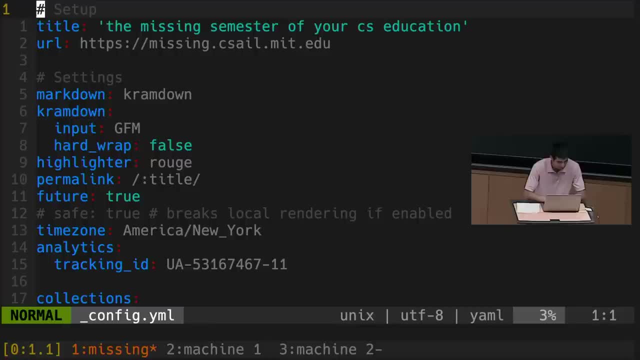 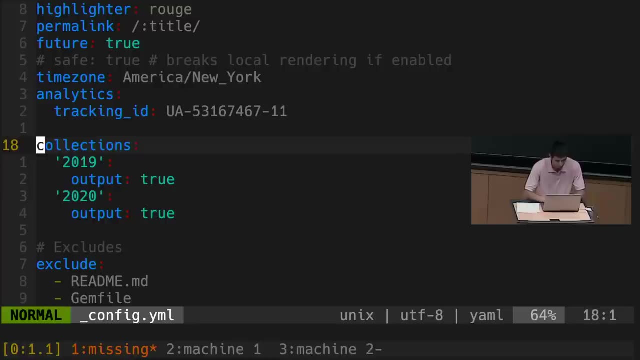 website And we can look at some particular file here. And let me go to some particular line here And I can be looking at this and be like, oh, why was this particular line added? What does it mean? And I can look at the git blame for this. 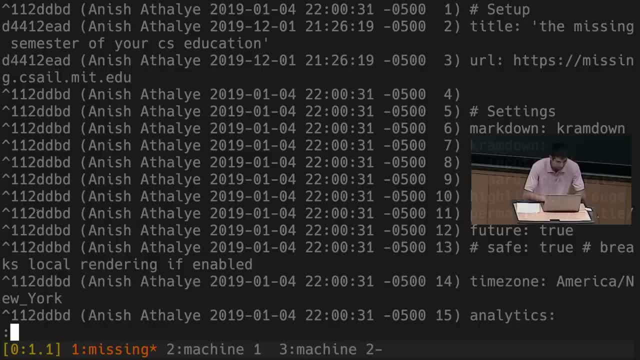 So if I do git blame configyml, it'll print out all the lines in the right column And then in the left side it'll show me what commit that change was made in and by whom, And then, looking at this, I can go down to this collections. 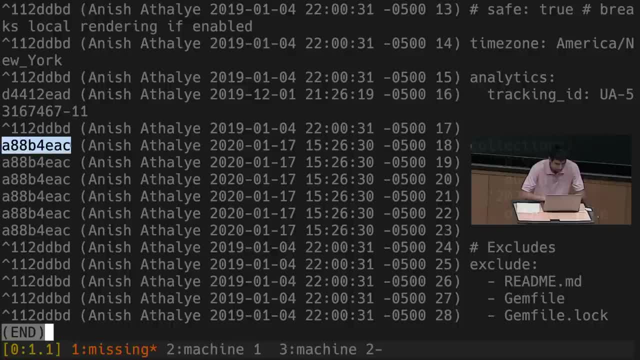 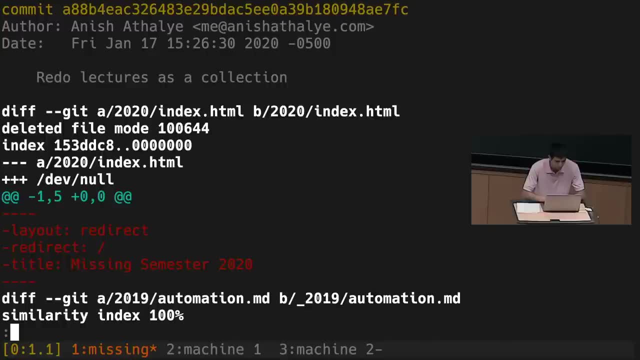 line It was made in this commit. That's the last commit that modified that line And now I can use the git show command to get information for that particular commit. Oh, and this is kind of useful: Redo lectures as a collection. 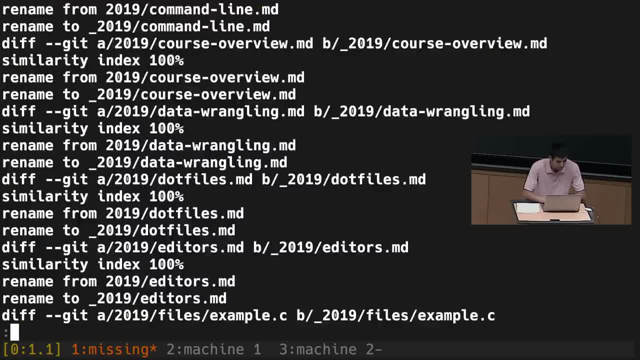 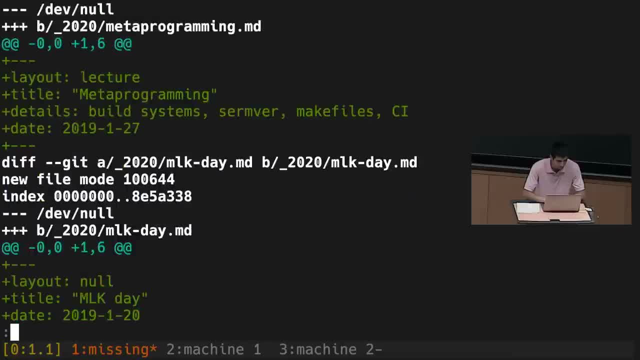 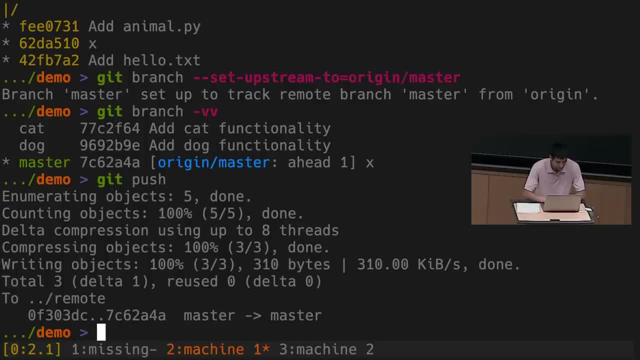 That's probably what was related to that collections line. And then, beyond just showing the commit and the commit message, it also shows me the actual changes introduced in that particular commit And I can go look through them and understand what's going on. Another kind of cool command is a command called git stash. 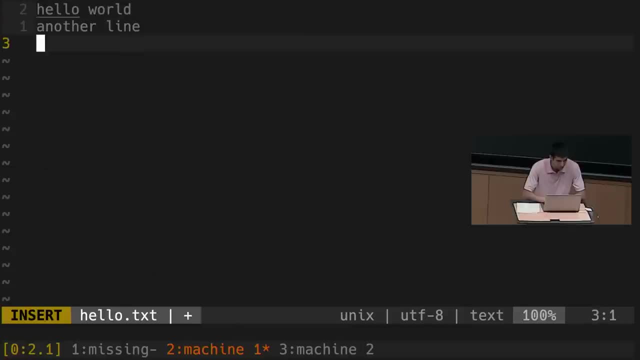 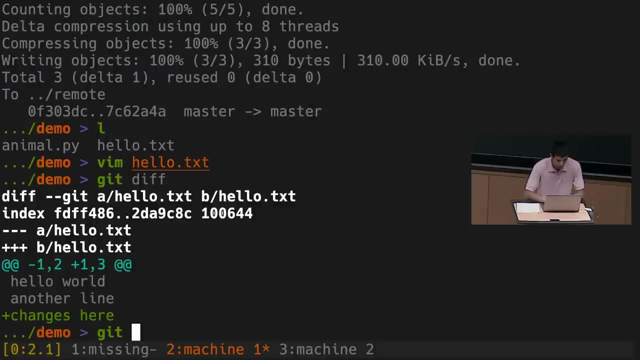 So let's go back to our demo repository and demonstrate that here. So say I have some changes here And I temporarily want to do this. I do want to put them away. If I do git stash, it will revert my working directory to the state it was in at the last commit. 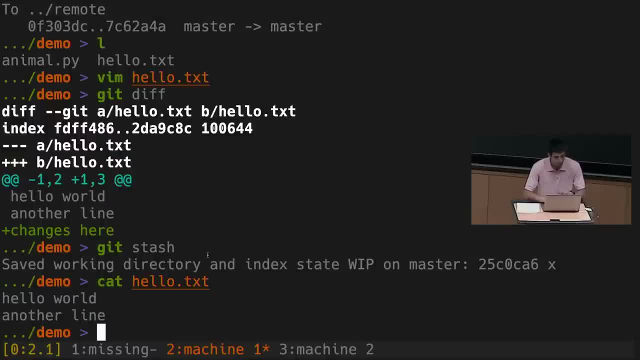 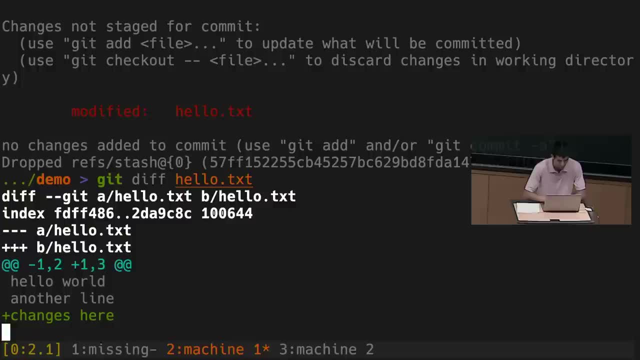 So if I do cat hellotxt, that change is gone. But it's not just deleted, It's saved somewhere And if I do git stash pop, it will undo the stash. So now if I look at hellotxt, it has the changes I made. 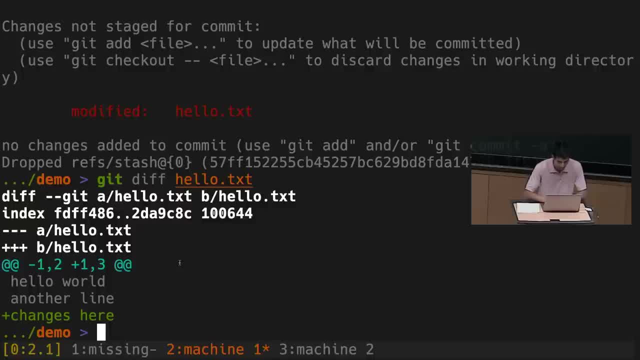 So yet another useful command. Another really neat command is something called git bisect, And this has a complicated interface that we're not going to demonstrate in detail, But basically this is a tool that can be used to solve a bunch of problems where you need to manually search history for something. 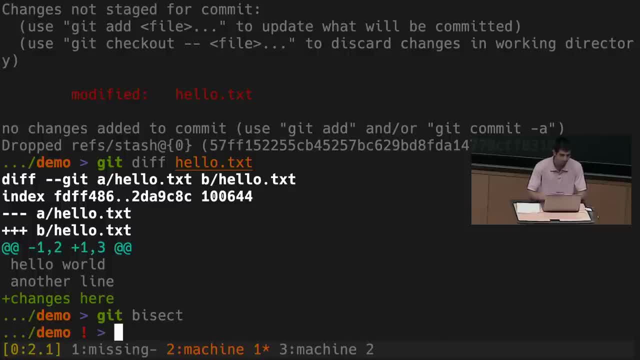 Suppose you're in a scenario where you've been working on a project for a long time, You have lots and lots of snapshots, You're 1,000 commits in And then you notice that some unit test doesn't pass anymore. But you know that this was passing one year ago. 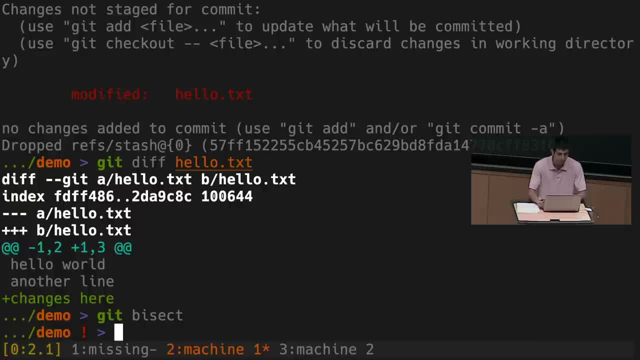 And you're trying to figure out at what point did it break, At what point was this regression in your code introduced? So one thing you could do is manually check out, go back one commit and see if the unit test is still failing. 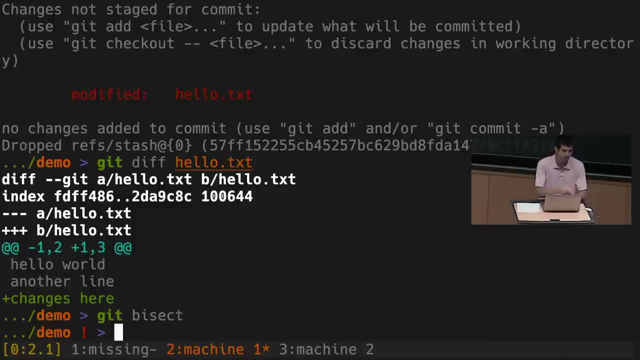 Go back one commit, see if it's still failing, And eventually you'll find the first commit where the test stopped working And it'll probably tell you what broke. But that's kind of annoying to do manually. Git bisect automates that process. 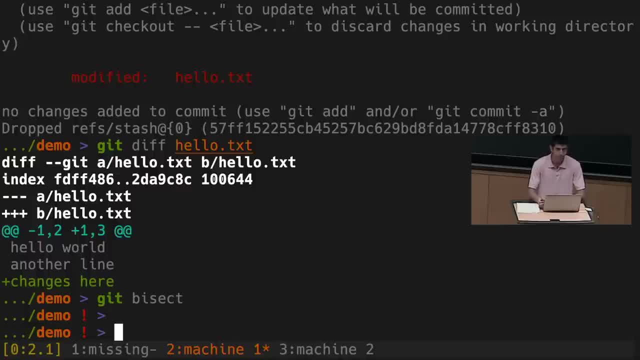 And it actually binary searches your history, So it does this in the most efficient way possible. And not only that, git bisect can take in a script that it uses to try to figure out whether a commit it's looking at is good or bad. 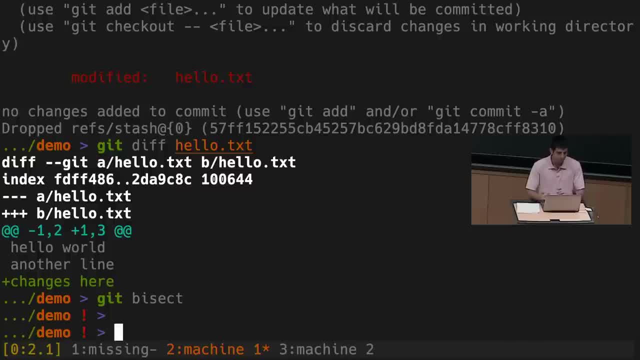 So it can be a fully automated process. You can give git bisect a unit test and say: find the first commit where this unit test stopped passing. So a really powerful tool. Another random thing that's kind of useful is something called a gitignore file. 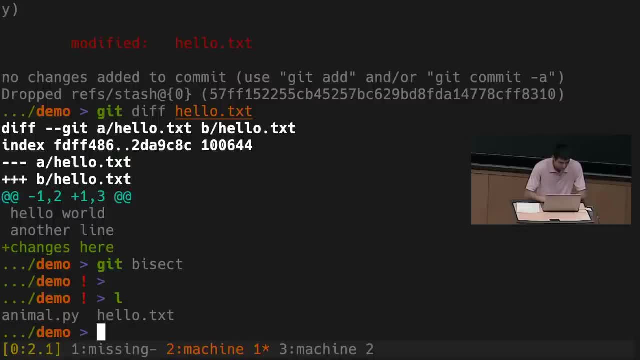 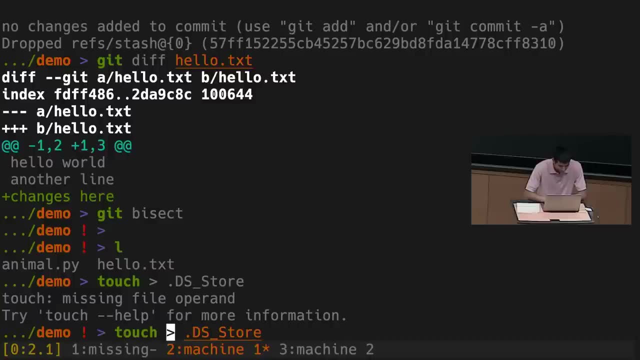 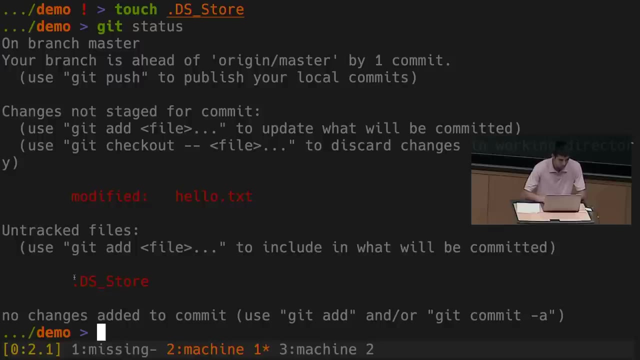 So by default, if you have random files in a directory like: let me create the ds underscore store file, Whoops, Create the ds underscore store file and then do git status. So ds store is like some nuisance file that Mac OS creates. 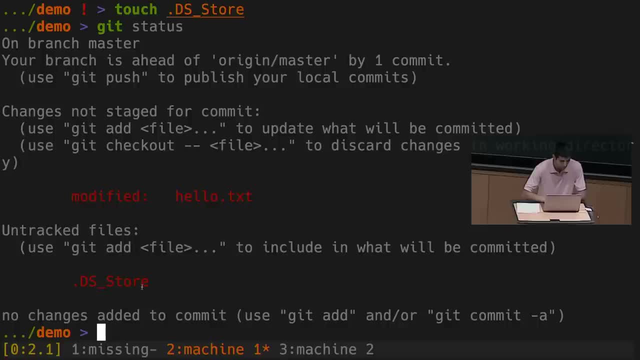 I don't know exactly what goes in here, But basically, once this file is in this directory, now whenever I do git status it says: oh, there's this new file that I've never heard of it before, but it's apparently here. 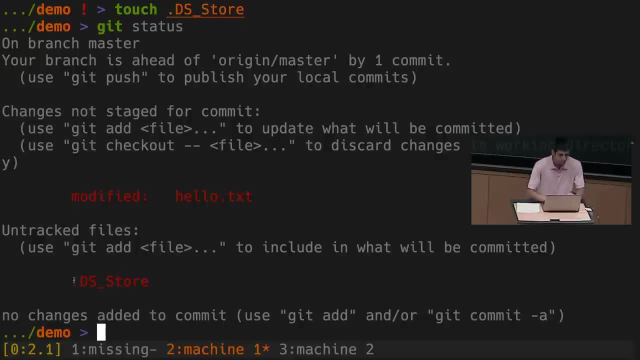 Do you want to add it, And this sort of stuff gets annoying. And there's a lot of other stuff beyond OS-specific garbage that might be in a directory, Like, for example, if you're working with C code, you might compile it and produce o files or executable files. 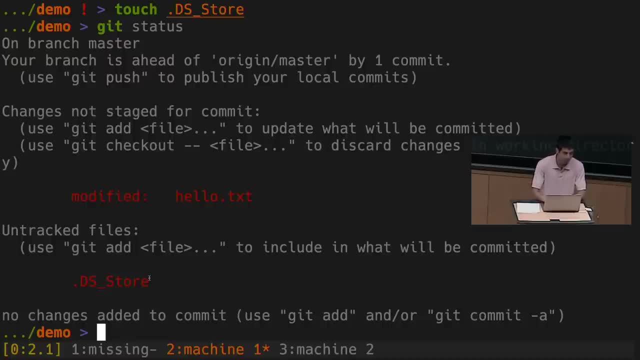 or things like that, And you probably don't want binaries to be part of your commit history. You only want the source code, And so git has a way of you being able to tell the tool that you don't care about a particular set of files and to ignore them. 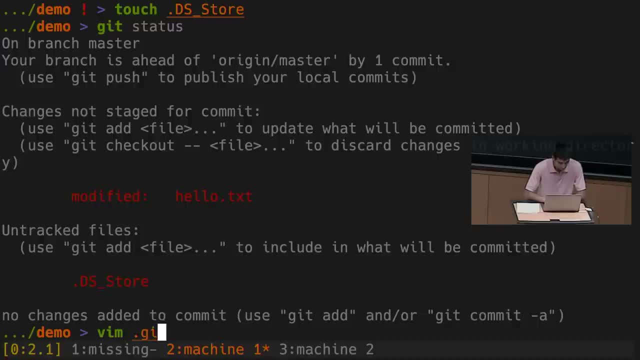 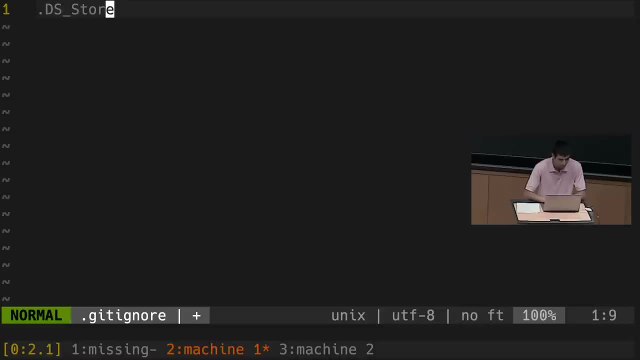 And that's something called a git ignore file. So if I go and modify the file called git ignore in the current directory, I can specify particular file names or patterns of file names, Like, say, I can specify star, o, so any file ending in o. 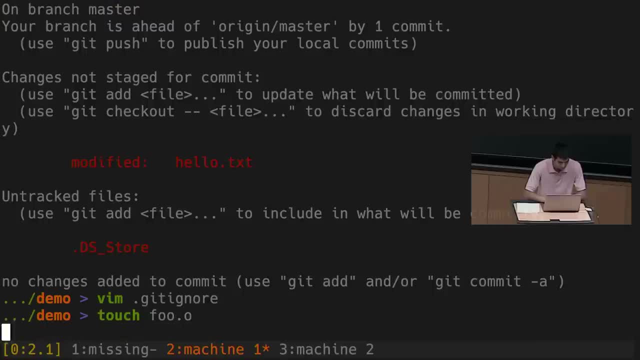 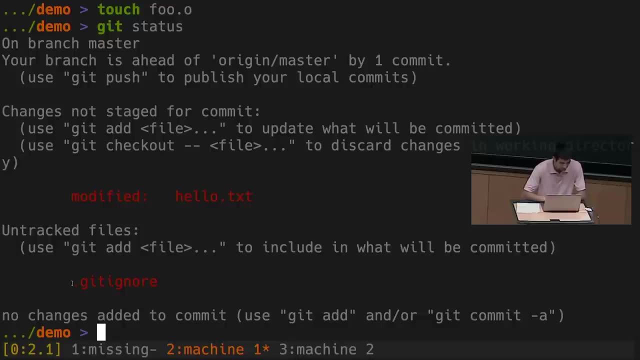 along with ds store. And now, if I touch fooo and now do a git status, I'll see that git says: OK, I have hellotxt, which I modified, sure? And then I have git ignore. So you should track your git ignore file using git. 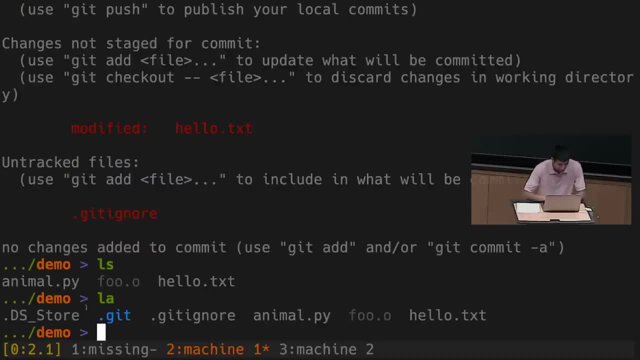 But notice that it doesn't mention my ds store file or my fooo file that's present in the current directory, because that has been git ignored. So that's a quick overview of a little bit of advanced git functionality, just to give you a flavor of what 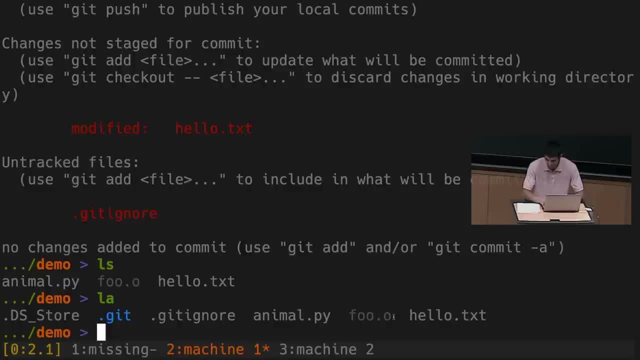 sorts of cool things this tool can do. And then, finally, we have a couple other topics that are covered in the lecture notes in more detail. I'll just quickly list them here, so you know what to look for. One is that there are many graphical clients for git. 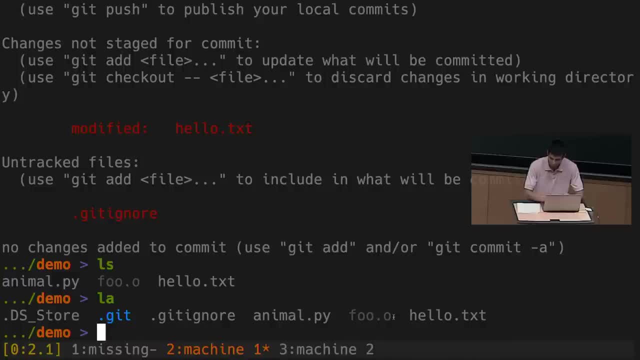 We don't personally use them. We like the git command line tool, But some of them are kind of OK and you might want to check them out just to see if you prefer using those. Another thing is shell integration, So you've noticed that in this tutorial. 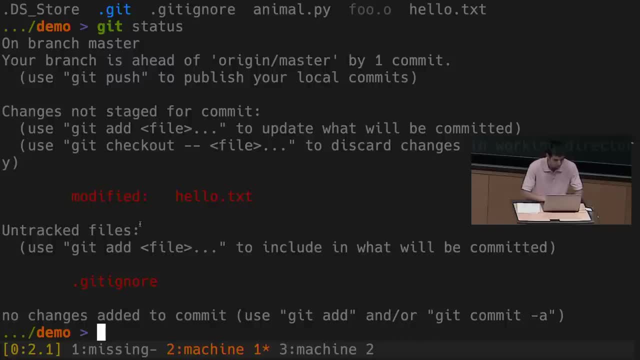 I've done git status a whole bunch to see kind of what's going on with my repository. Well, that's kind of annoying to do and a lot of people have their shell prompt set up so that just within this shell prompt itself, like on every line. 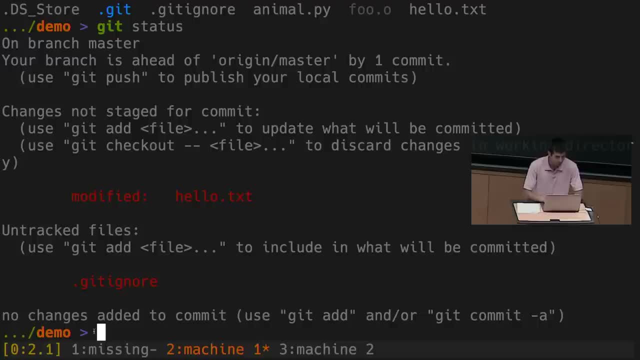 it will show me a very succinct summary of what's going on with my repository. So it might show me a summary of what branch I have currently checked out, along with maybe if I've modified files or untracked files, And so we have a link in the lecture notes. 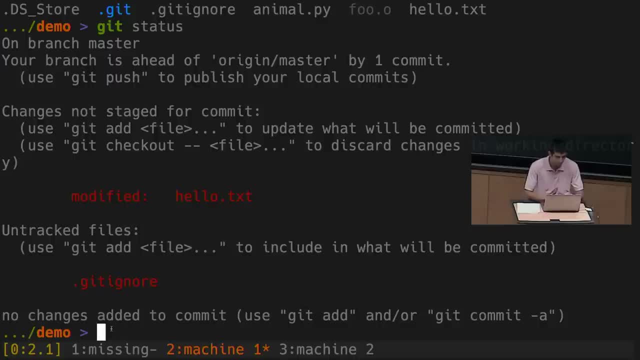 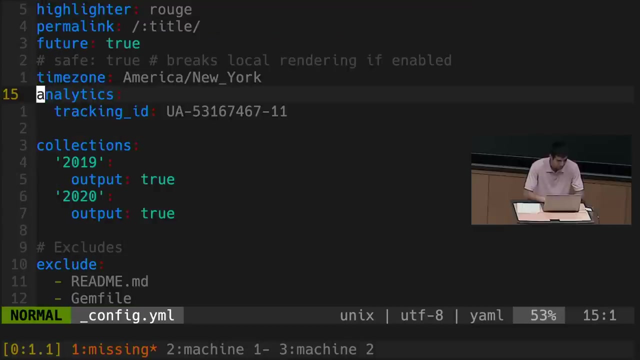 on how to get some nice shell integration for displaying git-related information in your shell prompt, Similar to that you can get integrations with your text editor. So, for example, I use vim And I have a plug-in for vim that does all sorts of interesting git-related stuff. 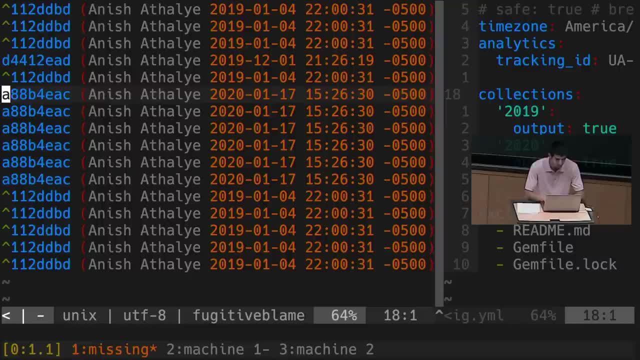 One thing I can do within this plug-in is look at git blame information. So remember we just looked at this through the command line. Instead, I can look at it with this plug-in and it lets me work with it a lot faster.